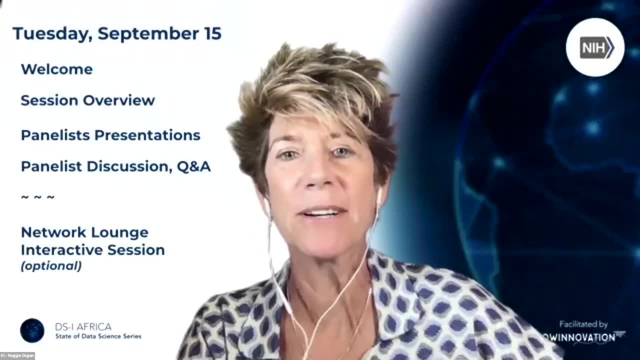 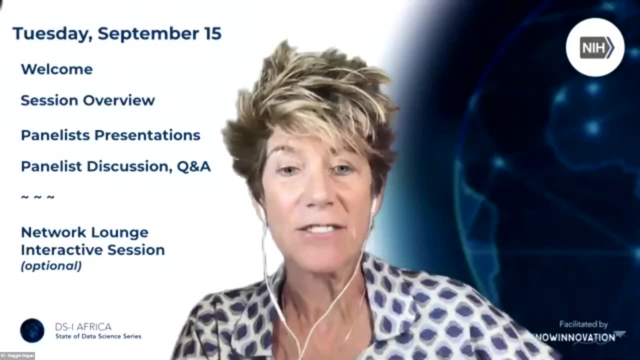 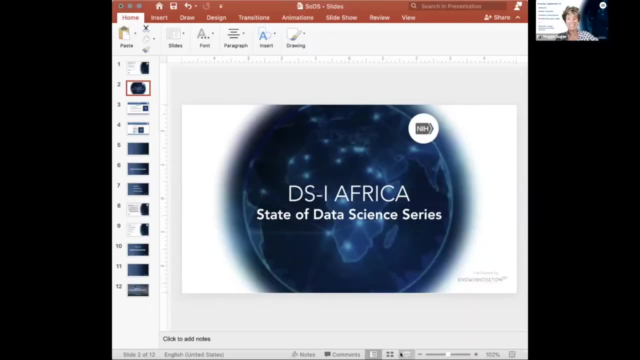 each other and continue to interact with everybody and dig deeper on the topic of biomedical imaging and data science in Africa. So, incidentally, I want to show you just a few slides to let you know that today's event is associated with the NIH Common Fund. 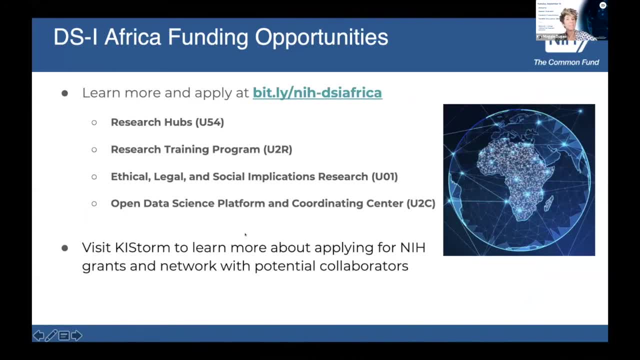 The funding opportunity. this is the NIH program on harnessing data science for health and discovery and innovation in Africa. So there are four different opportunities that are currently open: research hubs, research training, ethical, legal and social implications, open data science platform and coordinating session, If you want to learn anything more about any. 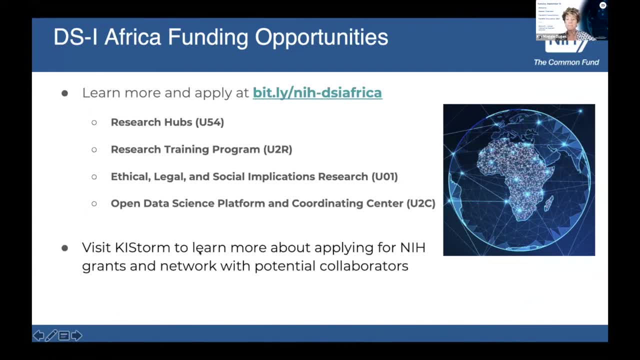 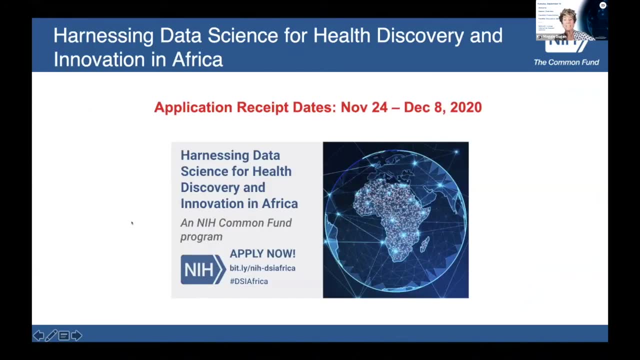 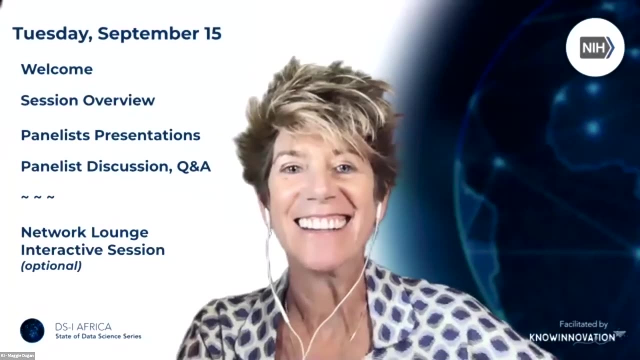 of these funding opportunities. we invite you to visit ChiStorm to learn more about how to apply, Or also to go to the NIH site. The application receipt dates are between the end of November and early December, So we encourage you to explore this further and find out more about how you can be part. 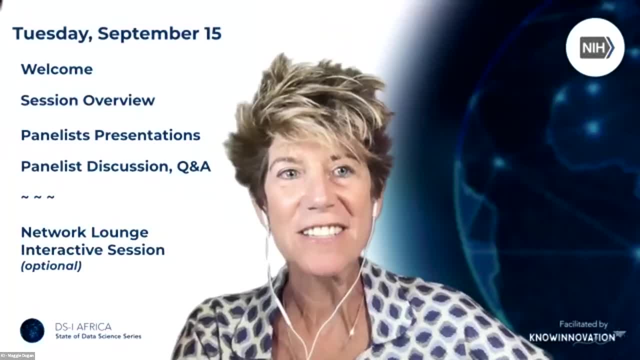 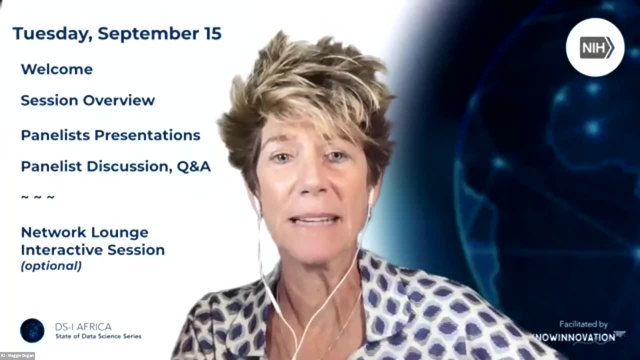 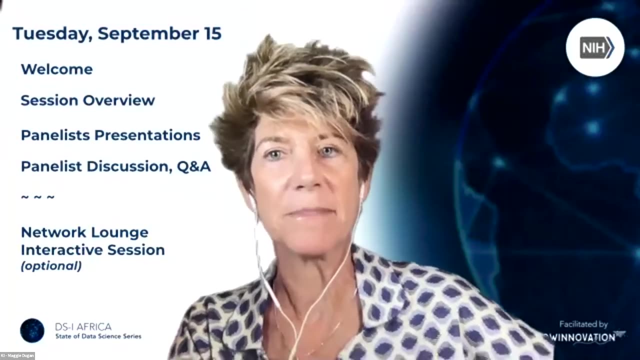 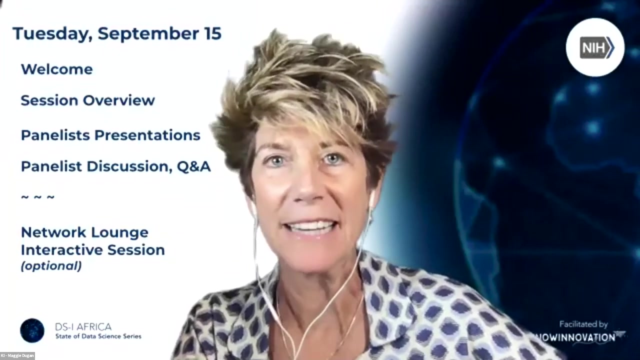 of this program. So before we start, just a few tips. We are recording this program So if you want to see anything again, you'll be able to find it here on ChiStorm or on the NIH site. If at any point during today's session you get bumped out, you get kicked out, you have problems with Zoom, you can't find where you're supposed to go, you can always go onto the ChiStorm need help page. Someone will be monitoring and we can help you find your way back to where you need to be. 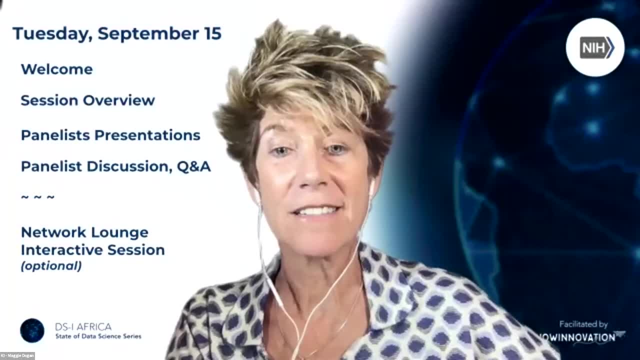 In this webinar we have the opportunity to ask questions. So you'll notice at the bottom of your screen there is a little Q&A button with some thought clouds, some speech clouds. You can click on that and add a question And as well, you can see what other people are asking. and if there's any questions, please feel free to reach out to us. 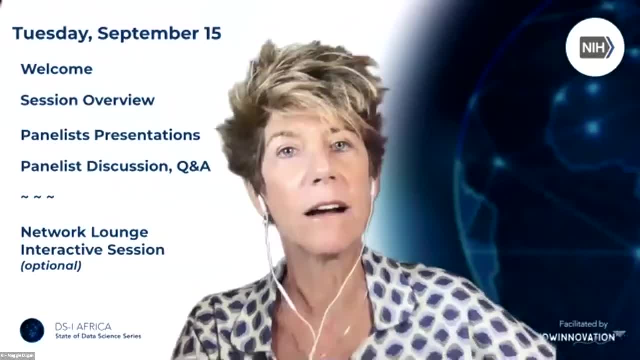 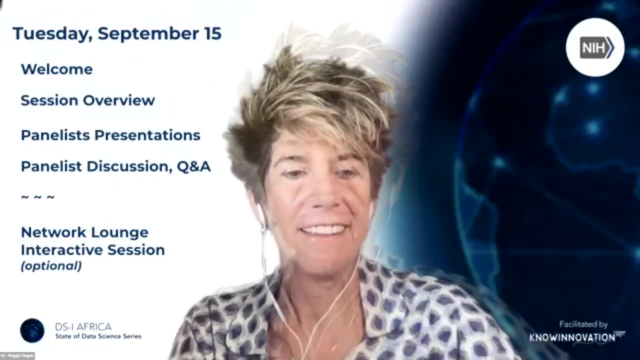 you can click on that and add a question And as well, you can see what other people are asking, And if there's a question that resonates with you particularly, you can say: yeah, I like that question too, by uploading that. 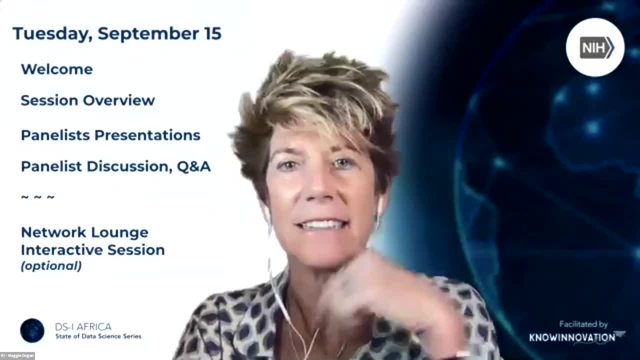 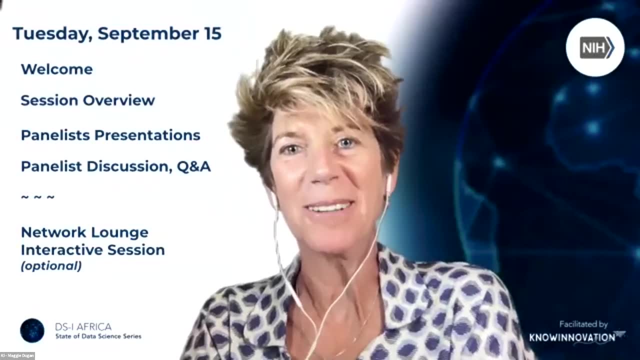 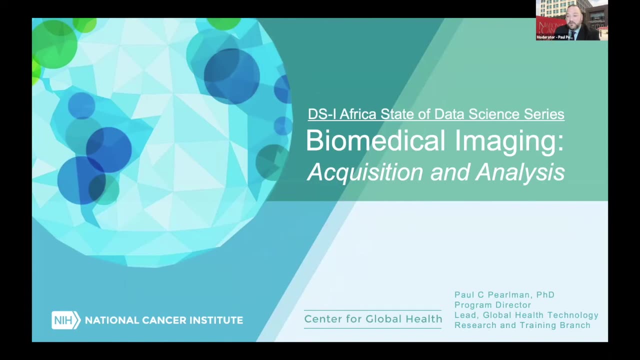 And I would just like to introduce to you our moderator, who is Dr Paul Perman from the Cancer Institute. Paul, Thank you, Maggie. I'm gonna keep this brief so we can get directly into our talks. So our session goal today is to highlight novel work. 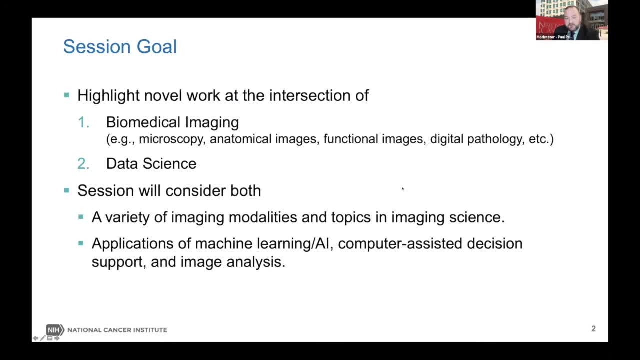 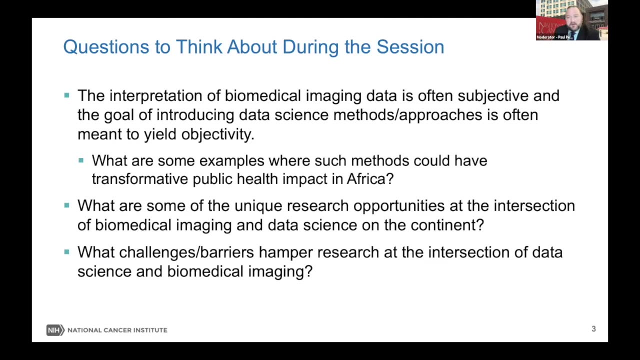 at the intersection of biomedical imaging and data science. The session will consider both a variety of imaging modalities and topics in imaging science, as well as the applications of machine learning, artificial intelligence and computer-assisted decision support and image analysis, As we're starting to think during the session. 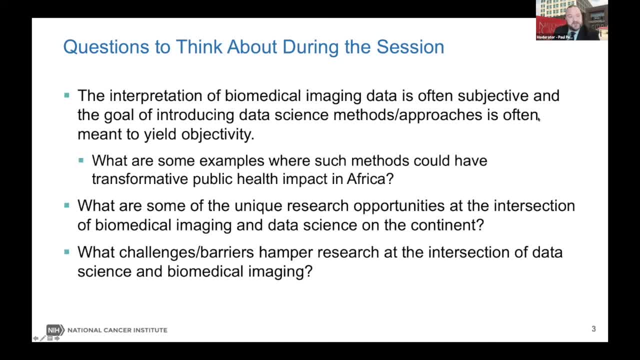 about the broader DSI program and maybe potential applications to that program. I want you to think about the interpretation of biomedical imaging data often being subjective and that the goal of introducing data science methods and approaches is often meant to yield objectivity. So, with that in mind, what are some of the examples? 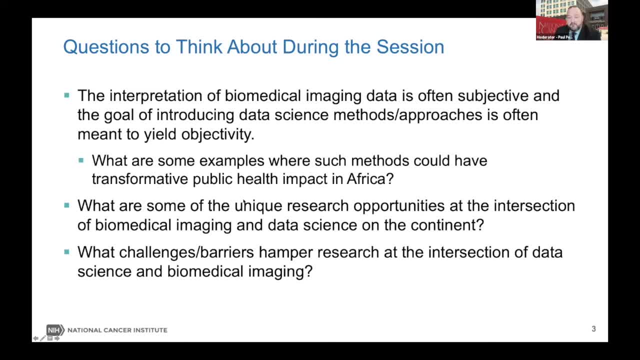 where such methods could have a transformative public health impact in Africa? Furthermore, what are some of the unique research opportunities at the intersection of biomedical imaging and data science on the continent? Finally, what are the challenges and barriers that hamper research intersection of data science and biomedical imaging? um. so today's panel consists of these. 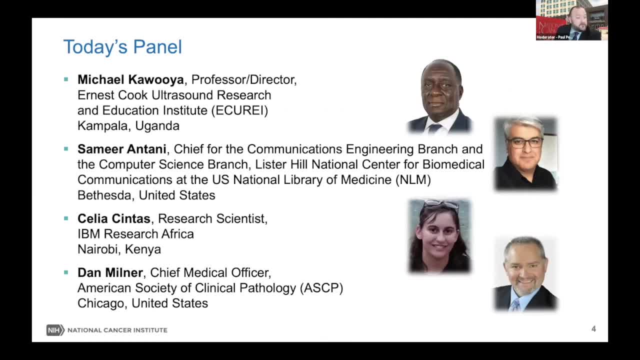 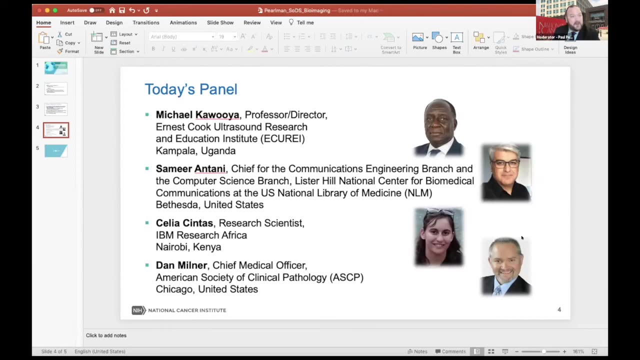 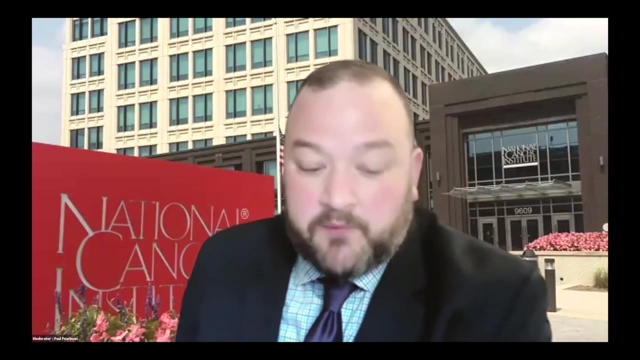 four speakers, uh doctors michael kaluuya, uh dr samir antani, dr celia santos and dr dan milner, who all introduced prior to each talk. so, um, as uh dr kaluuya is uh getting his slides up, i will go ahead and stop sharing and introduce him. um so, professor michael kaluuya is a general radiologist. 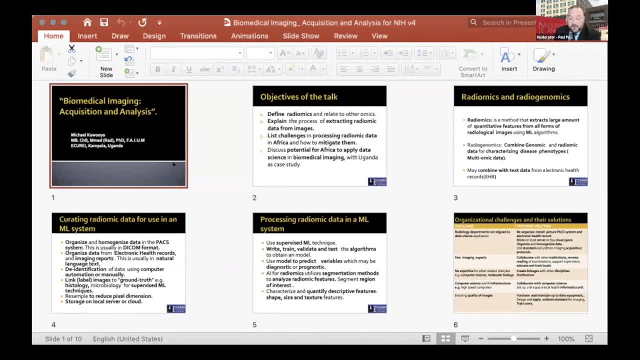 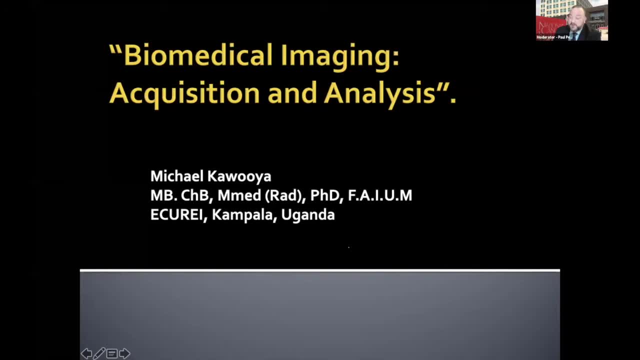 with a special interest in diagnostic and interventional ultrasound. he's engaged in clinical work, research and teaching at the ernst cook ultrasound research and education institute in kamala. with that i'll turn it over to you, professor. good afternoon to you from uganda. we are going to look at the medical imaging acquisition analysis. 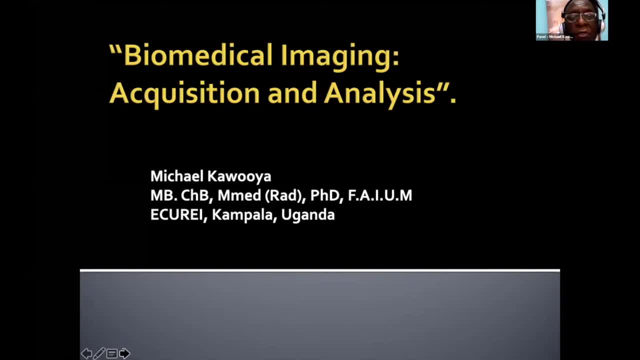 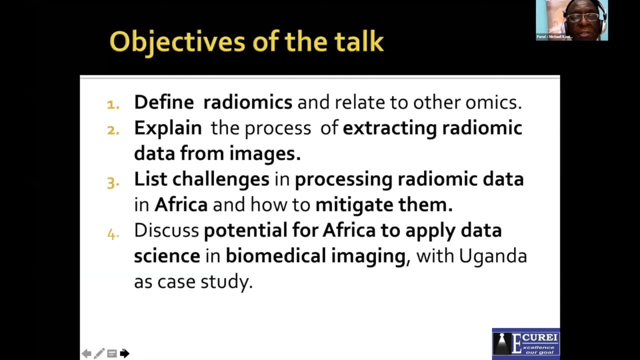 the talk i'm going to handle is going to be basically on imaging and we are going to look at biomedical imaging acquisition and analysis. the objectives to define radiomics and relate to other omics explain the process of extracting radiomic data images, list challenges in processing radiomic data in Africa and how to mitigate these challenges. 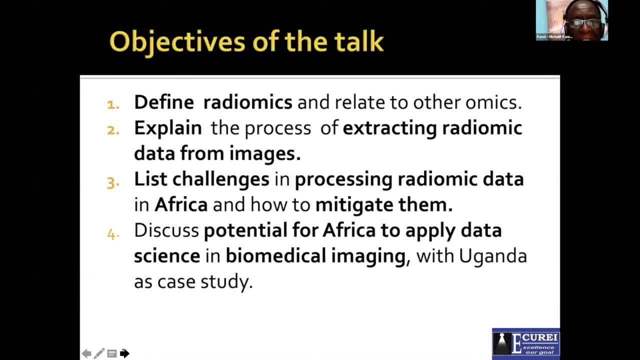 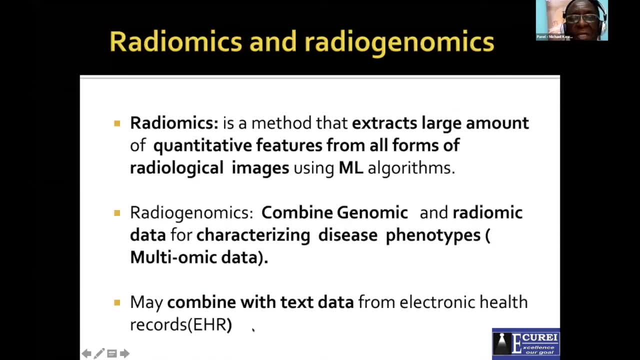 discuss potential for Africa to apply data science in biomedical imaging, with Uganda as a case study. Radiomics is a method that extracts large amounts of quantitative features from all forms of radiological imaging using machine learning algorithms, And there's also what we call radiogenomics, which combines genomic and radiomic data to 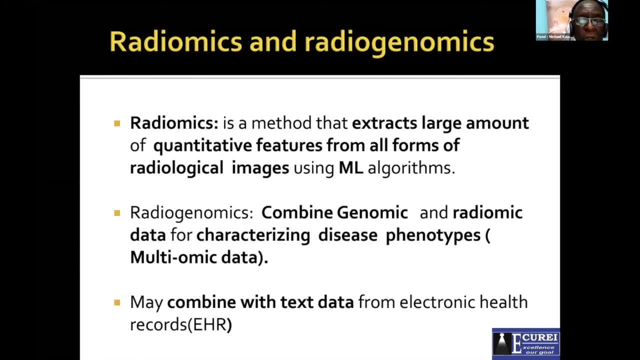 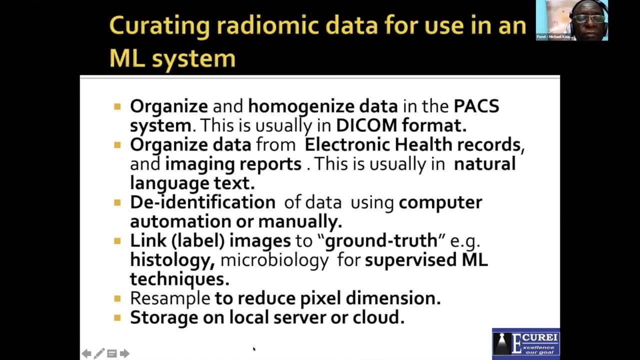 characterize disease phenotypes, and we call this multi-omic data. You may also combine this with text. data from electronic health records, if that is necessary. Curating radiomic data for use in an ML system. Data from imaging studies: These studies have to be organized and homogenized in the PACS system, and this is usually in. 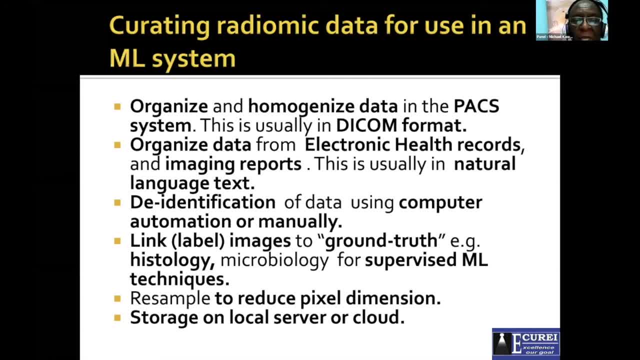 a DICOM format. We organize the data from electronic health records and imaging reports, and this is usually in natural language text. The data has to be de-identified and then also has to be linked to the ground truth, which may be histology or microbiology. 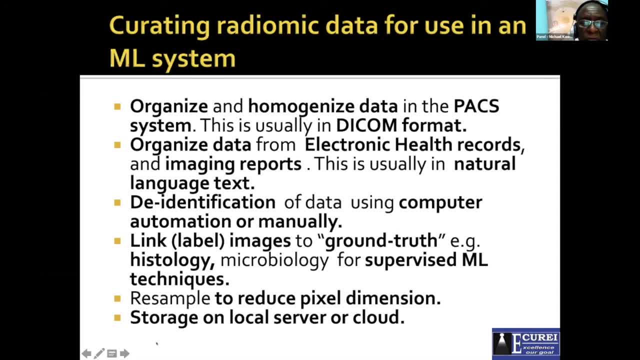 Because it is data which is in the system, It has to be linked to the ground truth, which may be histology or microbiology. Because it is data which is in the system, It has to be linked to the ground truth, which may be histology or microbiology. 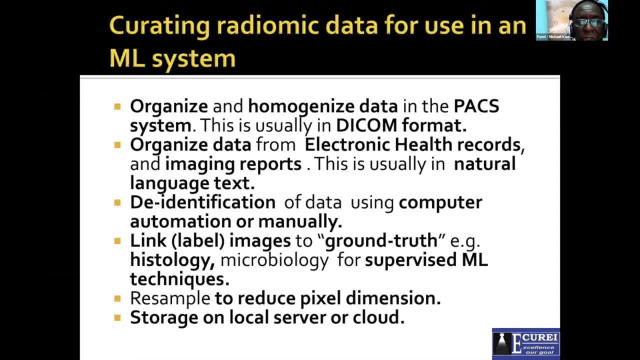 That data can be buzzed into jewelry. So the program has to be in the system of complex memory, so that夠 is very heavy. We have to reduce the pixel dimensions so that then we can be able to process it with the computer we have. 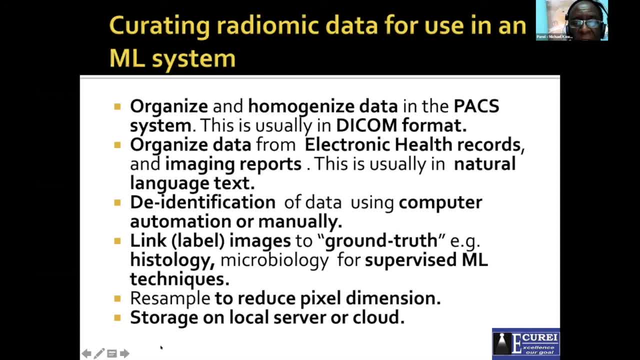 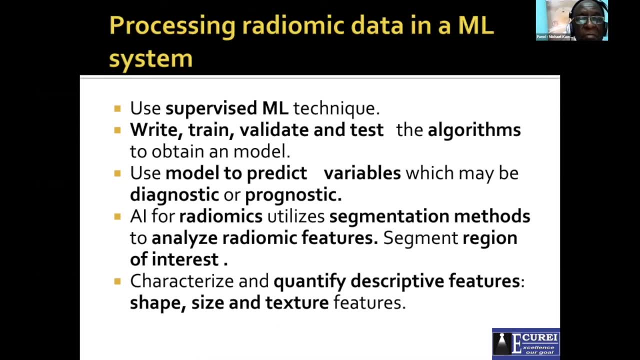 Otherwise it requires a very high-speed computer. then the data can be stored on the local server or on a cloud. Now how do we process data in a machine learning system? We usually use supervised machine learning technique. We're able to make any machine learning DA online in a workforce system. 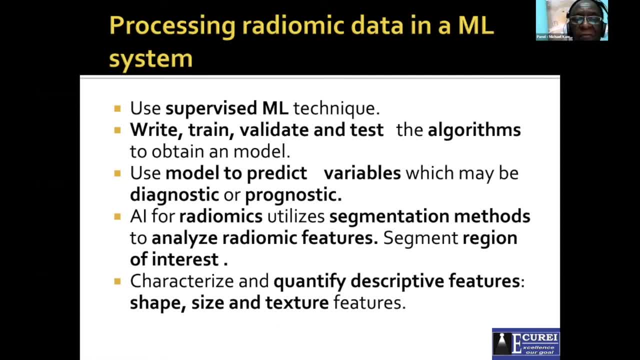 We want to have some potential timescales to confirm. We'll write, train, validate and test the algorithms to obtain a model. Then we use that model to predict variables which may be diagnostic or prognostic, And artificial intelligence for radiomic data utilizes segmentation methods to analyze the 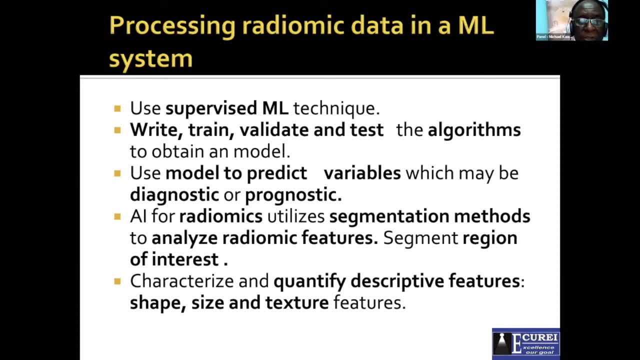 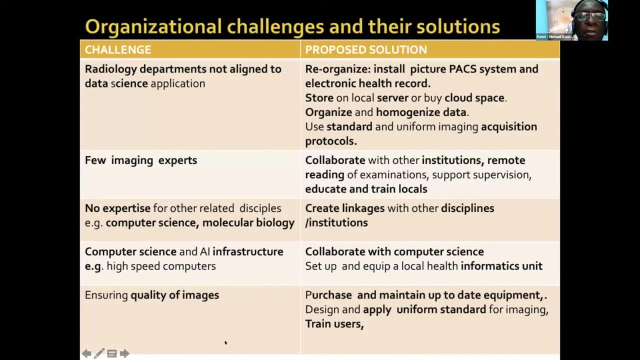 radiomic features and we segment the region of interest And then after that we characterize and quantify descriptive features, which are like shape, size and texture features. Now there are challenges with dealing with radiomic data data from radiology in Africa. 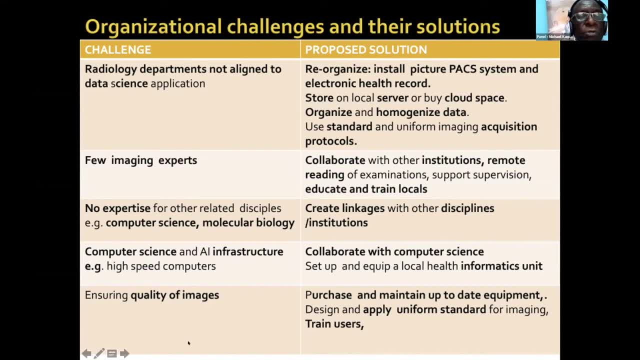 Organizational challenges on this table. we see radiology departments are not aligned to data, Data science application because this is new in Africa. So data has to be reorganized. We have to install a PAC system and also electronic health records. And these are not all over the country, all over the continent. 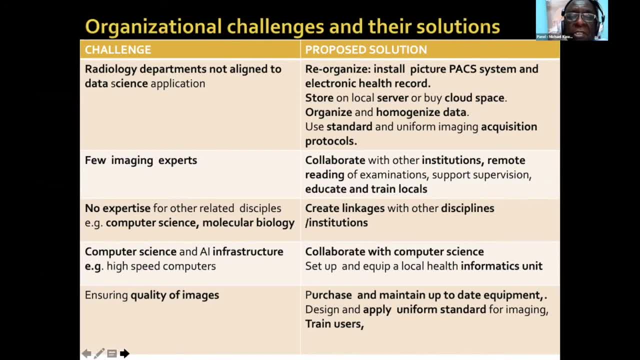 Many departments don't have PAC systems. The data has to be stored on a local server or in a cloud space, organized and homogenized. And then it's important that the imaging process We use to be standardized and uniformed so that data from different centers and from 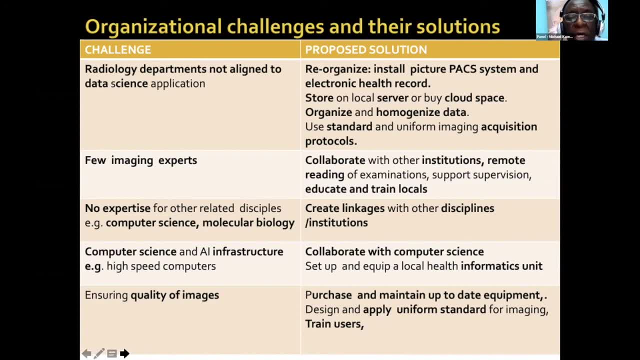 different machines can all be processed together. We also have a few imaging experts, and this one you can overcome through collaborations or you can use remote reading of images. And also it's important that you train locals to do the work and not only to rely on remote. 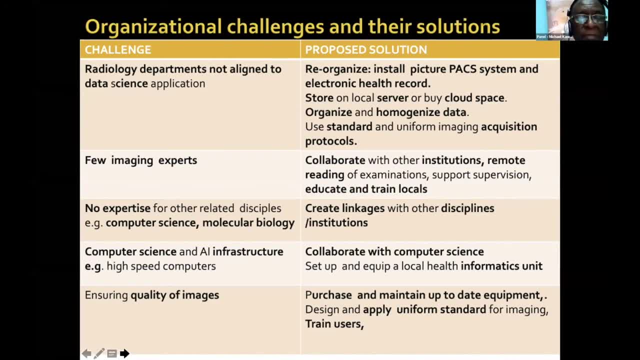 reading There is. in many departments there's no expertise in computer science, and so there is need for the department to form linkages and collaborations with computer science departments or institutions where there is computer science, so that they can access machine learning and. 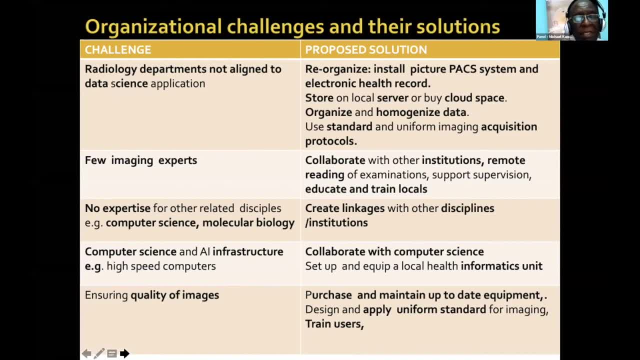 artificial intelligence facilities. Now, the computer science and artificial learning infrastructure requires very high speed computers. These are not usually found in radiology departments, Okay, But you can collaborate with a computer science department, and here one is usually likely to find high speed computers which can process data for machine learning and for artificial 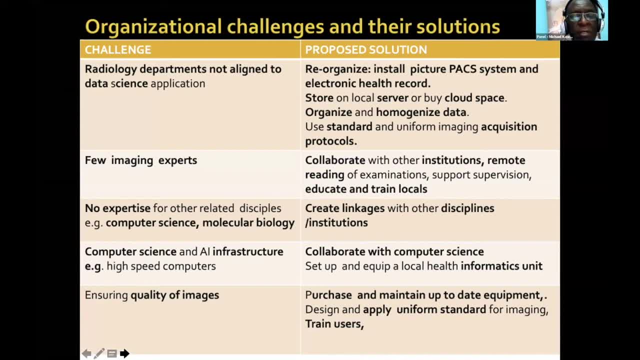 intelligence And the quality of the images in many parts of Africa still needs to be improved, and so there is need to purchase and maintain accurate equipment, and also design and apply uniform standards for imaging and training. Okay, So this is an example of how you can train the users, and this way you can ensure good 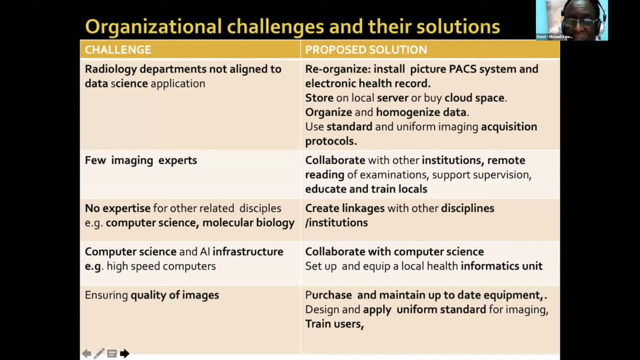 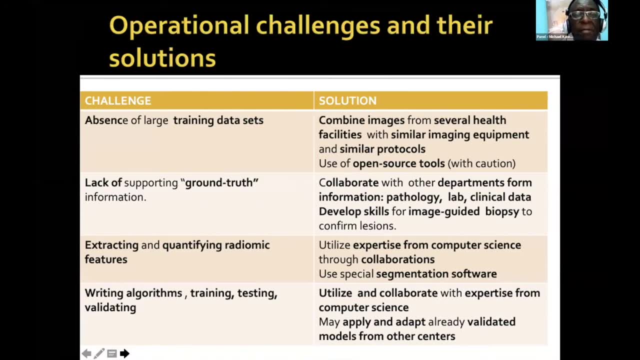 quality images which you can use in your artificial intelligence systems. There are operational challenges in this area- absence of large training, data sets- and so this one you can overcome by combining data or images from different imaging facilities, but ensure that they're using similar imaging equipment and also similar protocols. 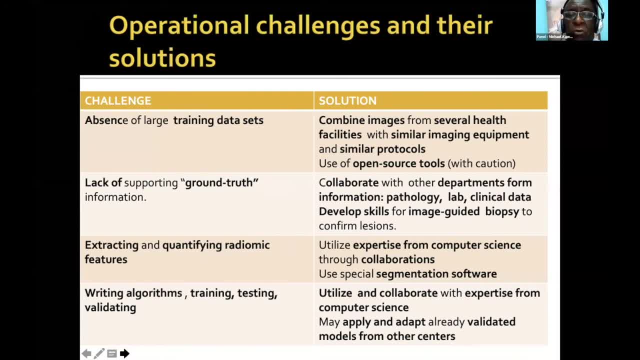 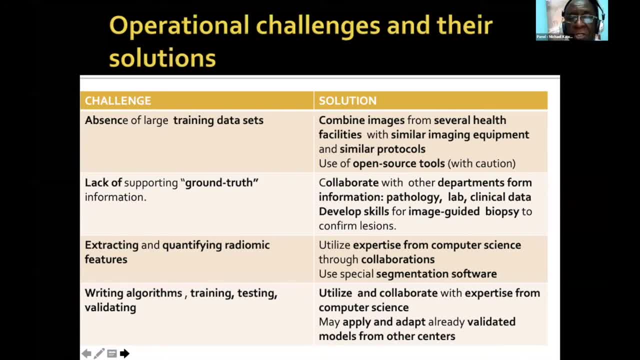 with the colleagues from pathology, from microbiology, so that we can – when we see an image there, we can be sure that either this is tuberculosis or this is cancer, through use of either pathology or – or imaging or microbiology. that is the ground truth to our imaging data. the data has to be extracted and 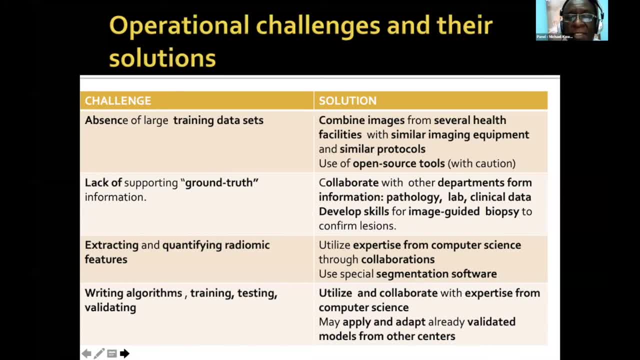 quantified, and here we use experts from computer science who can help us to extract data from these images, and also they can have computers with segmentation software to segment the images and then you can be able to to have this data processing, the machine learning artificial intelligent system, the writing of algorithms, training and testing and validating data. 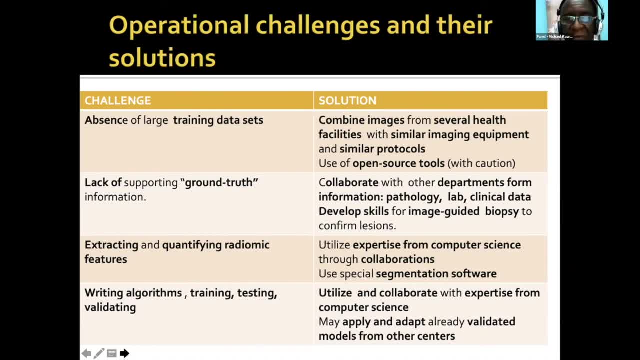 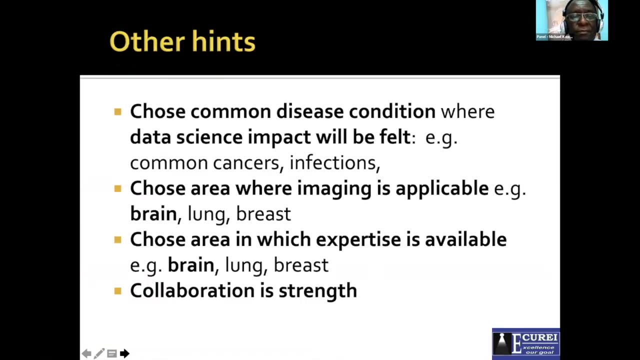 is not a skill which radiologists have or people in radiology, but then we utilize our colleagues from computer science who have the expertise to help us to write these algorithms, to train and to test and to validate that data. now some hints. if you want to undertake a project, 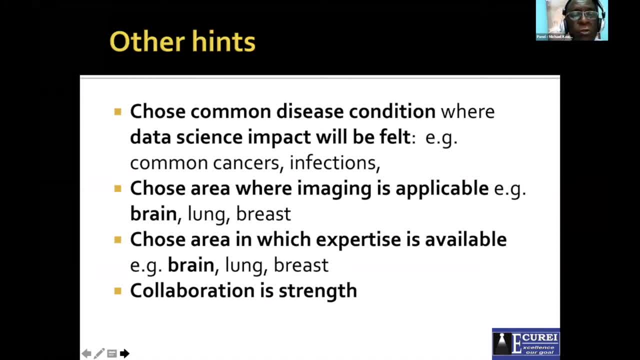 in data science. in africa you choose common diseases where the data science will have an impact, for instance, many cancers like cancer, prostate cancer, breast infections like tuberculosis. these are areas where data science may have an impact. we choose area where imaging is applicable, for instance brain, lung, breast. here we can apply imaging for the brain, like 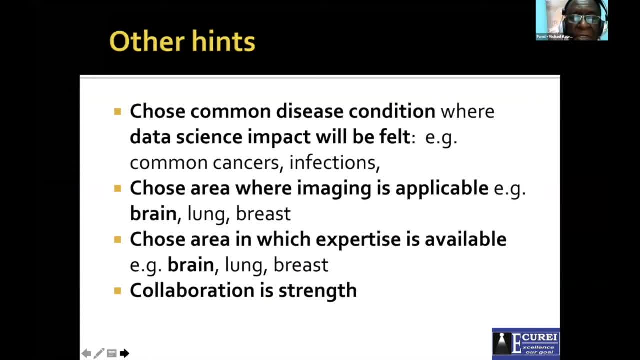 mri and city scan, chest x-rays and city scan for the lung and mammography and ultrasound for the breast, so that intersection between common disease conditions and diseases where you have imaging applicable, that's the area where you're likely to pick a topic to do your research in artificial. 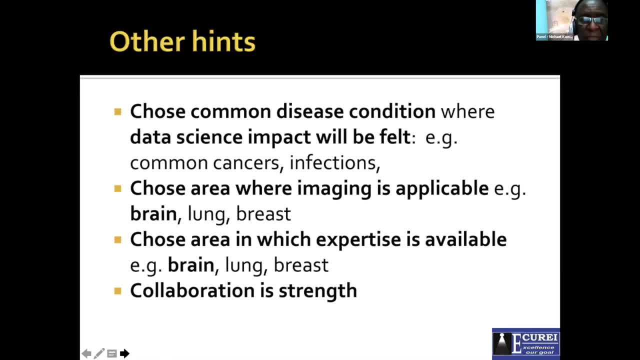 intelligence or to apply artificial intelligence and machine learning, and then you choose an area where you have expertise which is available, For instance experts for interpreting brain MRI or brain CT or experts for interpreting lung CT or breast mammography and ultrasound. And at times you may also need to link with colleagues from molecular biology for the molecular biology aspect of the tumor, also with colleagues from oncology and also with colleagues, of course, from computer science. 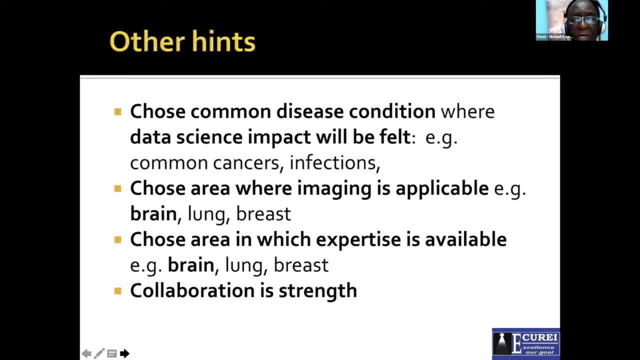 So you choose an area where you have expertise and you can undertake this project when you have all the capacity to do it, And then it's important to collaborate, collaborate, collaborate is strength, Collaboration is strength. You collaborate within the facility, you collaborate with other disciplines, you collaborate with other universities, with other centers and also with other continents. 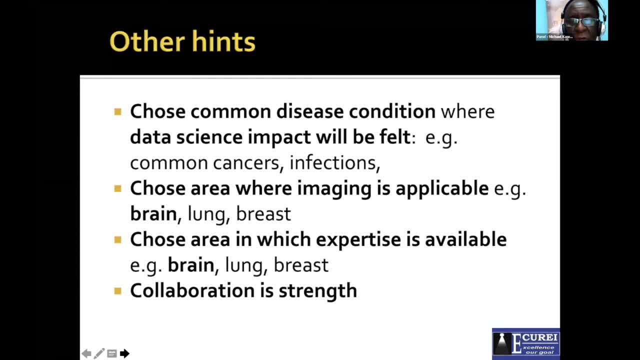 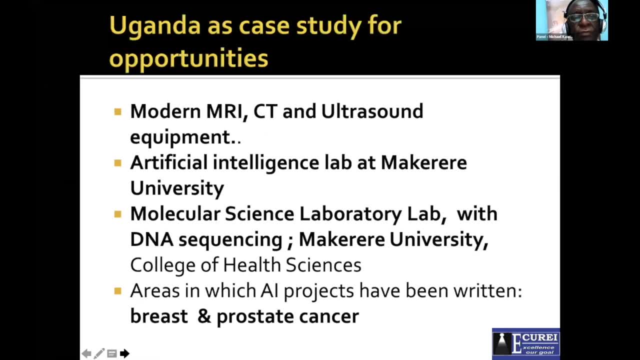 And then through this, you can have all the skill, the right skill mix, which you need to undertake a data science project. There are opportunities for many countries Like Uganda. here we have a modern MRI machine, CT and ultrasound equipment, so this can give you the set of images for you to use in your machine learning or artificial intelligence model. 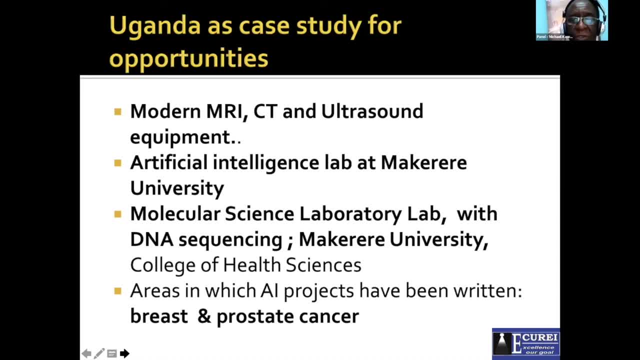 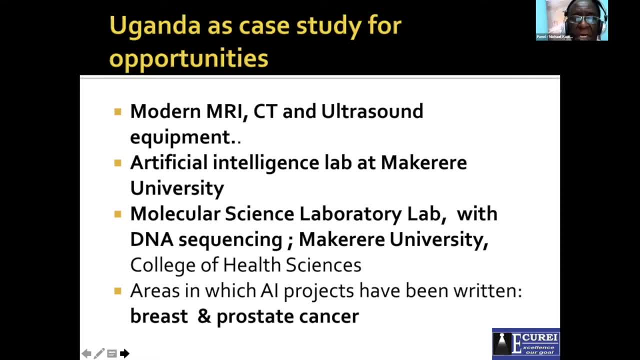 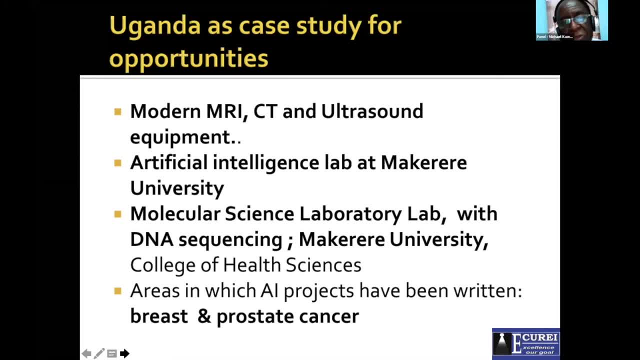 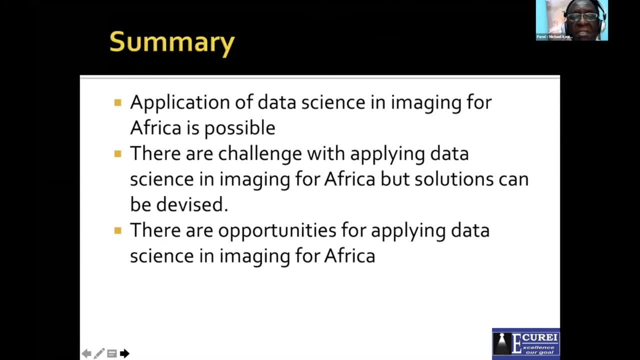 And for research And also for clinical applications. So, in summary, application of data science in imaging for Africa is possible. There are challenges that applied data science in imaging for Africa, but they're also solutions which can be devised, especially through collaborations. 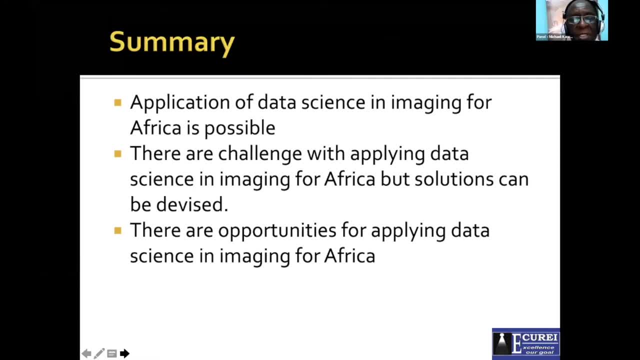 There are opportunities for applying data science in imaging for Africa And there are- I don't know- injuries, Fors, medical issues or circumstances, or medical disλλusions or pain, you know, I don't know- And this should be taken advantage of and this INH grant is a great opportunity. 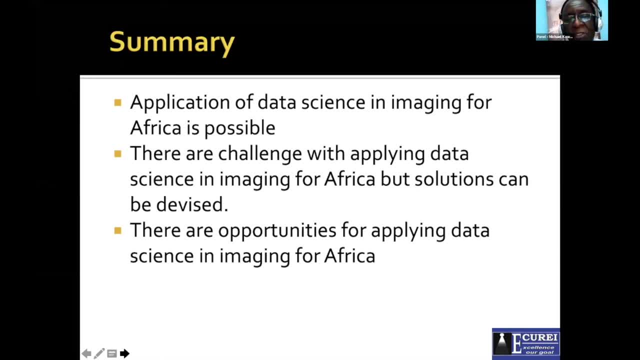 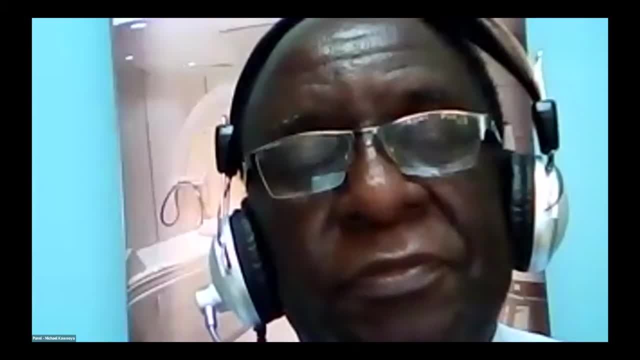 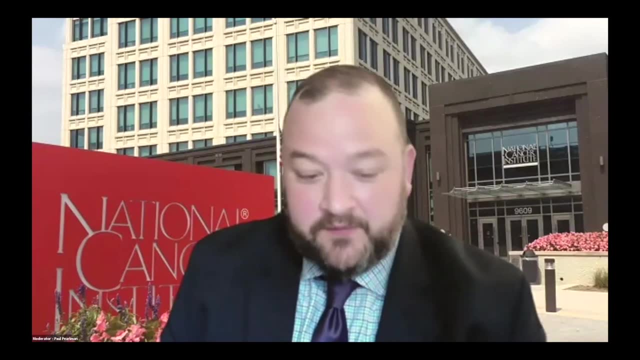 So I encourage you, I invite you, to come and join in and see how you can make use of this opportunity. Thank you so much. Thank you, Professor Kawuya. I want to remind everyone that the Q&A box is live and you can go ahead and start putting. 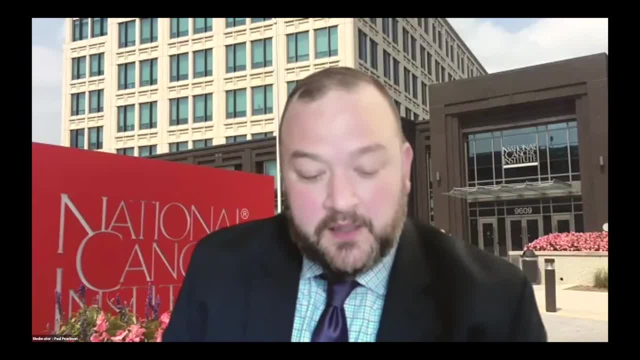 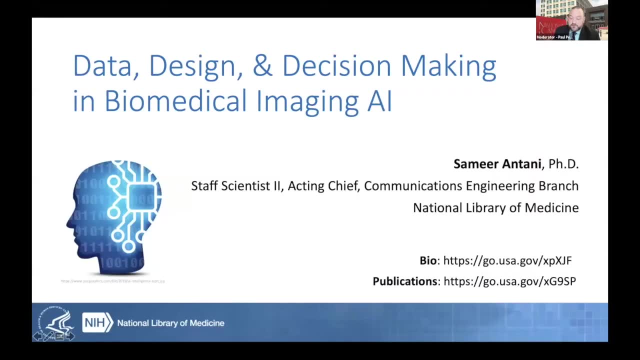 in questions as you think of them. So while Dr Antani is getting his slides up, I want to introduce our next speaker. Dr Samir Antani is an intramural scientist at the US National Library of Medicine with research interests in medical and machine learning for a variety of clinical problems. 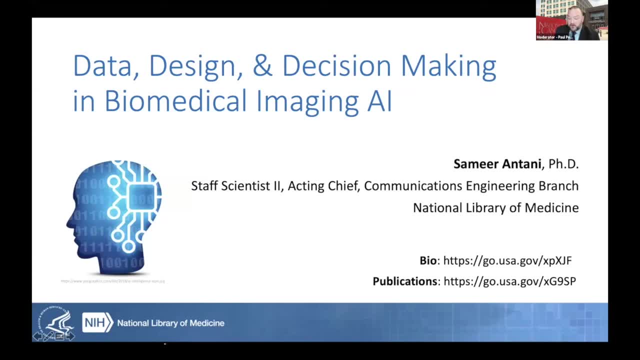 such as cervical cancer, HIV and TB, sickle cell cardiac myopathy and others. Samir, Thank you very much for the introduction, Paul, And welcome everybody. Good afternoon to everybody in Africa and good morning to the people in Europe. 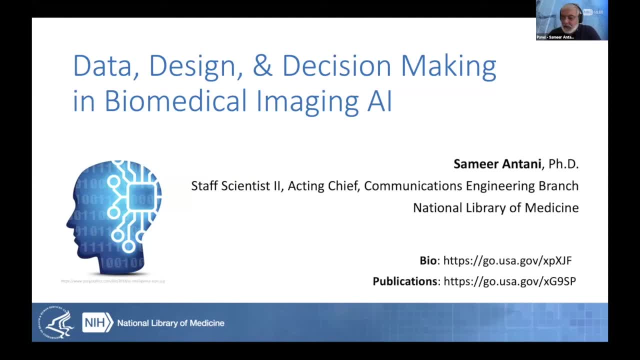 And welcome to the world as per your time zones. I'm going to talk about several aspects in biomedical imaging AI that relate to data science, to do with data design and decision making and the interaction between them, And I'll draw on some of my experience as an intramural scientist at the NIH working 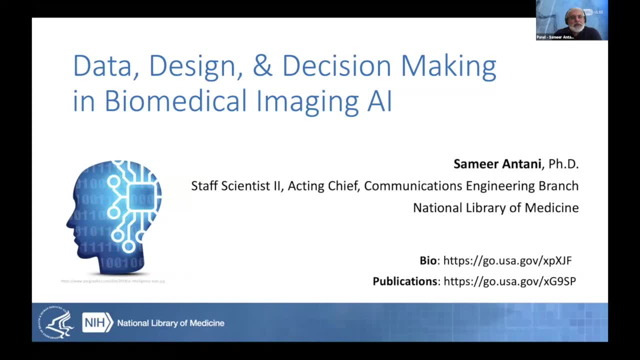 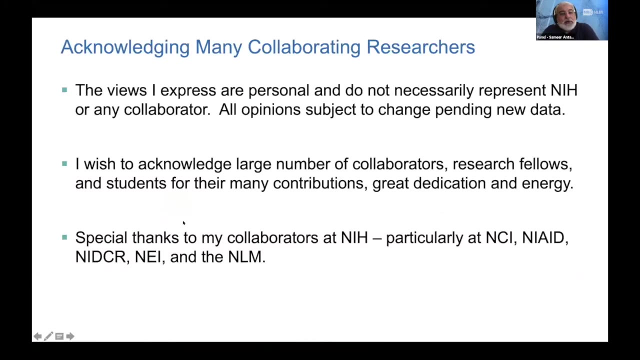 on some of these biomedical imaging AI problems And to help you think about your problems or your challenges as you embark on this journey. So before I go too far into my talk, I would like to acknowledge that what I'm drawing on are my experiences that I have derived from many, many collaborations over the past. 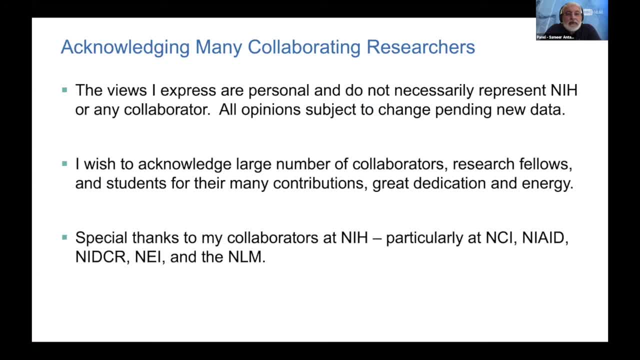 over 20 years And my views are personal. They do not necessarily represent the NIH or any collaborator in particular, And, as this is a rapidly evolving field, my opinions are subject to change as I learn more and we all learn more in this area. 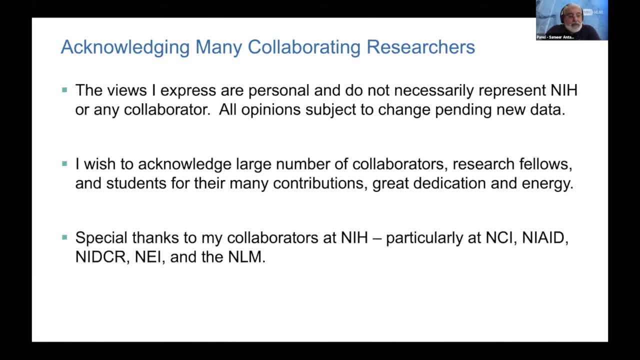 And the collaborators are many and they are varying from students who come from different parts of the world to research fellows and other organizations And within the NIH. I must acknowledge that there are a lot of people who are interested in this area And I'm going to talk about some of my experiences. 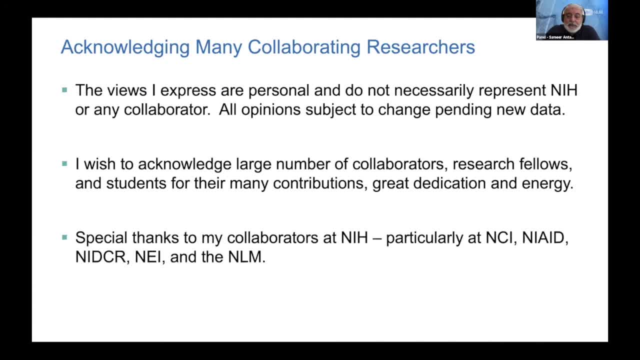 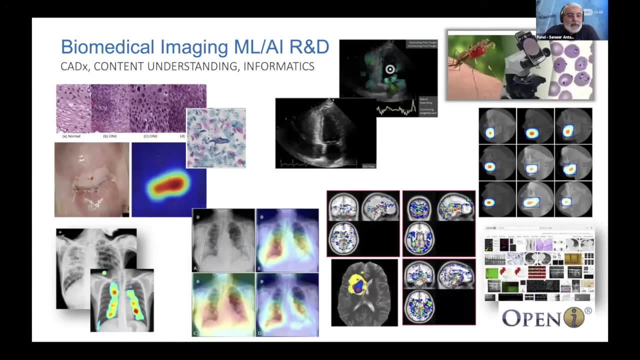 I want to acknowledge my collaborators at the National Cancer Institute, the National Institute of Allergic Infectious Diseases, Dental Craniofacial Research, the Eye Institute and the National Library of Medicine, of course, So this is a rather busy slide in images, but I'd like you to think about various imaging. 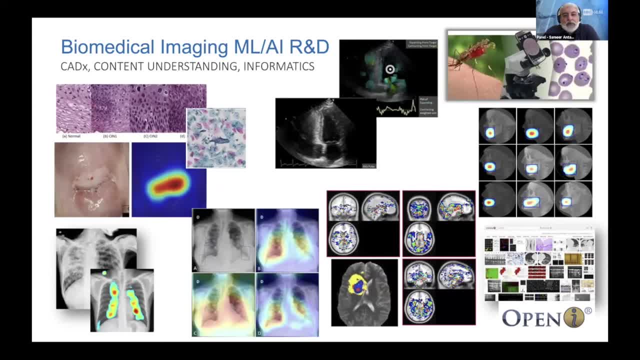 modalities that you see here and how one would process these images. On the left you can see top left a histopathology image. That's from a biopsy of the uterine cervix to do with cervical cancer, and I'll touch 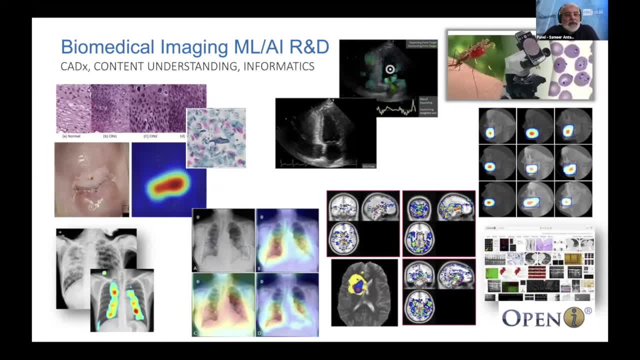 upon that a little bit. You also see a small swatch of a microscopy image from a cytology, from a typical pap smear- a liquid pap smear perhaps, or a traditional photograph of the tissue. You go into chest X-rays looking for disease patterns and onto 3D volume images from the 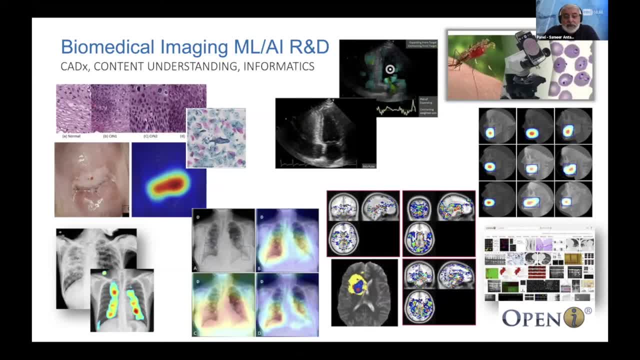 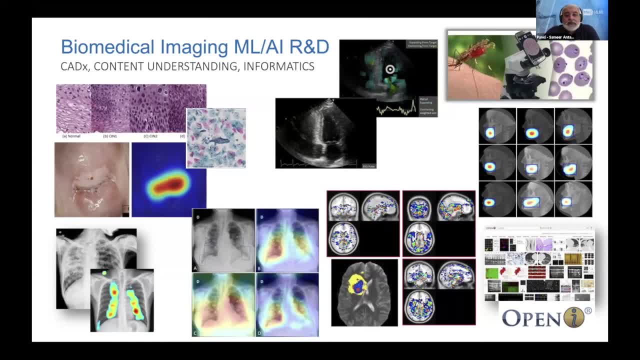 so that you can see more clearly. So what are the main problems? The second one is skin problems. This is the most common problem with the brain when you have a brain. I'm going to show you the second one video, but also an EKG that is embedded in there. That would be one-dimensional. 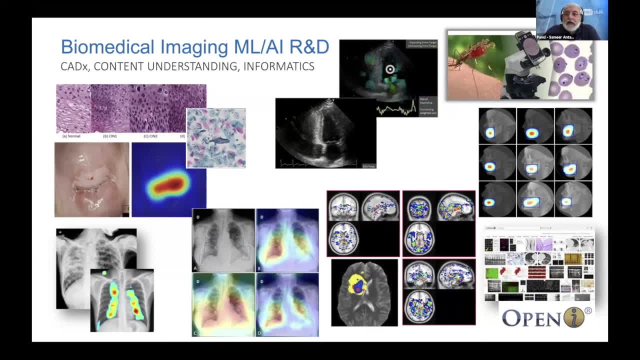 signal data that one might need to process, And the processing can be done using, of course, supercomputers or desktop PCs equipped with GPUs for processing, or even mobile phones- as exemplified in our ongoing work in detecting malaria using smartphones- And sometimes there are data that are involved in multiple 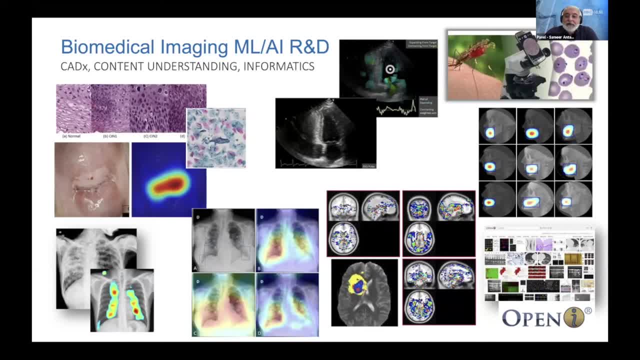 dimensions, and once you have collections of these images, one might want to access them using textual means. if you have metadata tags, or you may have patient health records, or you might want to recall them by their appearance, You it's very natural for us, as we look at it, to do that. 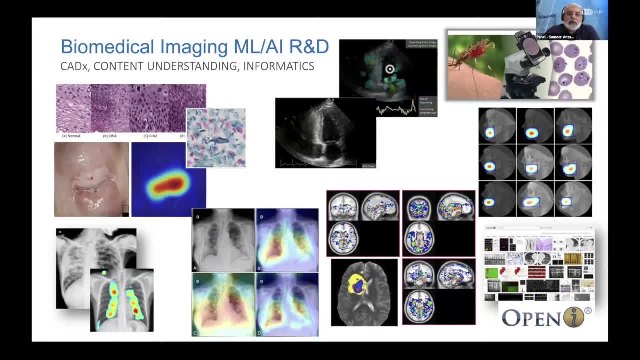 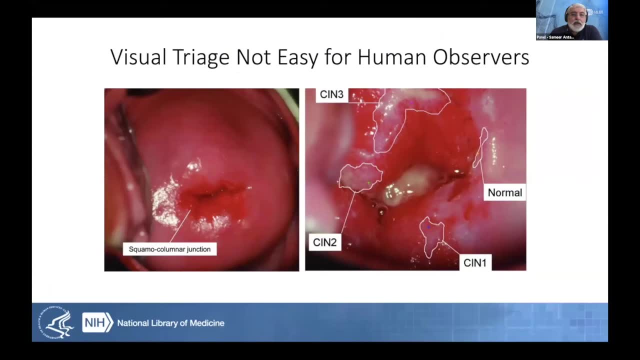 at pictures to be able to recall what something looked like, and that is the field of image understanding, or content based image retrieval, which is something that the open eye system tries to do in trying to connect words and pictures which are natural to us as humans. so with that background, I'll take you. 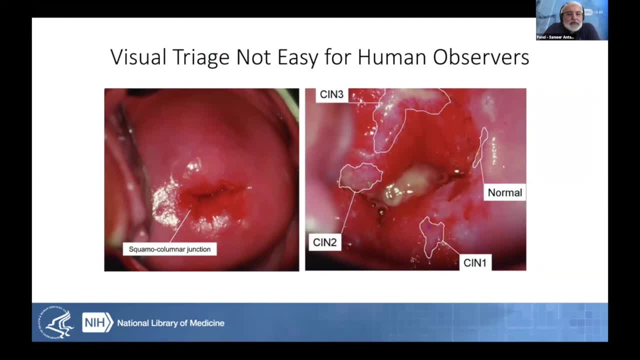 into on a journey which is to do with detecting cervical cancer or, more importantly, pre-cancer, since that can be treated. now, what you're looking at in the left is the picture of the different civics as seen by an ecologist or gynecological oncologist during the routine exam, and what you're seeing 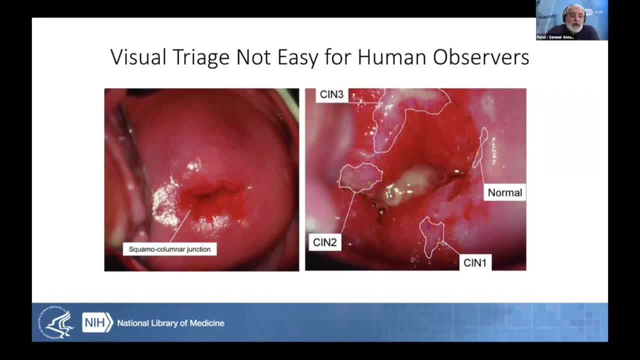 there is the dark region in the middle is the us, which is the entrance to the uterus, and what you're looking for are changes in the epithelium, the squamous tissue there, and there are two tissue types: the columnar cells and the squamous cells, and it's at this junction that you begin to see the 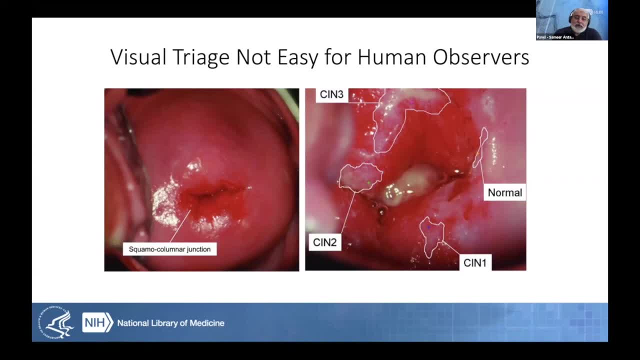 invasive effects of human papillomavirus, certain types of them that are particularly oncogenic and can lead to cancer. and on the right there are some regions that have been marked by an oncologist for us grading them as stage one, stage two and stage three. it's after stage. at stage two and and beyond is 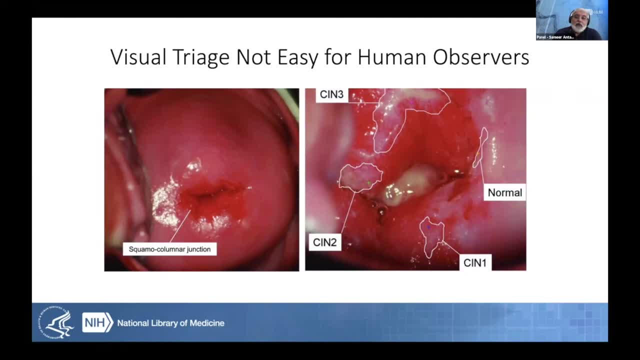 what we start labeling as pre-cancer, where one would want to treat, and using thermal ablation perhaps, or cryotherapy, so that any further damage is is eliminated and the woman can resume her normal life. and but we this is called visual triage, but it's not so easy for human observers and 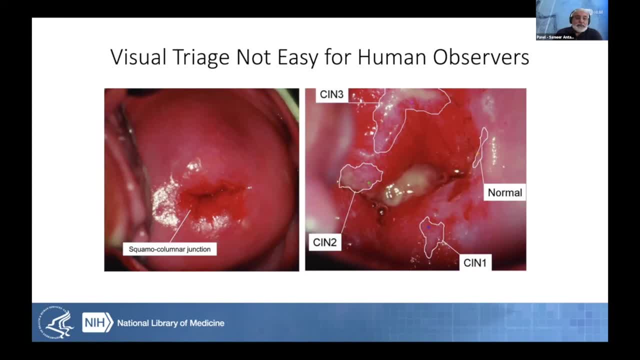 there is great subjectivity and of course this presents a good opportunity for computers to intervene and perhaps highlight regions, those who may have been less trained to, to provide some objectivity on how to detect disease and and where they can be treated. so there was some work done in the past, well over 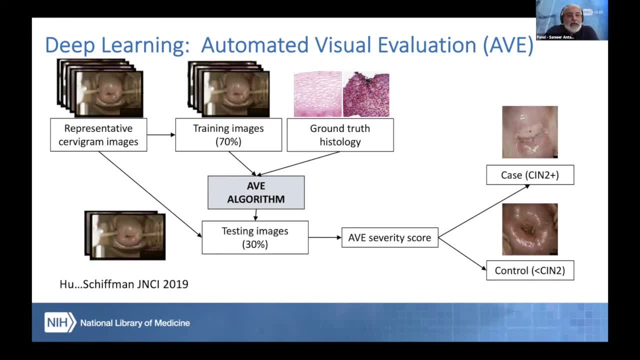 two decades now, but more recently. there was some work done in the past- well over two decades now, but more recently we had a breakthrough in using a deep learning algorithm, which is a neural network algorithm, also known as an AI algorithm- that looks at an image and is. 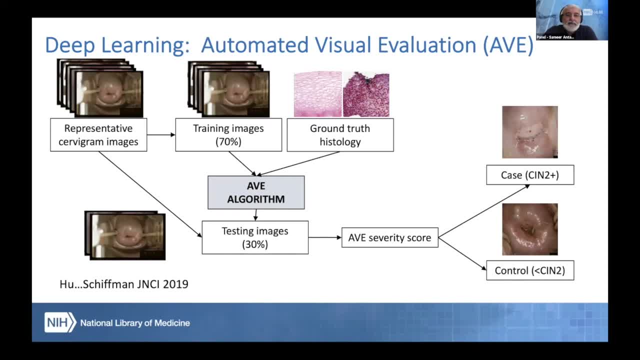 able to provide an ABE, or an automated visual evaluation severity score that predicts that an image is either a control that means normal, or is a case which is deserving of treatment. now, to train this algorithm, we need to train a. we need to train a. of course, we had a large collection from a seven year study conducted by the 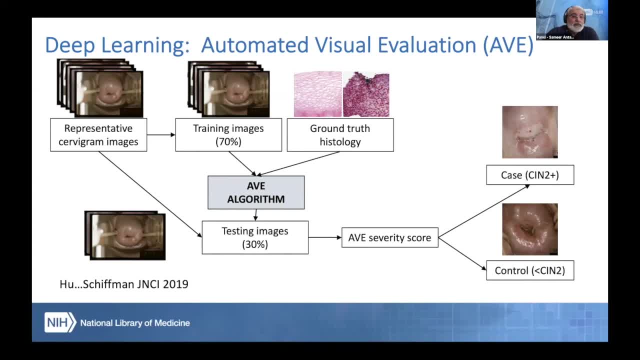 of course, we had a large collection from a seven year study conducted by the National Cancer Institute in the Guanacaste region of Costa Rica, and seven thousand women- nearly ten thousand- were followed over seven years, and the collection of images from every visit were then grouped into training images. 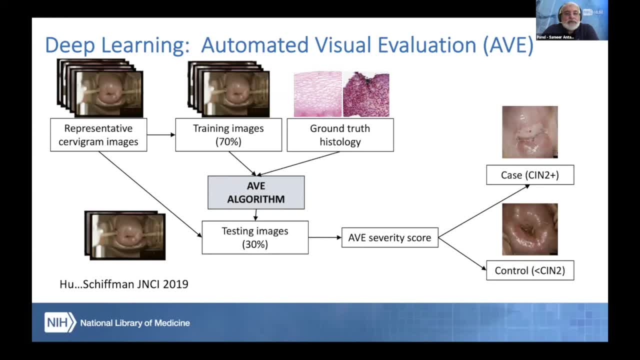 that were truthed or they were those that were indeed cases. there were biopsy truth that was applied to them and those selections were used to train the network and tested them so that it has very high performance, and the performance is shown on this chart here. 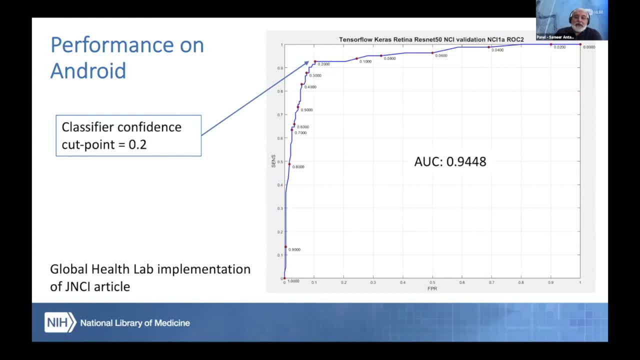 This is known as the ROC or the receiver operating characteristic curve, which plots the sensitivity of a test versus the false positive ratio on the x-axis, and you want this curve to be as much of a right angle, heading toward the one here or the top left. 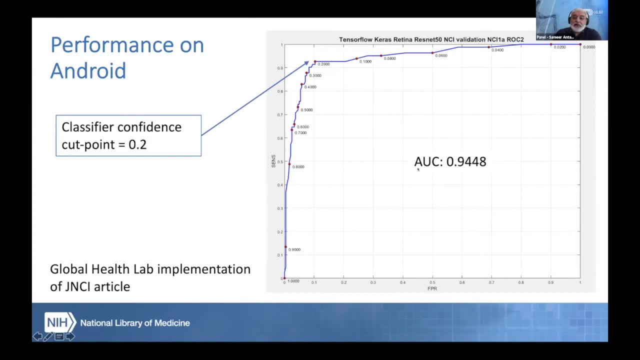 And, as you can see, this algorithm has a very high area under the curve, or the AUC of 0.94.. That means it is making very few mistakes. Now, that said, now, this is what, if you were looking at many deep learning papers, that 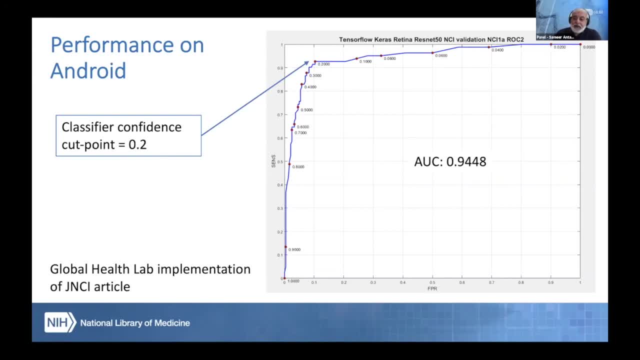 what you would be trying to track. however, this alone is insufficient. It's also important. It's important to see where you are having the thresholds set up so that you perform well, And in this case, the classifier was confidence was reduced to 0.2.. 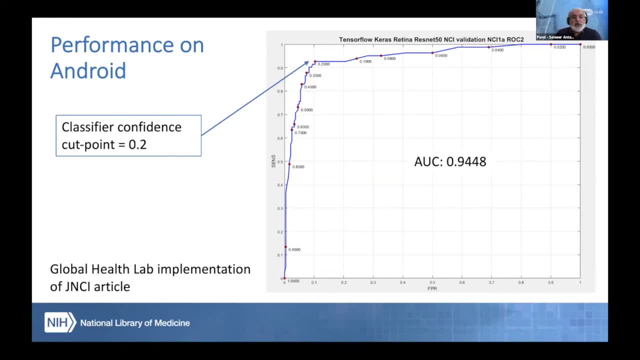 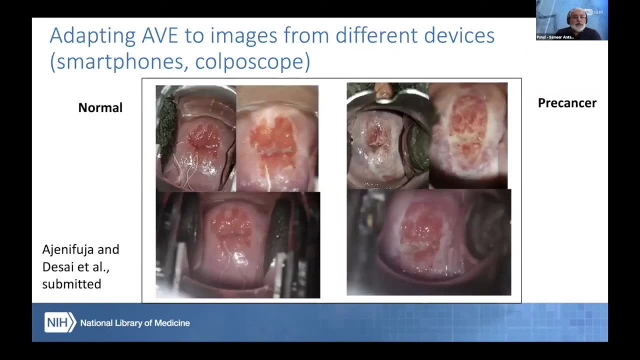 Normally you would want to be a classifier, to be very confident to be able to achieve this high a score, and that is a factor that's important. Also important to note is the variety that different cameras can produce on an image, and you would want to train your classifier with as many samples from different camera. 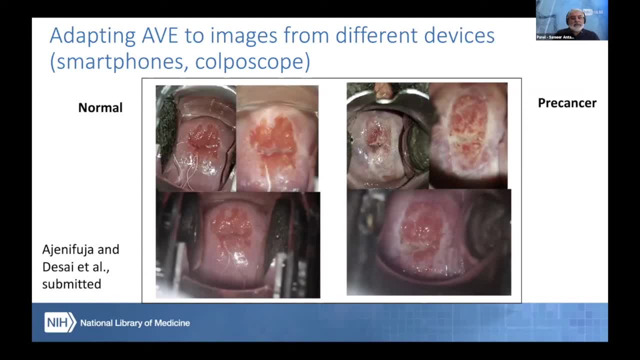 sources so that you have a sense of robustness and reliability in the performance of your AI algorithm, And this also alludes to different kinds of data that you need to use to train your method so that it doesn't do very well on a small kind of a set of images, but a broad variety. 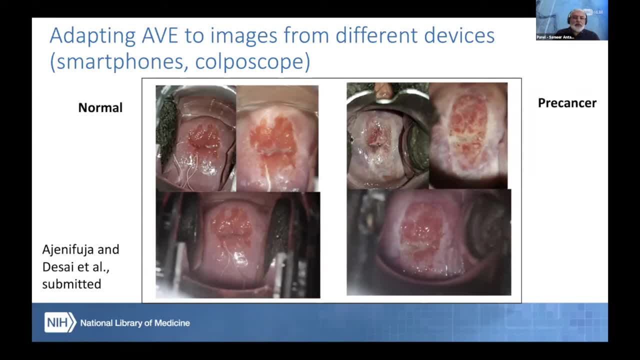 of images. that represents the population that you are building the algorithm for, So this is a very important point. Thank you. Any other comments? Paolo Davi, OK, Yes, These are the three key più points, and they're very important for clinicians. 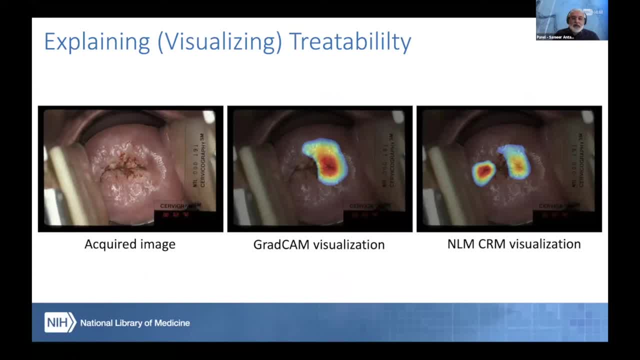 In each. you can look at down the graph for the fine picture that you wanna have, absolutely an image of. you know a cancer in clinical development, and you can go to the specific Stanford evil. or you can take the cancer's whole profile and say that AI and con'oc. 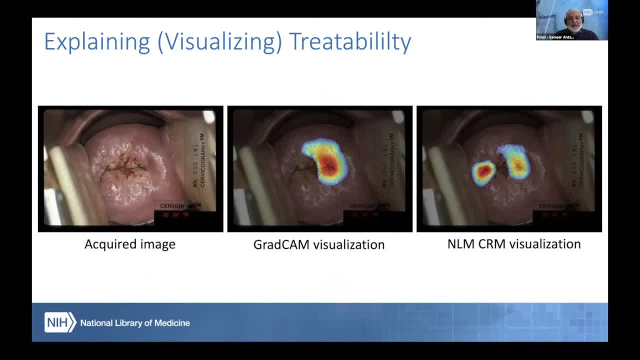 touch orativa examination and the medical status must be legitimate. Okay, But interestingly enough, each AI algorithm was highlighting a different region of the image, which, of course, introduces doubt, And that's why it is still an area of research. 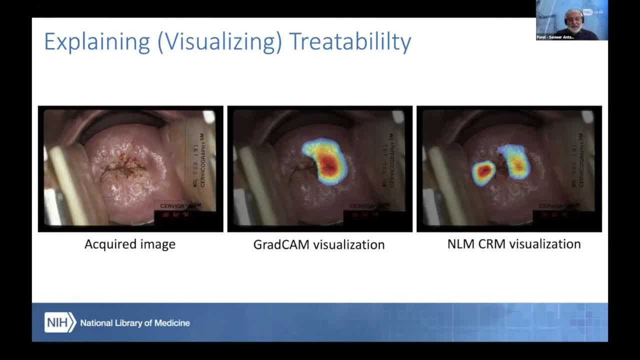 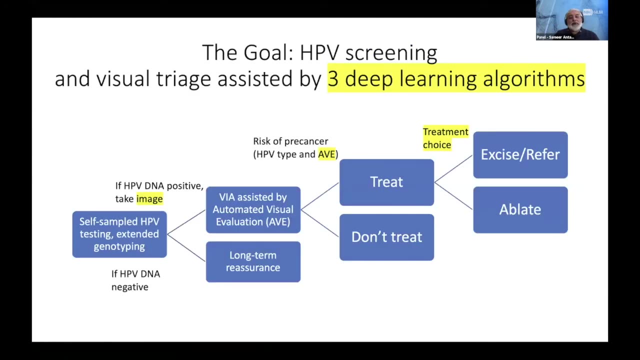 But AI can help you classify something correctly, But it's also important for you as a researcher to focus on why it is classifying an image as a case of a control and what region it is highlighting that is worthy of treatment. So if you think about this problem now, from going from the left to the right, you can see an image has been acquired. 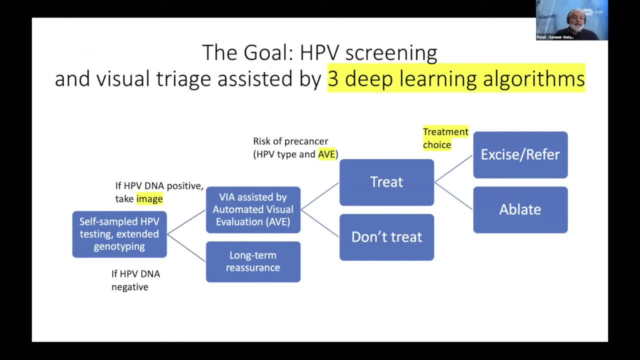 And there is an HPV DNA test done And if the person has HPV positive, then we would like to be able to decide if the person should be treated or not treated. That means the case of a control And then, if it is treated, there will be a second algorithm that will be determining if the region should be examined. 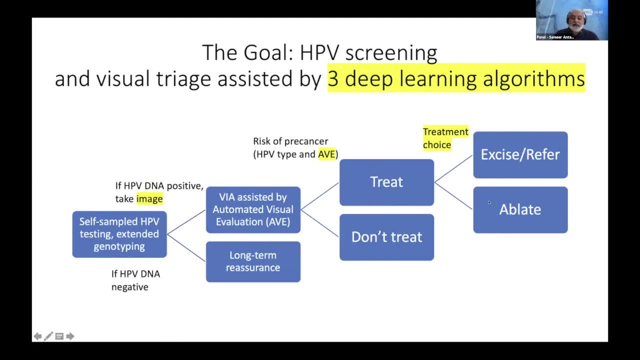 And that is the size, or thermally ablated. And so you have different kinds of algorithms that have been trained on different kinds of data: images, as well as HPV data, which may be textual in nature, that are informing the clinician to make a better judgment and provide for treatment. 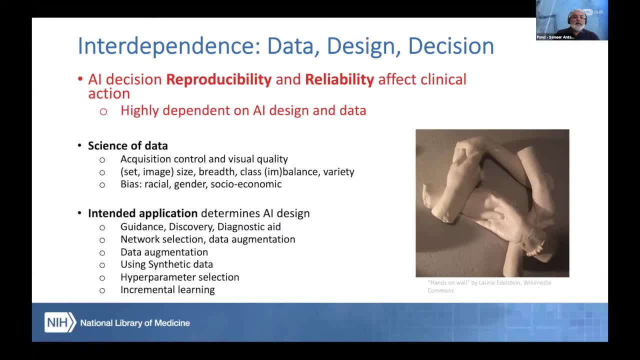 So what I'm going to highlight here is the high interdependence among the data, the AI design and the decision that is produced, so that you have a highly reproducible and highly reliable data, And so the byproduct of that is that if we are able to build an HIV-resistant approach that is not yet cognitively sensitive, then what we're trying to achieve is a highly verifiable outcome from the AI that can help affect clinical action. 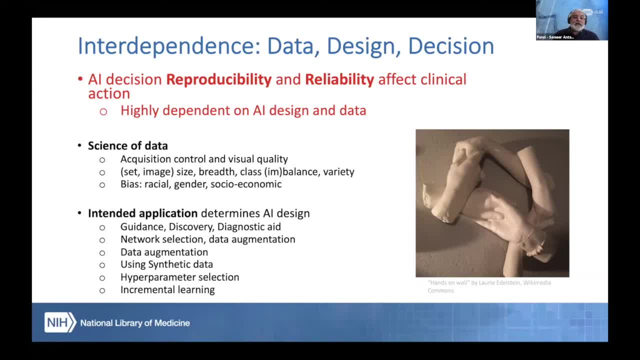 And in thinking about this we use the word data science, but I like to try to think of it as a science of data. It is acquisition, control and the visual quality of the data, How large your set size is, for treating large is the set size. 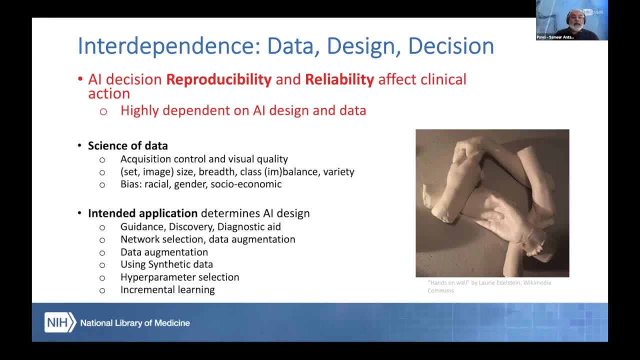 necessary, statistically speaking, to get the reliability and robustness from the algorithm. You also want to think about any racial or gender or socio-economic variety that might be introduced there which can affect the quality of the images And, in terms of thinking of the AI design. what is the? 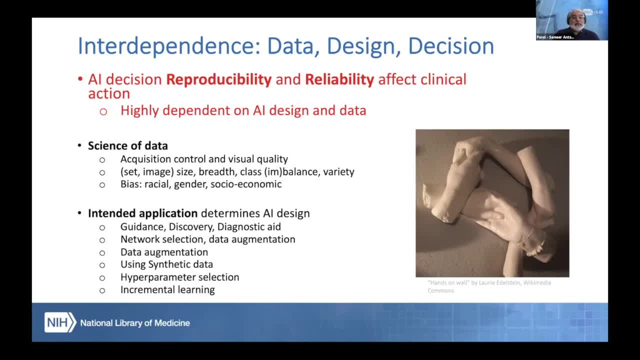 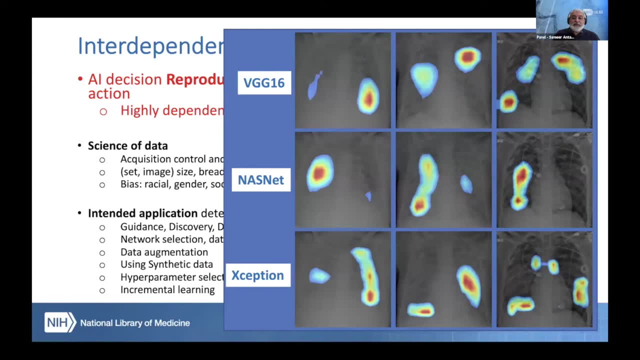 intended application? Is it for discovery, which is research, or is it diagnostic aid? What kind of networks I'm going to use? And this is an example where you have different kinds of networks. Looking at chest x-rays in this example, how each 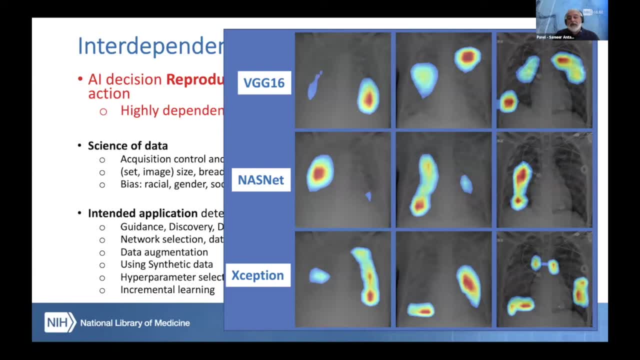 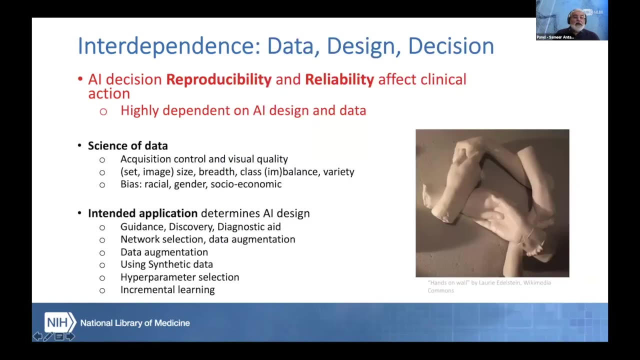 network or each AI algorithm, ended up showing different, highlighting different parts of the image. All had disease, yes, and all were correct, but they all were highlighting different aspects, And so the application is extremely important as well. If you're going to be using synthetic data, does it really represent? 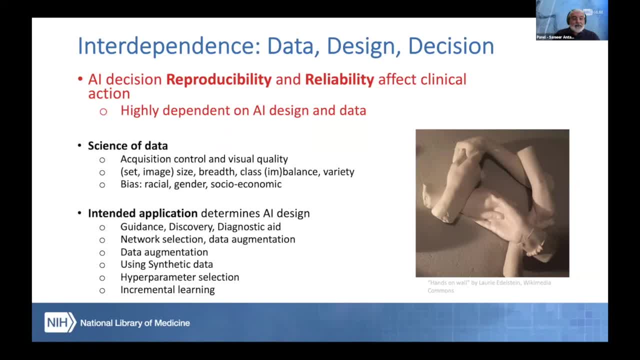 reality. How are your hyperparameters trained for your deep learning algorithm And how would you learn incrementally? That means humans correct machine. the machine learns to adapt and evolve over time is also a technique that needs to be researched and considered in designing an AI algorithm. So I'll leave. 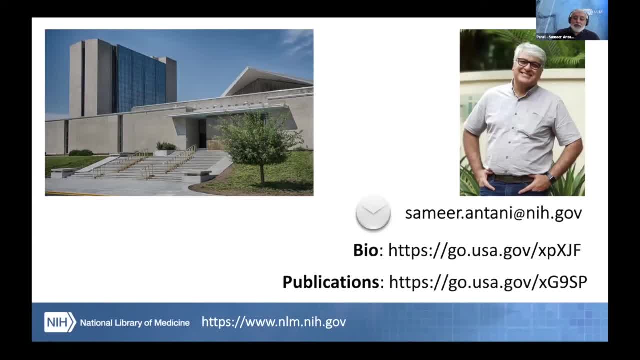 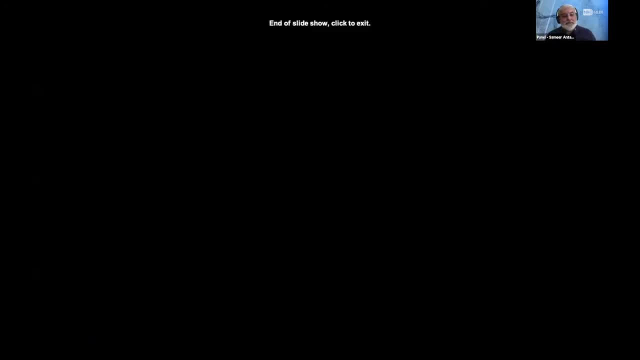 it there and here's my contact information. but before then I invite you to join Network Lounge and interact and have a chat. Thank you for attending. Thanks, Sameer. As Dr Cintas is getting her slides up, I'll go ahead and introduce her as well. 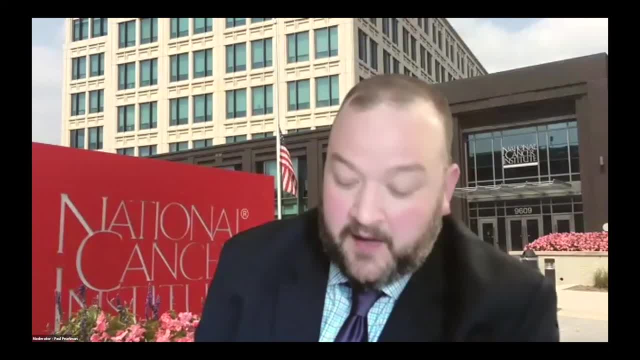 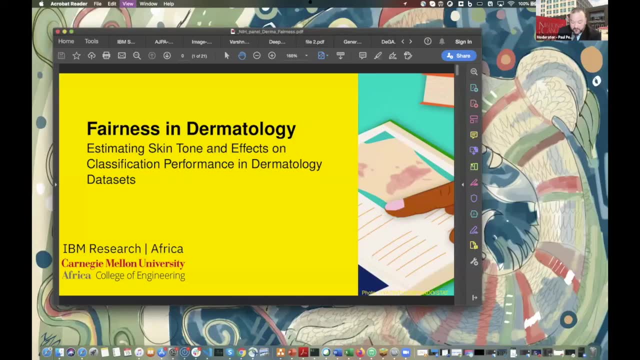 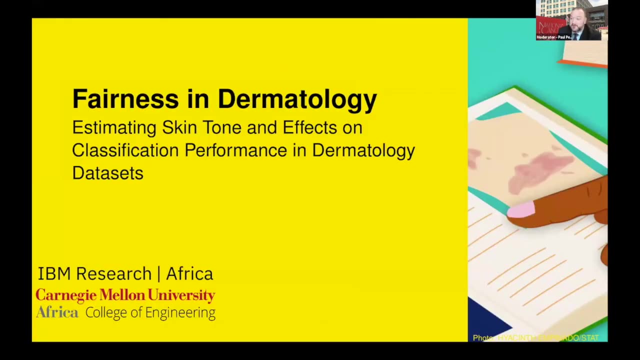 Dr Celia Cintas is a research scientist at IBM Research Africa in Nairobi. She's a member of the AI science team at the Kenya lab. Her current research focuses on the improvement of machine learning techniques to address global health challenges and exploring subset scanning for anomaly detection under generative 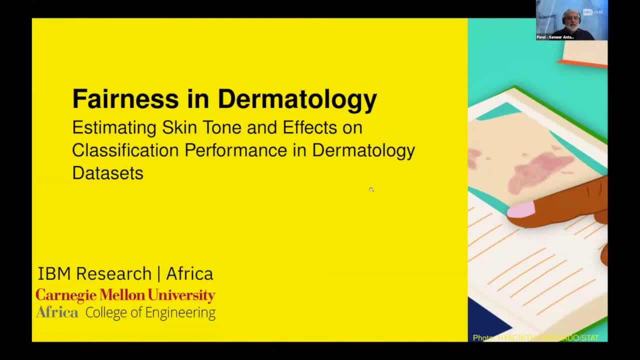 models Celia. Thank you, Paul, for the introduction. Good morning, good afternoon. In this talk we want to discuss fairness in dermatology and how machine learning models are built for a skin disease diagnosis And to see if there is an equal skin tone representation. 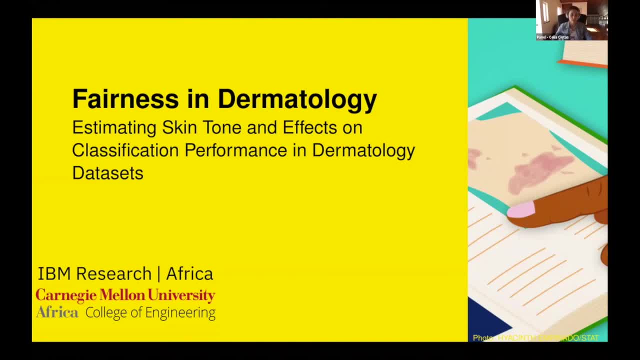 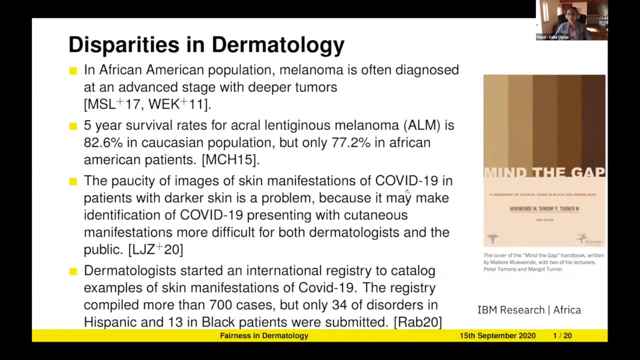 in these datasets. This work was jointly done with the College of Engineering of CMU Rwanda, IBM Research, both Yorktown and Nairobi labs. Thank you, Thank you. We know that in dermatology, as in other medical fields, disparity exists across ethnicity. 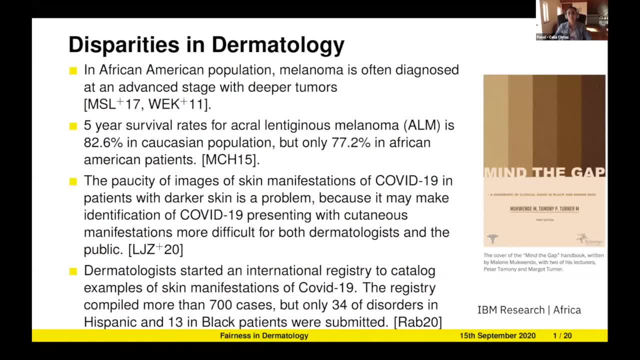 For example, in Black African American population, melanoma is often diagnosed at an advanced stage. Survivor rates of ALM occur in African American Caucasian populations. Due to COVID-19,, dermatologists started an international registry to catalog skin manifestations of skin. This registry compiled 700 cases, but only 34 of them were Latinos and 13 from African American patients. 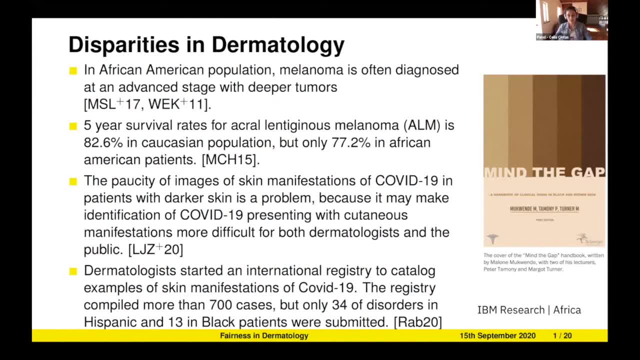 Professionals are raising concerns regarding the issues in the medical space. An excellent example is Mind the Gap, a handbook for clinical science in black and brown skin, written by Malone Mugwende. As we know, machine learning systems are very complex. They are very complex. 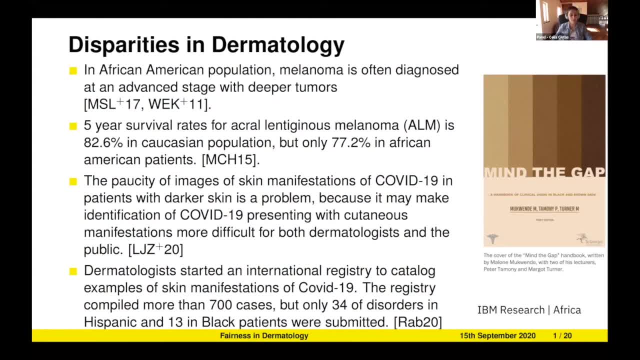 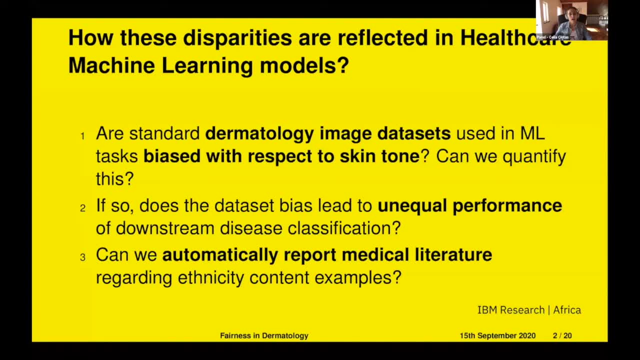 They are very complex. The reason is that these systems may place certain groups of people at systematic disadvantage due to the bias of datasets. So we want to see how these disparities are reflected on the healthcare machine learning models. First, we want to check if the standard datasets used for machine learning tasks in dermatology are biased with respect to skin tone, and can we quantify this? 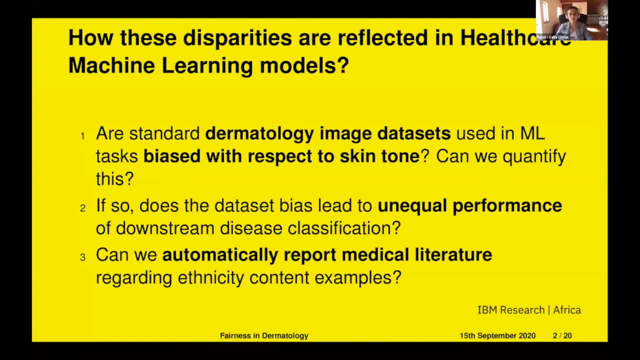 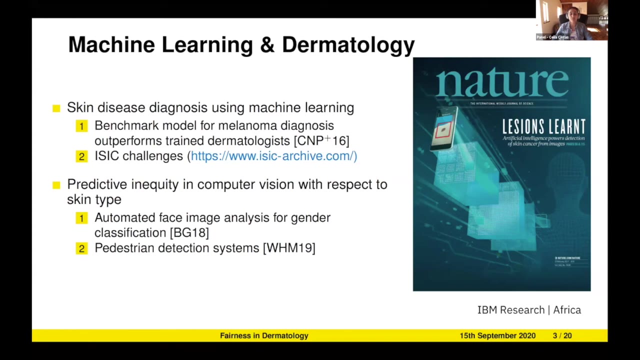 If so, does the dataset bias lead to a learning disadvantage? led to an equal performance of the disease classification, and can we provide an automatic report of medical literature regarding these ethnicity examples? From the machine learning perspective, recent advantage on computer vision and deep learning led to breakthroughs in the development of skin. 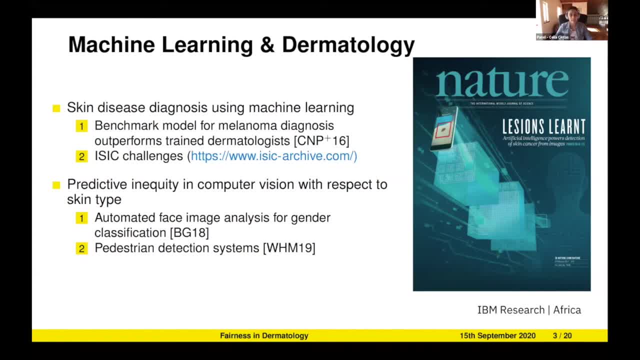 image analysis and diagnose. For example, in melanoma we have benchmarks models that outperforms training dermatologists Since 2016,. we have the ISOC challenges that show problems on facial segmentation, clinical diagnoses patterns and lesion classification. On the other side, we leverage work on productive. 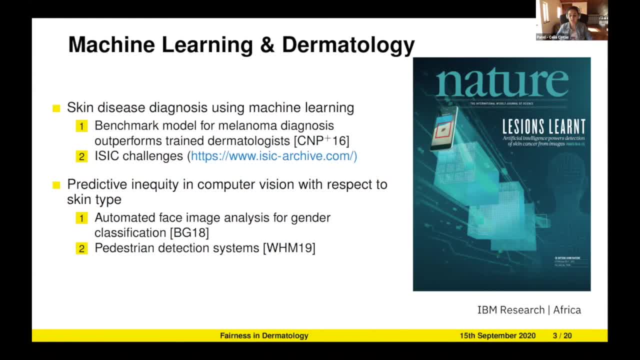 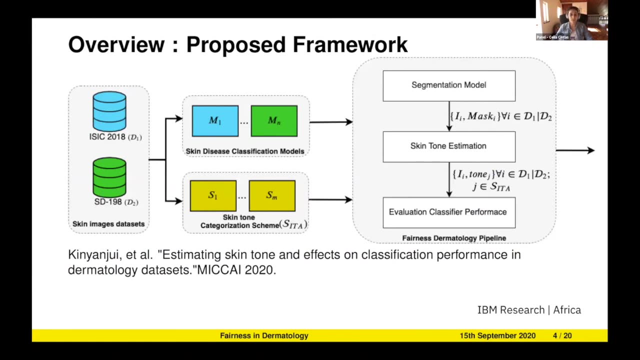 inequity in computer vision regarding skin tones. This was proposed by Joe Buolivities and Timnit Guebru. So what we? what we want to propose is a framework to estimate the skin tones and their effects on classification performance in dermatology data sets. this work was led by tim and newton. they will be presenting 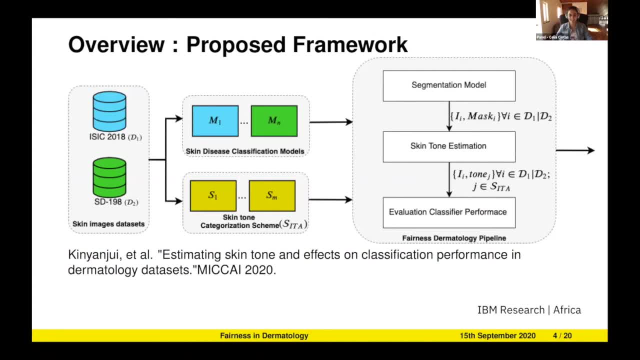 in much more detail at mikai 2020 on next month, but the main idea to have this framework ongoing is based on three steps. first, we need a segmentation model to be able to extract the non-disease skin reactions, to be able to estimate a skin tone metric. and after we have this, 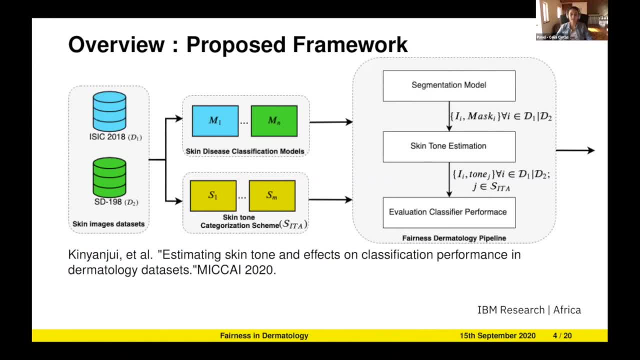 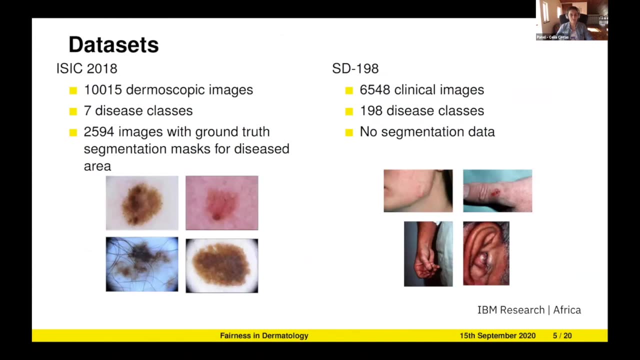 information we can do a stratified evaluation to see that the skin disease classifiers are working correctly across all the skin tones. so to evaluate uh this proposed framework, we use two common data sets in dermatology isic 2018 with multiple thermostatic images across. 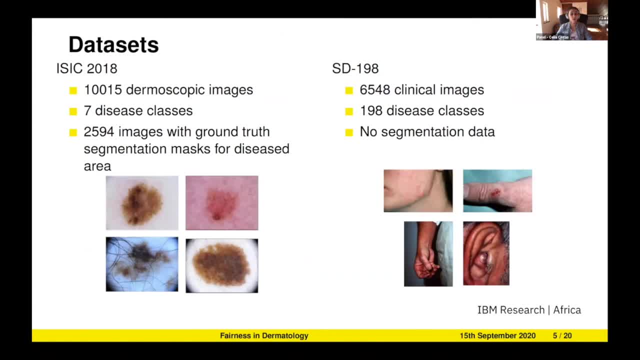 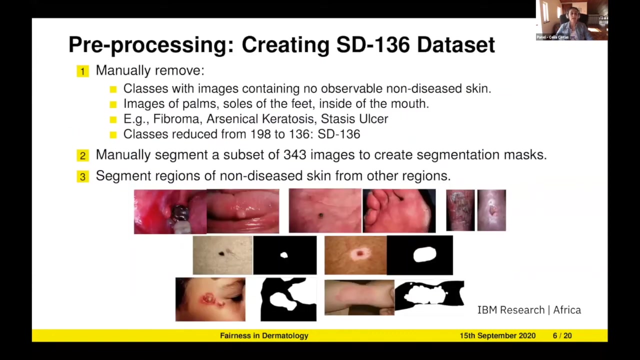 seven different diseases labels and a subset of images with ground truth of segmentation masks. in the other hand, we have sd198 with multiple clinical images over close to 200 disease classes, but with no segmentation data. for our purposes, we need to run some manually preprocessing before using them, such as removing classes with images that we don't have observable non-disease skin. 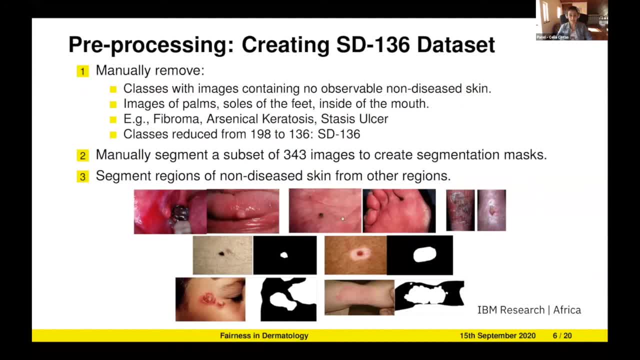 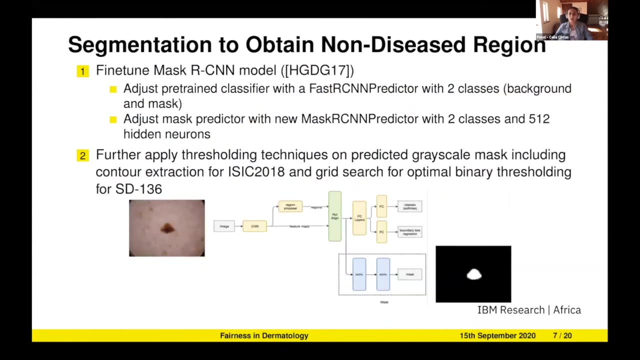 reactions and we also removed specific body parts, such as inside the mouth, as you can observe here, and we manually segmented a subset of these images to create our segmentation mass. ground truth: first, our, our, our module for segmentation to obtain the non-disease region. we need to have a segmentation model that is able to detect the non-disease skin reactions. 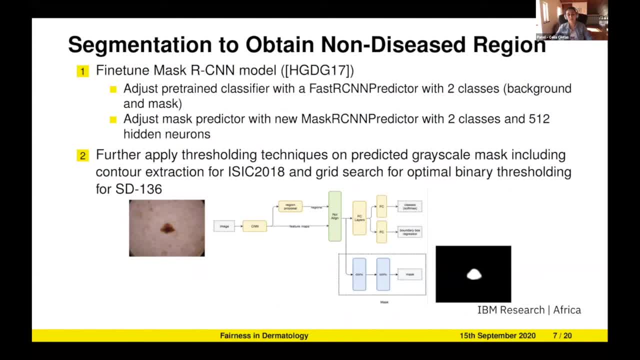 to treat skyscrapers, then exporting the unknownctor in our batches, so it will express the違う image found in relação to these places. in this many of these different models. in a non-disease糯 net model, you can casually start to capture all of the animal. 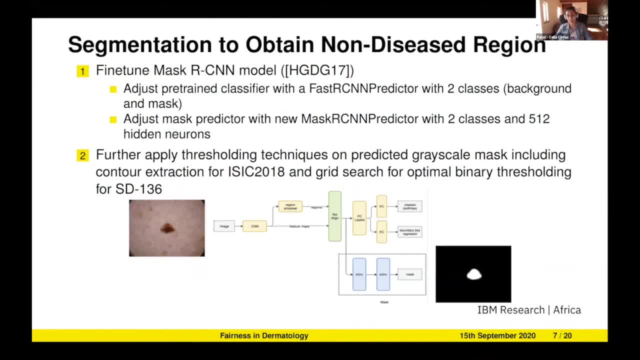 granules or any otherТы'll look at in this being an example, an image can be bone-tested, where the reproductive, once it's treated, it reflects things like static blood literature as well as local blood data. we, Så we'reÜ, can then regulate the tactics we perform with that and cause some changes to the 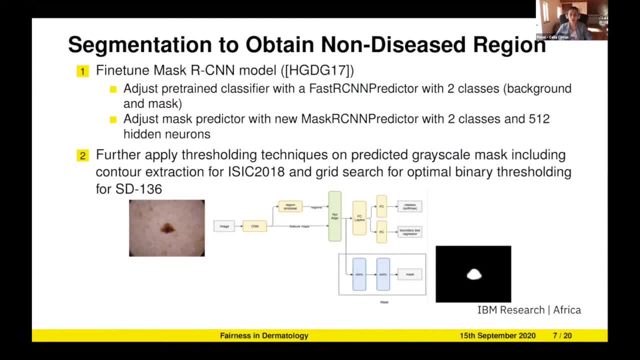 infection and are individual cases that are unές 듯. they can be searchable or they can be aromatic, and we are auch, As the output of this network is a grayscale mask. we actually need to apply some thresholding techniques to extract a binary sample, as we see in the bottom right. 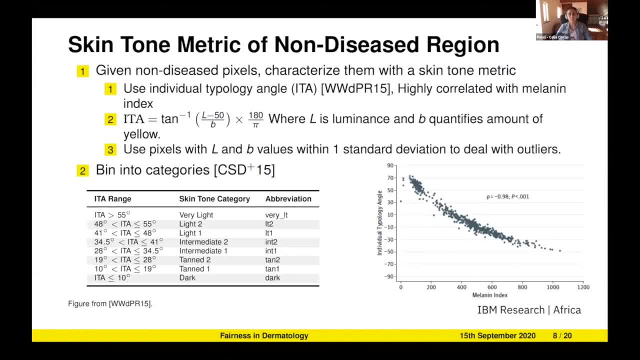 After we have our non-disease region of pixels, we need to characterize them with a skin tone metric. Particularly, we use individual topology angle that is highly correlated with melanin index, as you can see in the bottom scatter plot to the right, ATA is an angle metric. so we need to move from pixel information, transform it to another. 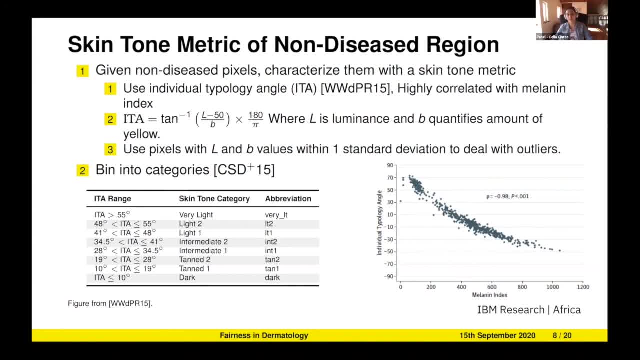 color space and extract luminance information, a bead that quantifies amount of yellow in that pixel. We transform these to an angle and after we have these ATA values, we can bin them into ranges. Previous work used five different categories to bin these ATA values, but we extended to 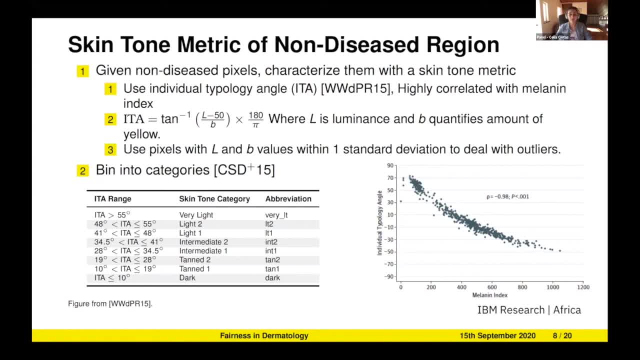 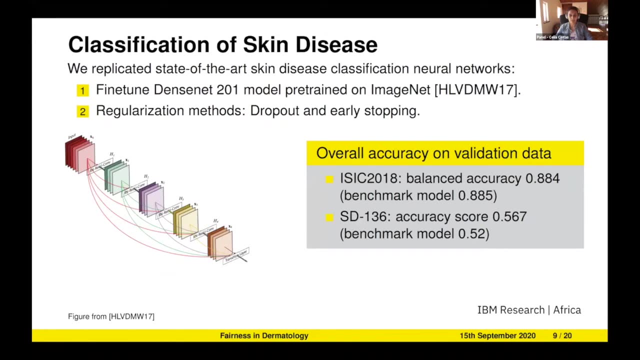 eight to have a more fine granularity of different skin tones. As you can see, lower ATA values go to tanned and darker skin and higher ATA values go to lighter skins. So now we have our skin tone information. Now we want to see if the skin disease classification 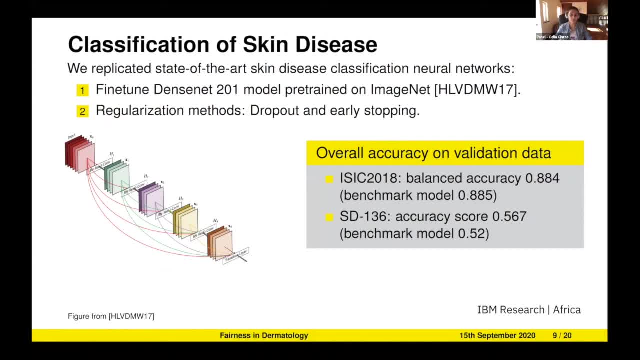 model performs equally across all the skin tone spectrum. For this we replicated state-of-the-art models Particularly. here we are looking at DenseNet that we use for a pre-trained model on ImageNet and basic regularization methods such as dropout and early study. You can see that across both datasets we have 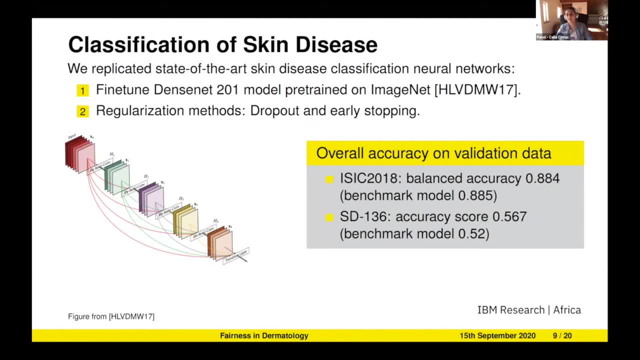 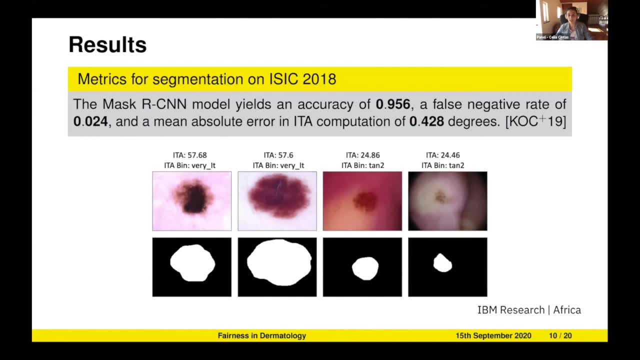 similar accuracy to the ones in leaderboards or reported in other papers. Let's look first at results on segmentation on ICIC 2018.. Here we can see a high accuracy and a low mean absolute error ATA computation. What this means is: how good is our method? 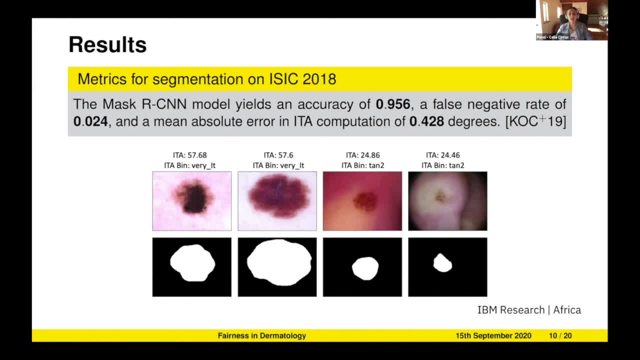 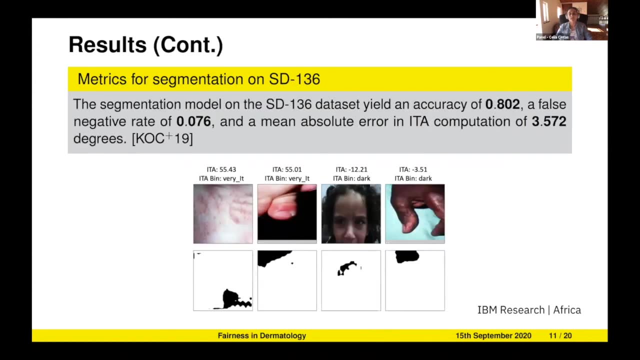 to detect which pixels belong to a non-disease skin area against the other one. This is a good example of how well we can compute or estimate the skin tone based on these pixels. For the second dataset, we can see that our accuracy goes a little bit low and our mean. 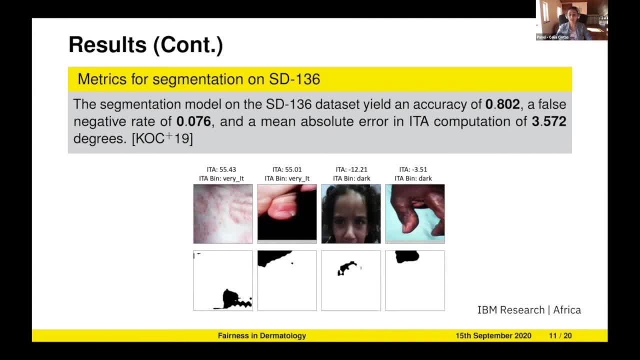 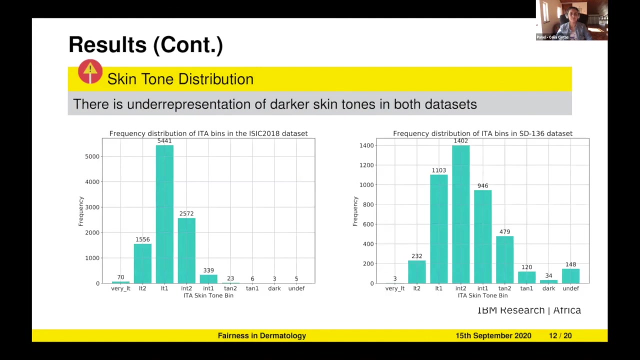 absolute errors for ATA computations go high. Some explanations are that this dataset doesn't have any standardized way to collect data. We will have different body parts here and we can see how the accuracy is different between the two sets of the two, For the third and the fourth datasets. a very good reason is that the accuracy according 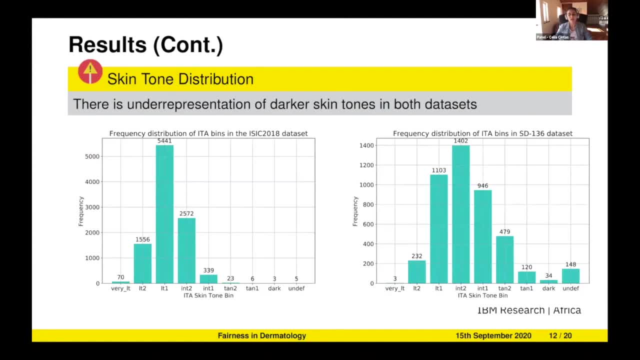 to the deterministic data set is higher than the accuracy of the other two. Perhaps the accuracy of the other two is a little bit higher For the final set we have a high accuracy. look, that looks like the average deviation from the average bit And we can see how good is our accuracy. We can see that the accuracy. 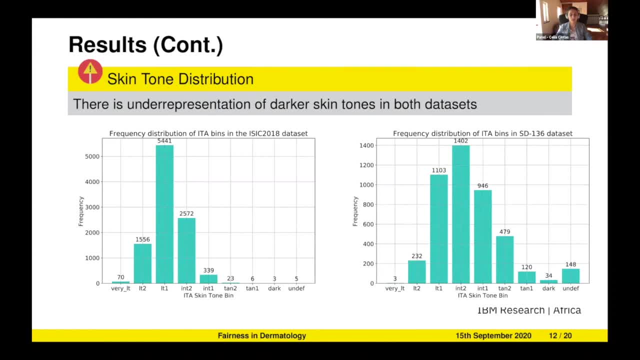 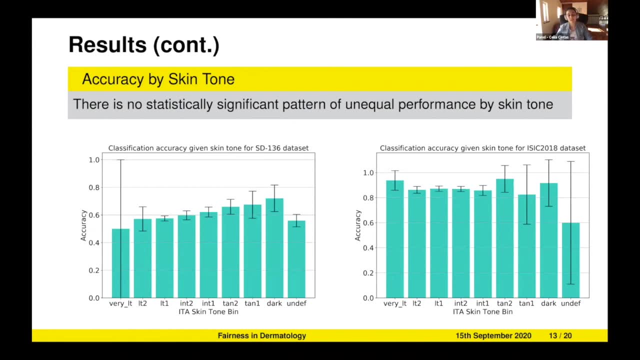 of the filter is higher than the accuracy of the other two. As you can see, we are not on these ranges of the skin tones, but the bias in the data sets doesn't seem to affect the classification result for each of the skin tones, but the caveat to. 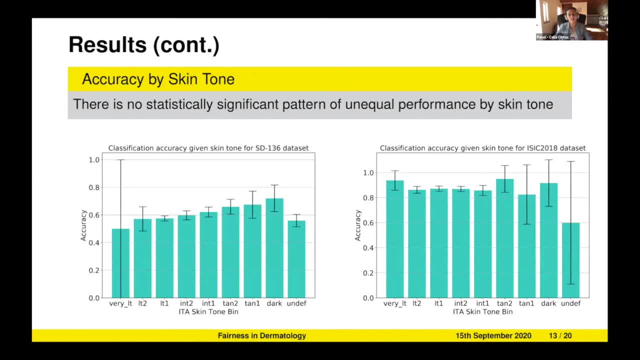 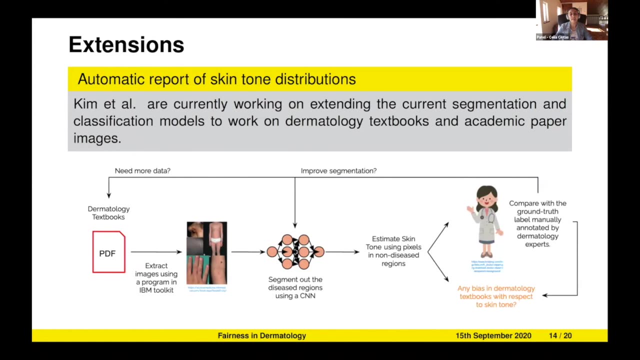 these results is a very small sample size for darker skin tones, so further research should be done, augmentating this part of the data set and rerunning some experiments, some extensions. that currently Hanna, one of our member, is working on is: how can we use the same framework but to dermatology textbooks? 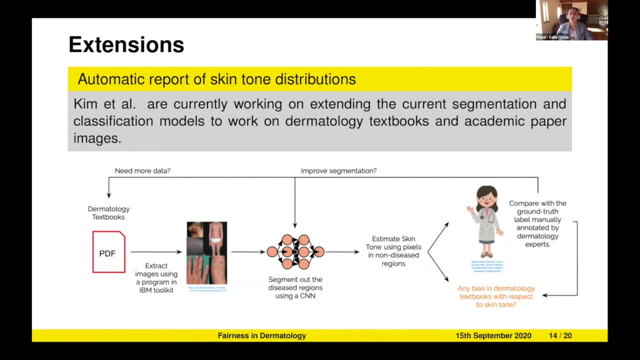 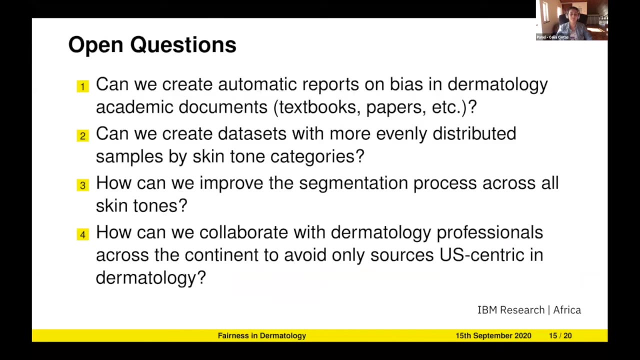 so currently our framework runs for dermatology data sets, but we want to expand these to textbooks or academic papers so professionals can have information on the representation distribution of examples in these documents. we still have a lot of work going on. we are wondering how can we create? 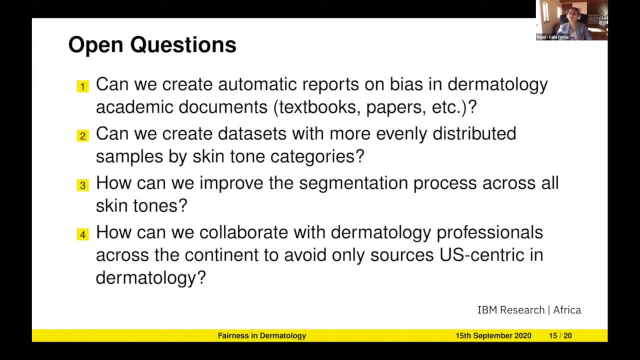 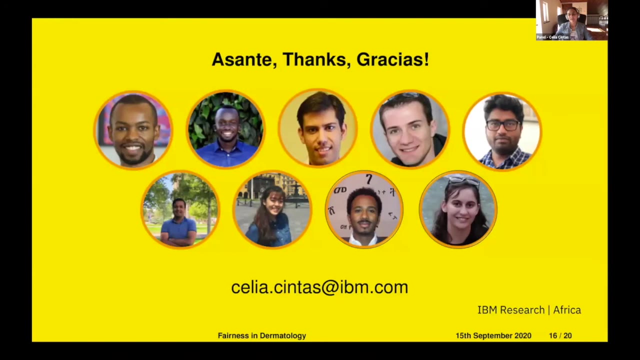 data sets with more heavily distributed sample cycles and skin tone categories. how can we improve the segmentation process in the wild images such as textbooks or papers? and how can we collaborate with dermatology professionals here in the continent to avoid only sources for US centric in dermatology? here are all my colleagues that are: 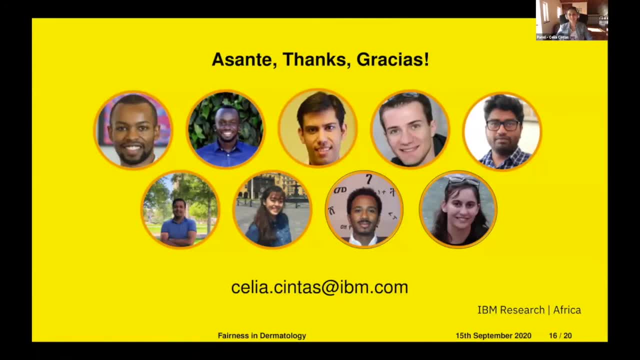 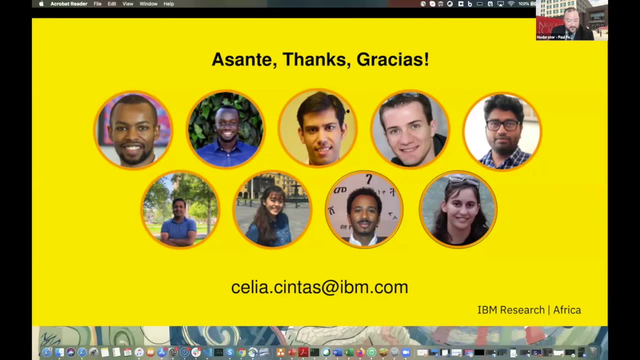 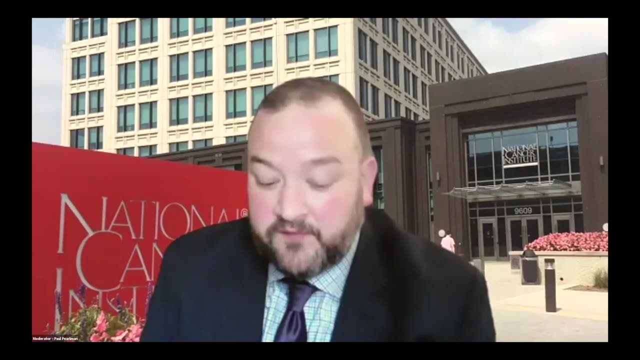 working on fairness and different health care applications. thank you so much for your time. thank you, Celia. while dr Milner is bringing his slides up, I'll go ahead and introduce him as well. dr Dan Milner is the chief medical officer for the American Society for clinical pathology, based in Chicago and works. 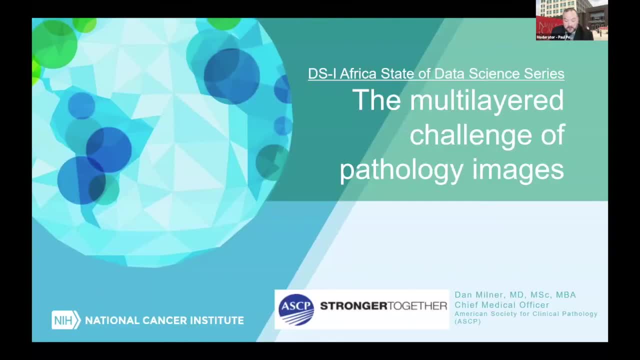 with more than 20 countries on pathology, capacity building, including telepathology, and personnel. yeah, so this morning, thank you so much to my fellow speakers who have set a wonderful stage for what I'm going to discuss, and what I'd like to do is dive really deep into pathology. very briefly, because this is a 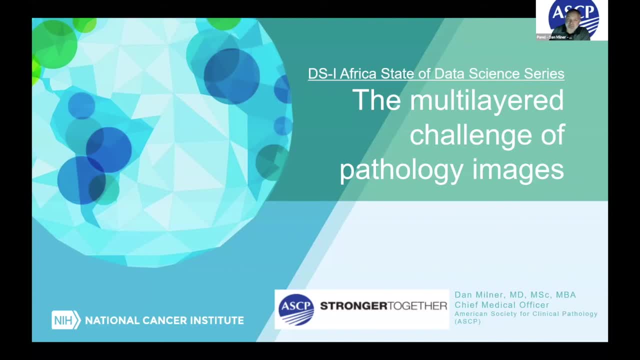 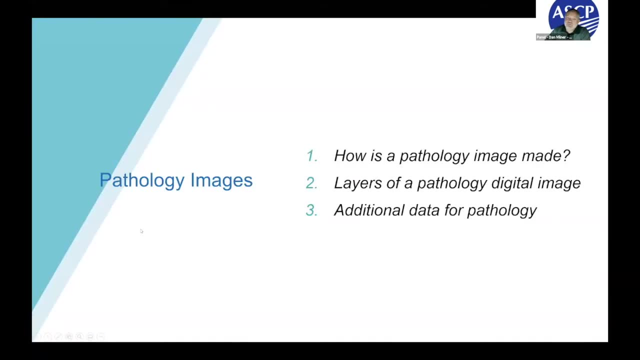 rich source of images. someone in the Q&A has already asked or pointed out that, so I just wanted to go into that in a little bit more detail. so to begin, I just want to talk about pathology images, and first, how is a pathology image made, which I think is important for everyone in the audience to understand. the 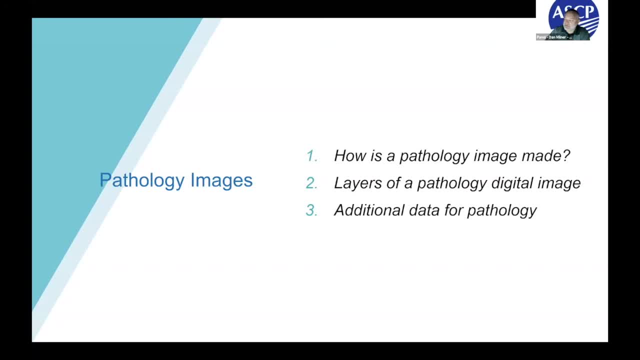 complexity of that process before we actually get to that image. then talk about the layers of a pathology digital image from the the lowest level resolution to the highest level, and what that means for research implications. and then, and lastly, talk about additional data, which has been touched on briefly. 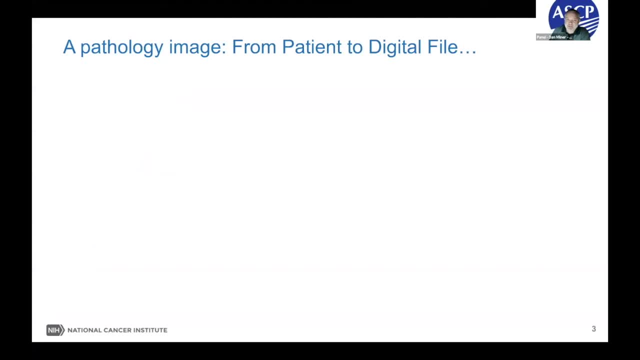 by my fellow speakers. so let's talk about a pathology image from a patient to a data file. so, for those of you who are familiar with pathology, this will be a little bit of a review. for those of you who are familiar with pathology, this will be a little bit of a review. for those of you who are 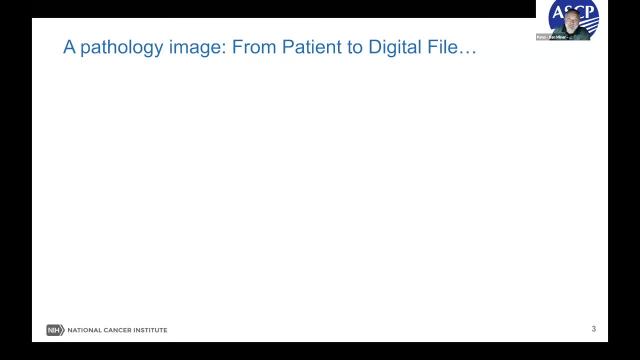 not keep in mind that there are three main sources of, or three main types of samples that you may use in Africa for pathology. those are cytology, which is the study of cells, surgical pathology, which is the removal of tissue from a live person to make a diagnosis of cancer or an infectious disease, and then autopsy. 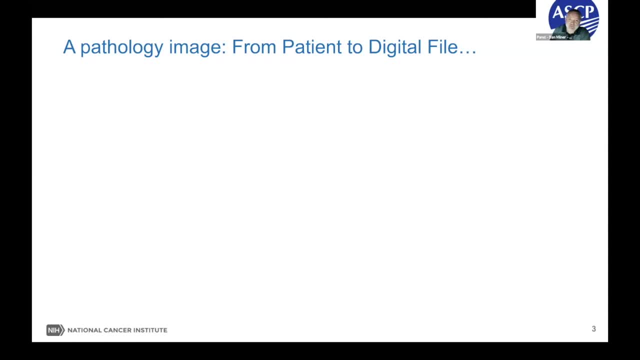 pathology, where you remove tissues from a dead patient in order to make an anatomic diagnosis after death. and that whole process- here illustrated by an example of taking a sample from a breast tumor, is not dependent on pathology. it's dependent on the clinicians: the proper way that the 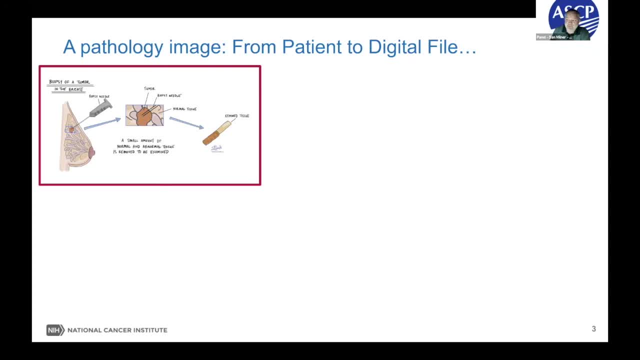 sample is taken, handled, processed, labeled and fixed before it is sent to the pathology lab can have massive impacts on the quality of the image that's produced at the end, and so this is a component of research or a program that has to be well understood and documented once that sample is collected. 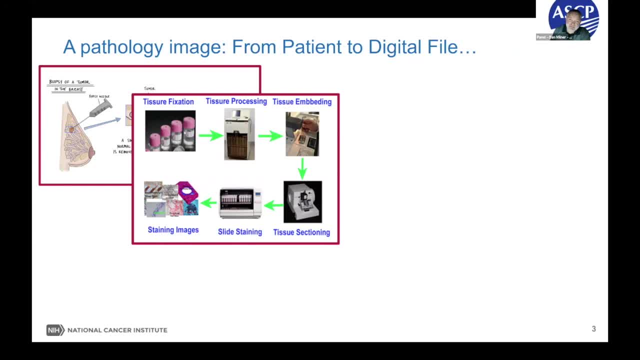 and sent to the laboratory. it's in a fixative which has to be of a certain type. it's put on a tissue processing system. it's then embedded in paraffin wax. that paraffin wax block is then cut with a razor to produce a slide. 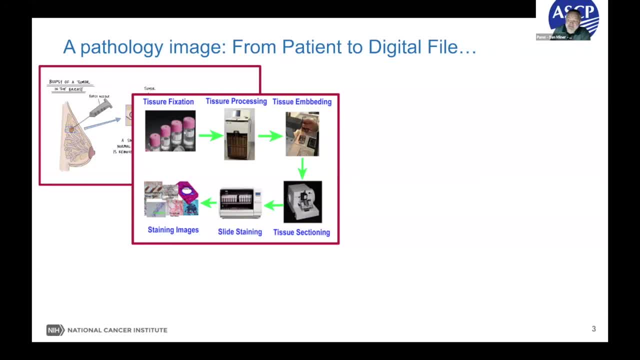 that slide is then stained using a variety of different staining techniques and then you have a stained image and this is the classic histology slide or even cytology slide that a pathologist would look at under the microscope and read. and, as you can see, there's already a lot of steps in this process that can 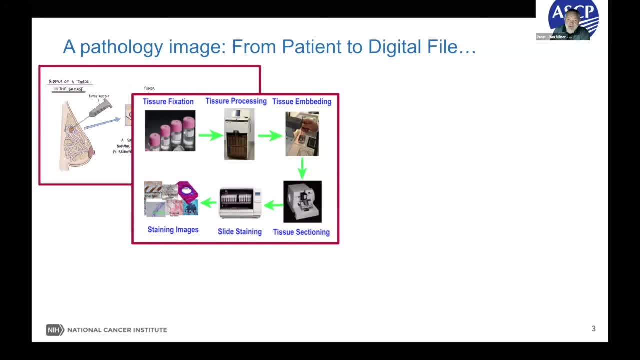 go wrong. if fixation is wrong, if the tissue processor isn't functioning properly, if the tissue embedding isn't done with highest quality, these images are not going to be ideal. now we have our glass slide, and we need to. we need to scan it to create a whole slide image or a digital image that we can then analyze with a computer. 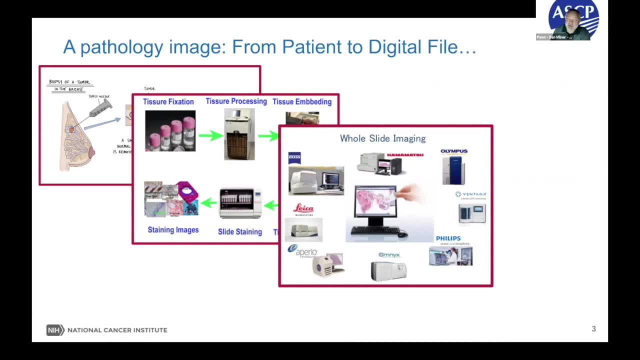 well at this point we have lots of options. there's not just one way to scan a slide. there are at least a dozen different companies that make whole slide imaging systems. they use different background processes. some of them, like Philips, use Blu-ray technology. most of them use basically a microscope inside. 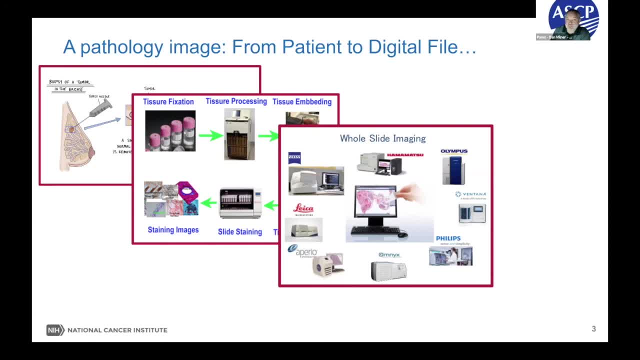 the system that scans either by moving the slide or moving the microscope objectives, and they can scan at different resolutions. they can scan at 20 X or 40 X and have optical zoom up to 80 X or 100 X, but all of that is variable and needs to be understood before you try to use this for research. 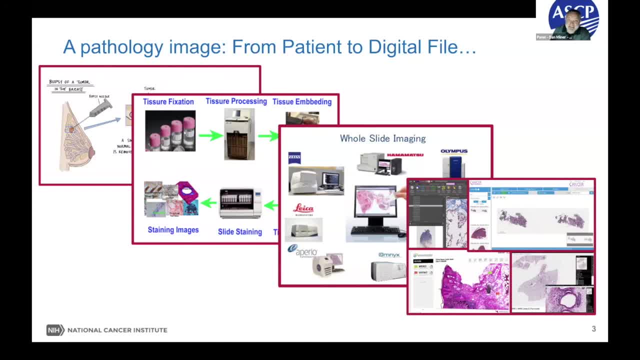 and then, lastly, once you have scanned that image using that system, you now have have to look at that image or study that image, And there are a variety of viewers. at that point, Each company that makes a scanner will have a different software viewer. 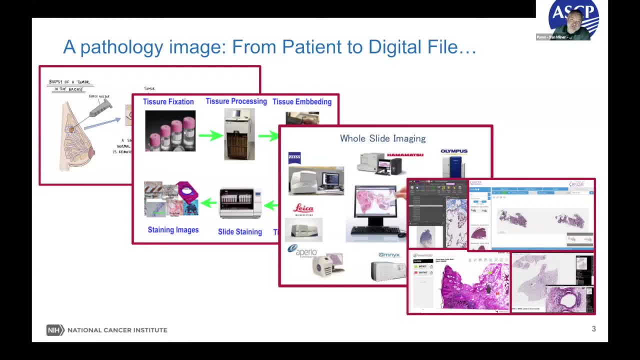 There are some agnostic viewers that are available as open source software, And all of those use different file formats, They process the image slightly differently when they open it, And so those are other aspects that need to be understood. So just to recap this, as we go from the patient, 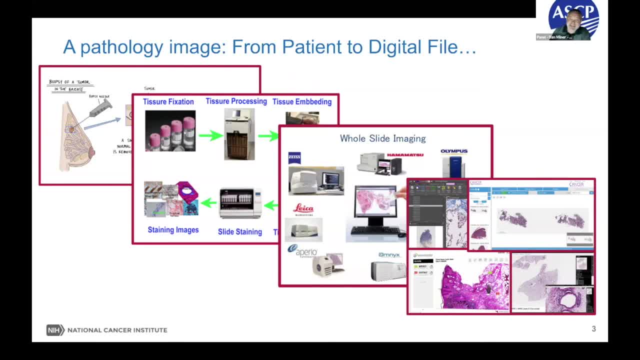 to a digital file of a pathology image that we want to analyze in our research. there are all along the way, steps around quality, around assurance, et cetera, that you want to make sure you're keeping up with and accounting for in order to make sure. 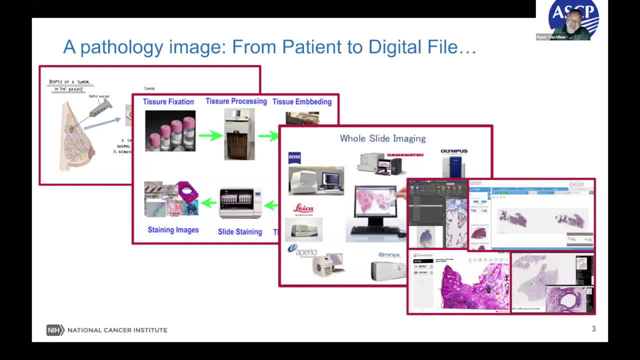 that that final image you're looking at is of high quality, And this is not something you can take for granted. If I had the time, I could talk to you for hours about the challenges of pathology in Africa. This is what ASCP works on. 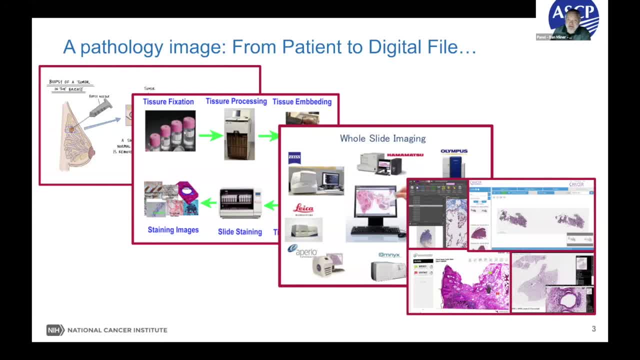 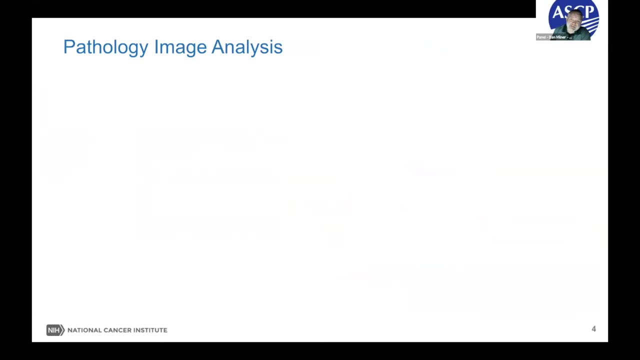 We work with multiple laboratories to help improve their quality, to provide equipment, to provide immunistic chemistry, And the goal is to produce high quality images for diagnosis, but also high quality images for research. What about pathology image analysis? Now, my colleagues have shown you radiology. 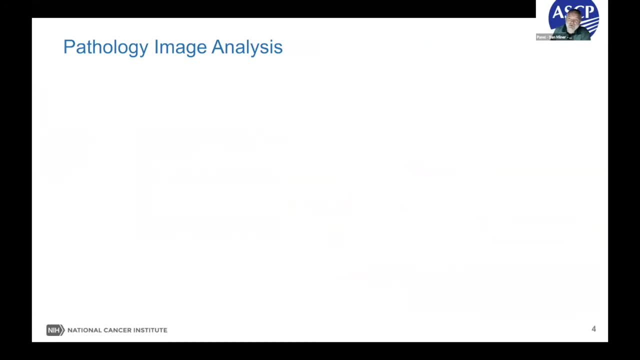 gross image of the cervix as well as skin, And those are very complex, as you could see. the process that they were using And pathology is slightly more complicated than all of them for a couple of reasons. So if we think about the image that I'm showing you here, 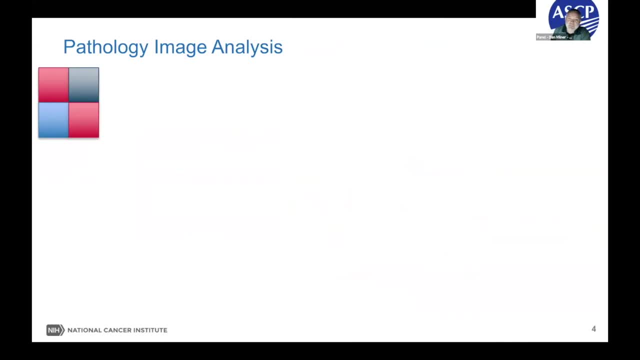 of four boxes- two red, one blue and one black- and we want to teach a computer how to figure out what those are, the orientation, et cetera. it wouldn't be that complicated, And this is very similar to trying to understand. 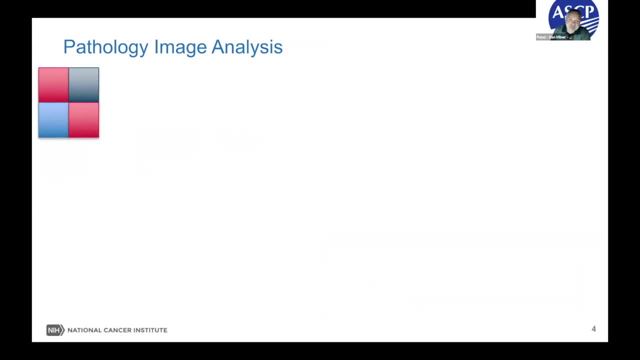 a radiological image which is in black and white, or possibly even a skin image which is almost two-dimensional, the way that you look at it. But with pathology we have all those different colors, but we also have layers: A histology slide or even a cytology slide. 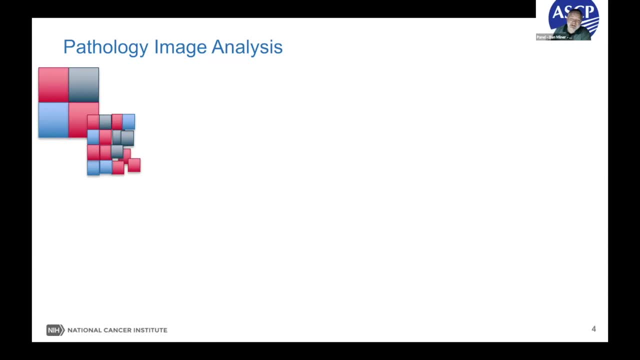 can be many microns thick, And so from a given image, the camera can actually take multiple layers and have multiple slices or Z stacks that we have to look at And in research you may need to account for that. Then, when we finally look at our image, 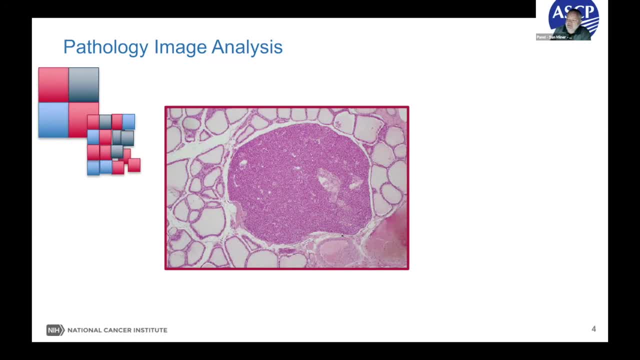 for example here this is an image within the thyroid of a parathyroid. something very simple. You can see at this low power that the surrounding tissue is different and the tissue in the middle is unique or is of one type. And for a pathologist, they look at this slide. 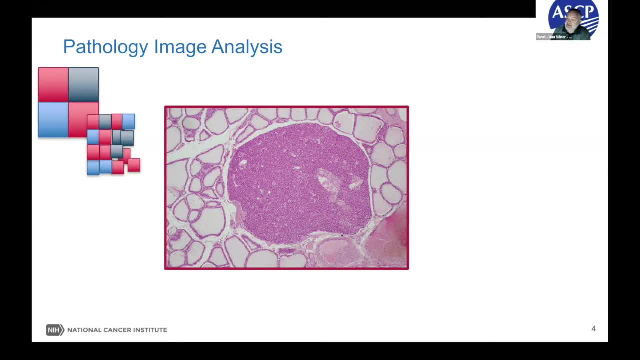 and instantly think, oh, that's thyroid with a little parathyroid in it. But for a computer it first starts and says, oh, there's a light area, there's a dark area, and then it does pattern recognition to figure out where it is. 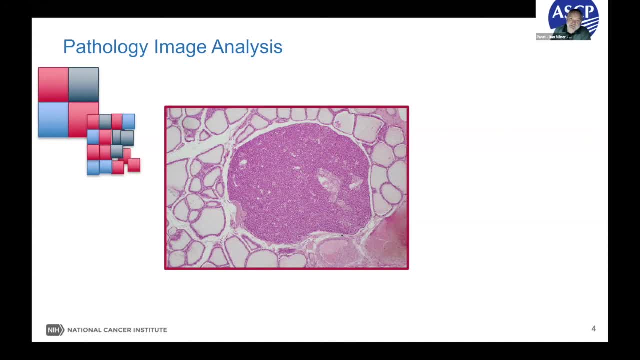 And then it can finally say this is likely a structure within a thyroid gland And looking at the color of the nuclei, et cetera, it can determine using AI or comparative metrics that this is likely a parathyroid or some other structure. 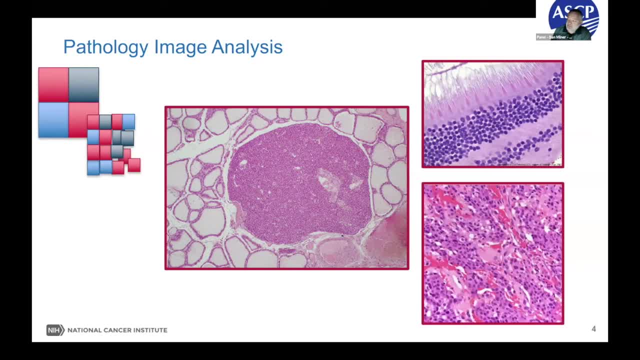 But this is at a low power. If we now zoom in to a higher power, as in these two images, these are from completely different cases. you can see that in the top image there's a lot of structure. This is a very structured picture. 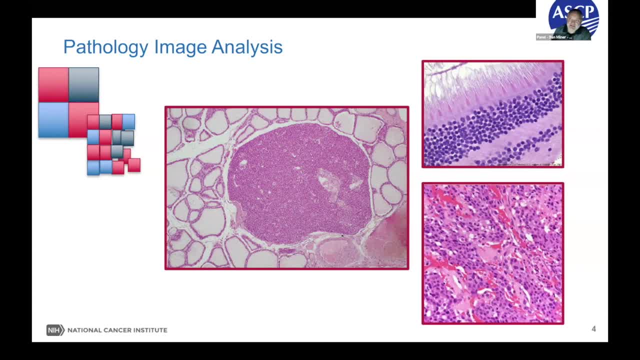 It's got orientation. It looks very unique and almost like something that anyone should be able to recognize with a little bit of training, And this is, in fact, part of the retina of an eye, And so you can see the rods and cones. 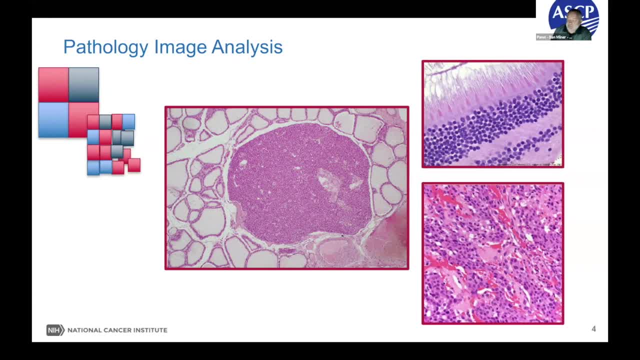 and different parts of the eye, But the lower image of histology is just from a random part of a tumor And what you notice is that there are some blood vessels in there. That's the red stuff, There's some purple nuclei, There's some pink. 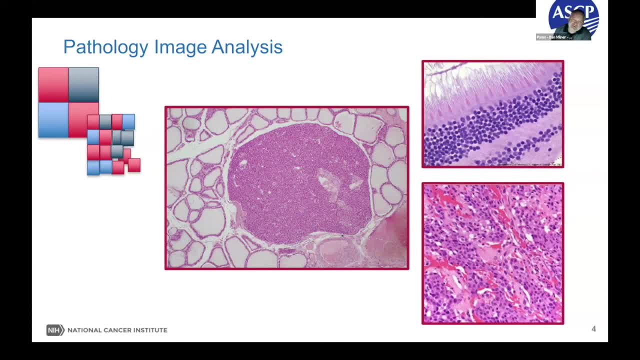 There's some black, There's some white, There's some blue, And this is actually very interesting. And I think what's really interesting is that there's a lot, of, a lot of information that we see in the material, but it's completely disorganized. 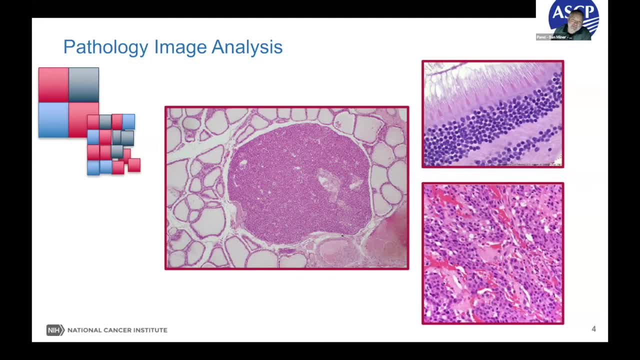 We don't have that structure that we see above, And it's very high power. This could come from the slide in the middle, but it's such a high power that we don't have a lot of context around it. And so when a computer or an AI algorithm 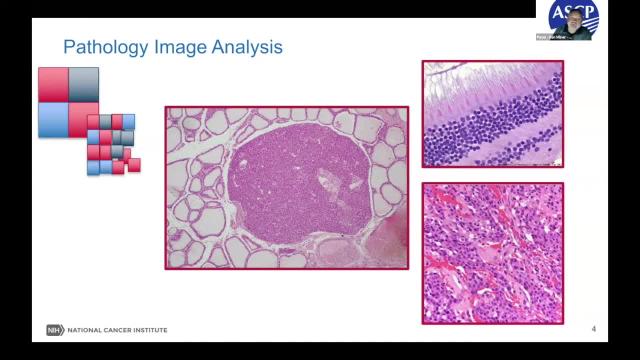 is trying to learn. it can learn at low power, but does it have that same learning using the same learning? To recap that if we just wanted to have our computer or our AI algorithm recognize that this was a parathyroid within thyroid tissue, you can imagine that it's not as complicated. 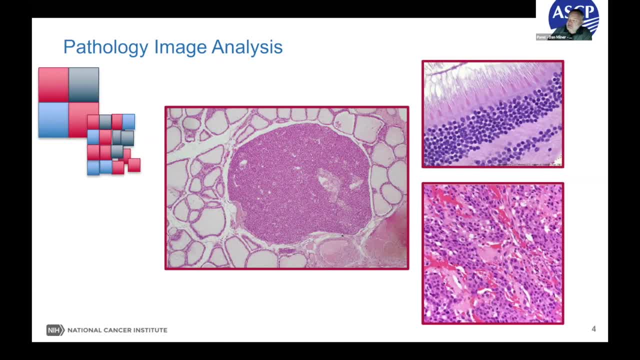 as trying to teach it to recognize, for example, the orientation of the rods and cones in the retina, or even to tell you what kind of tumor that is on the lower left or, I'm sorry, the lower right, because of the lack of orientation, the lack of structure. 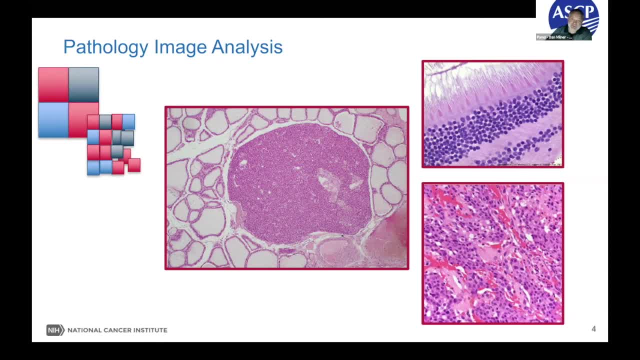 The AI really needs to study those cells, to study those nuclei and even look for details that we may not have in what my colleagues have been calling the ground truth. That is, a pathologist may look at that slide and say, oh, that's a X tumor and I recognize. 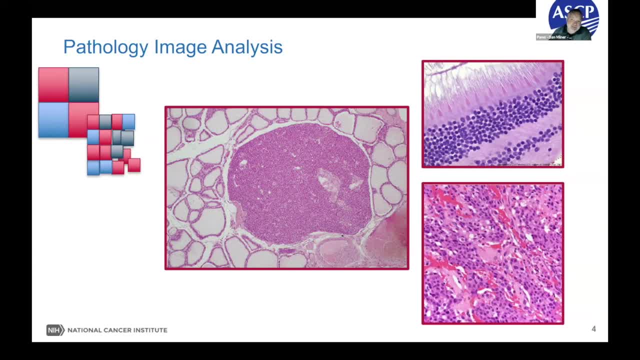 that from morphology. but they may be incorporating all the information about the patient- what the low power view looked like, what the high power view looked like- but AI is only looking at this one image and has to be able to also integrate that data. 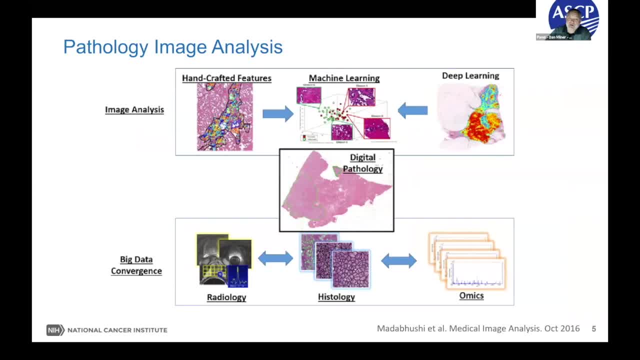 And then, lastly, there's all of the additional data that goes along with the pathology. So we've got that, We've got digital histology in the middle, which I've just walked you through, but then there's all the ways you can analyze it. 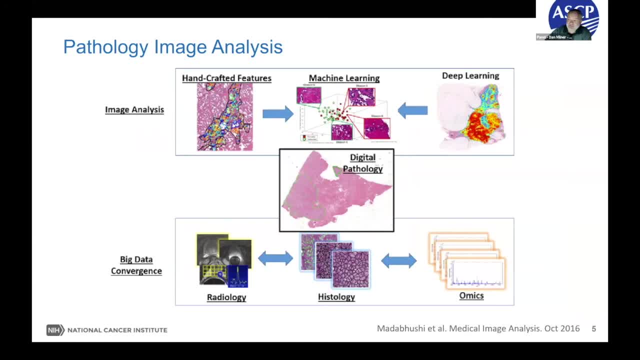 You can do handcrafted or hand-annotated features, where a pathologist or a technician goes in and marks off different areas. You can use machine learning where you, as Celia was describing, where you feed the machine thousands and thousands of images which have already been annotated and then it learns. 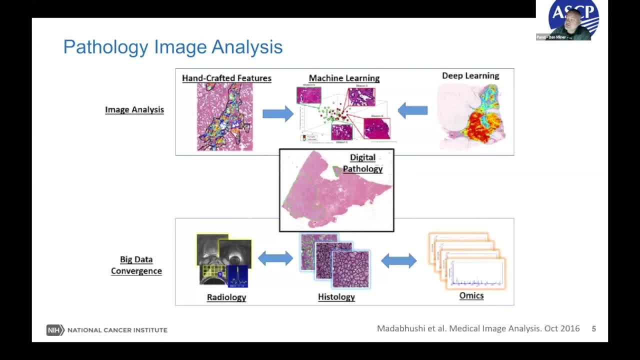 to interpret new images that it's never seen before. And then you can do deep learning, or neural networks, as Samir was talking about, where you teach it to analyze, And then you can understand the interactions of cells on a slide using multiple different 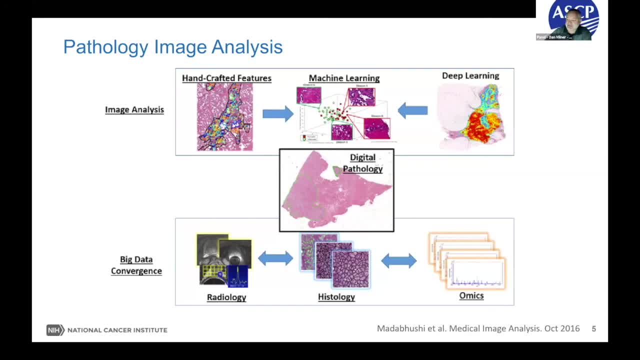 layers of information, for example, different stains or different color techniques, And then, as we were Michael was talking about, you may have radiology data that you need to correlate back with histology, And he was referring to histology as an example of ground truth to base on radiology. but 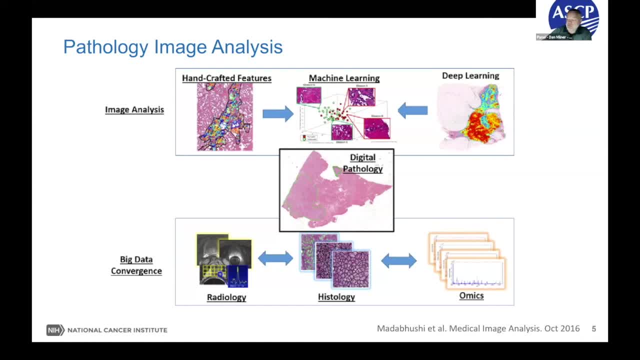 understand that histology also needs a ground, truth or a basis to understand exactly what's going on there. And then there's all the omics, data, transcriptomics, any other Kind of proteomic data, et cetera, that has to be related back to that histology. 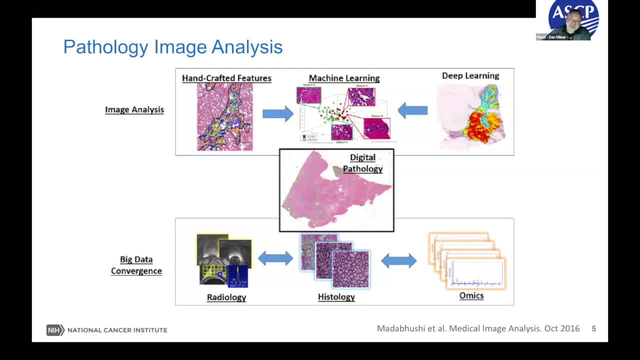 So there's two aspects of that. One is that histology must be high quality and absolutely perfect for all of these things to be integrated correctly to give you the best result, But then when it is really exactly what you want it to need, or what you want or need it. 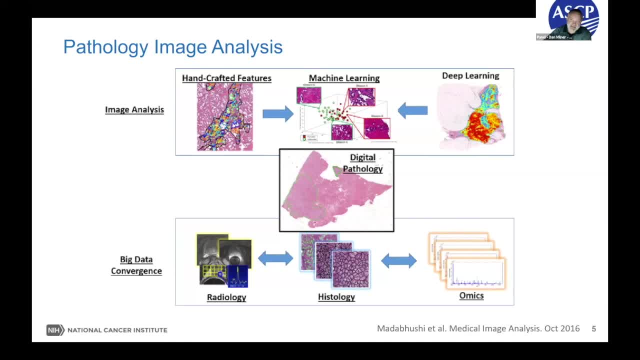 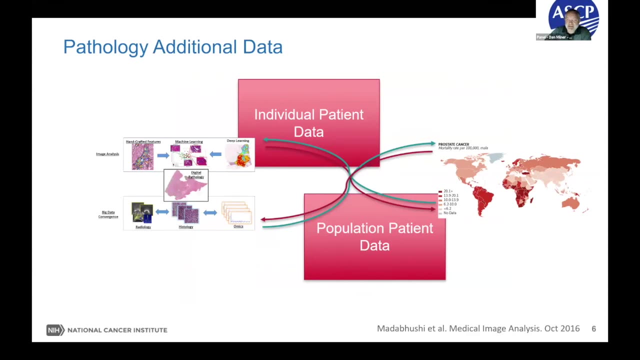 to be. it needs to be integrated correctly to all of this data, using annotation and tags and case tracking, so that your omics data on RNA expression is matched to the proper set of histology Images. and then, when we think about all of this, there are two ways that this data can. 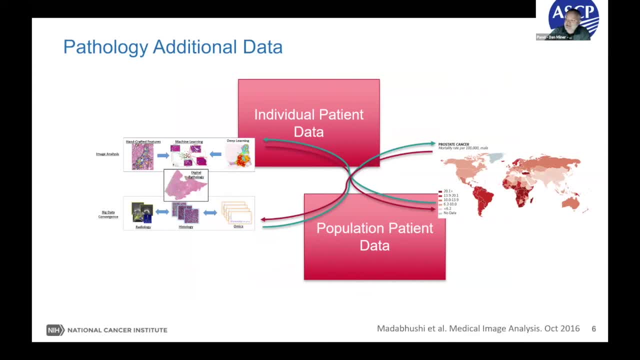 sort of come together, especially in data science or big data projects. We can think about individual patient data where we have, you know, 10,000 patients from multiple countries that all have a same cancer or similar cancer or infection, And we're feeding all the data about those patients into a database. 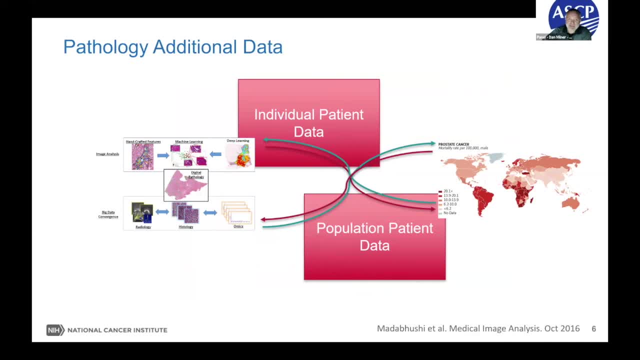 And that's sort of creating working models or AI models for how to do things. But then there's also population, patient data, the demographics of the population, epidemiology, cancer registries, et cetera, which may be anonymous data. It may be more about a region or a population than it is about individual patients. 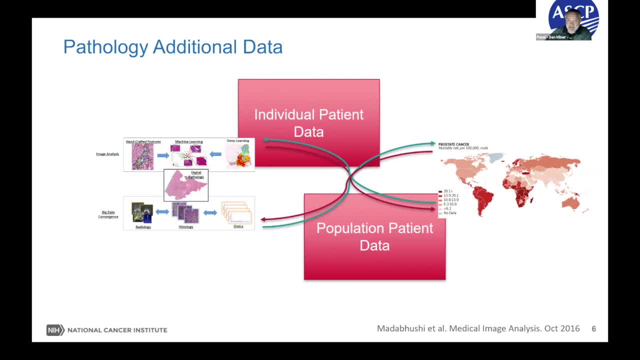 And that's important, because, for those of you that are thinking about projects that are going to have impacts for policy, or how you are going to inform the government of spending money, et cetera, you want to think about population, patient data, because you're trying to do what's. 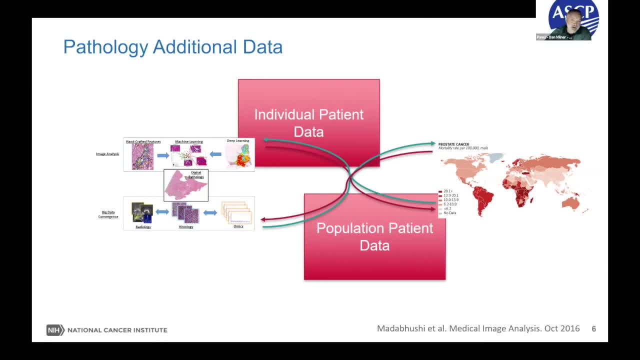 best for the population. But if you're in a program or you're doing a clinical trial or you're trying to treat patients, you're going to look at individual data to say what are we learning from this system, to go back and help that one patient as we move forward. 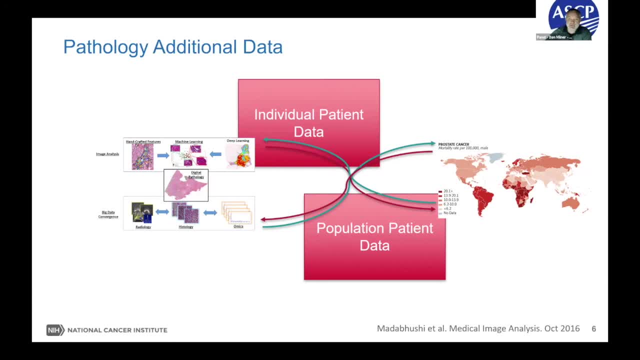 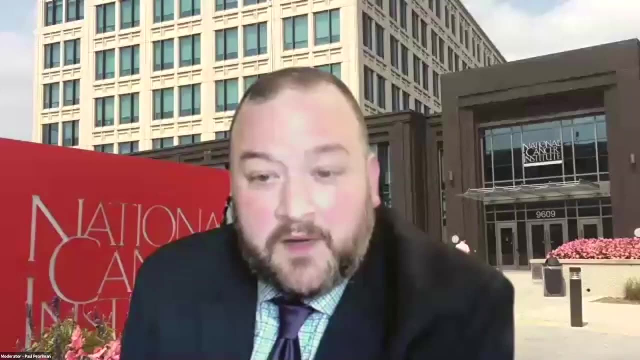 And that uses very similar techniques and integrates the data in a similar way, but it's just a different level of analysis and a different level of understanding. So I think with that I will close and turn it back over to Paul. Great Thanks, Diane. 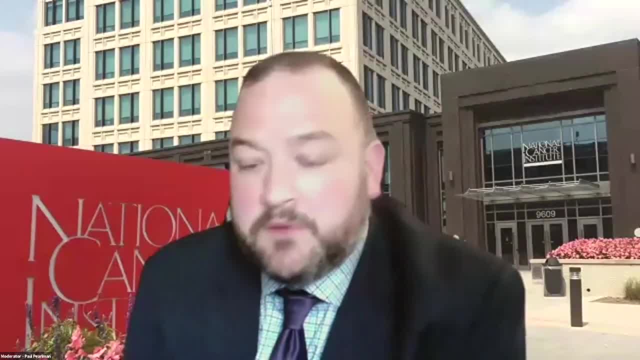 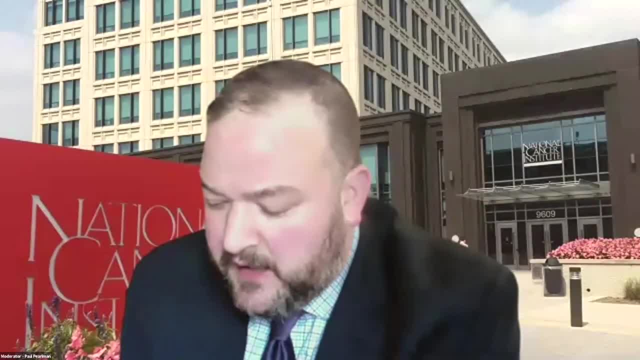 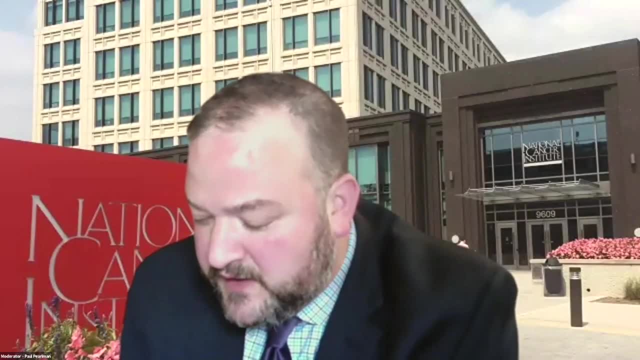 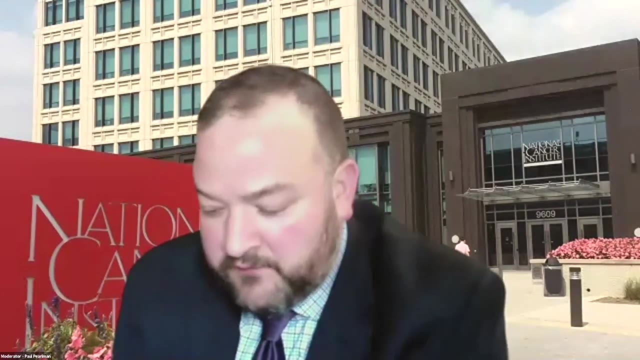 Thank you, Thank you, Thank you. I'm going to go ahead and kick it off with maybe a couple questions that were hinted in the talks, So this one is initially for Professor Kouya, but I think was relevant to everyone. How should we think about applying machine learning and artificial intelligence when? 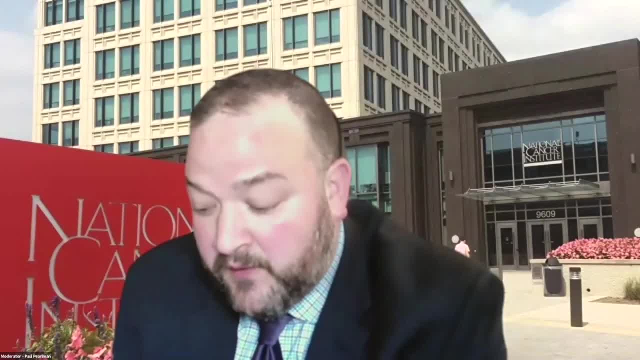 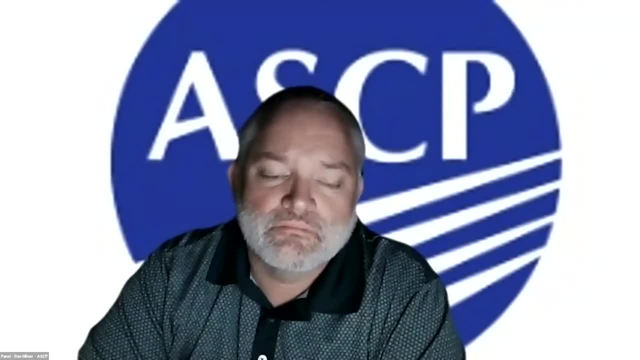 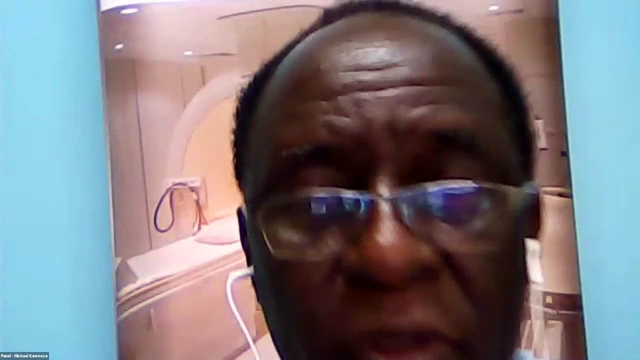 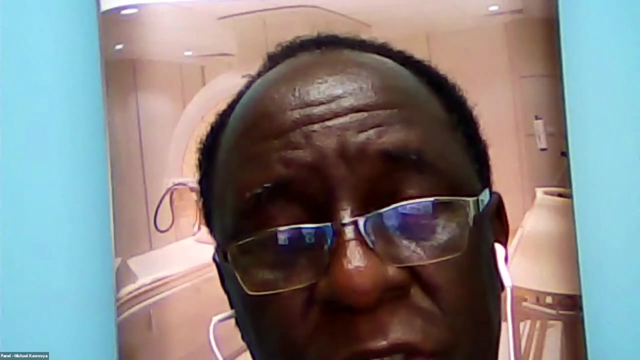 our data sets may be small or, as Professor Kouya suggested, some of our data sets have poor image quality. Thank you, Paul, for that. When our data sets are of poor image quality, it becomes difficult for us to apply machine learning, because it would be difficult to train the algorithm with images. 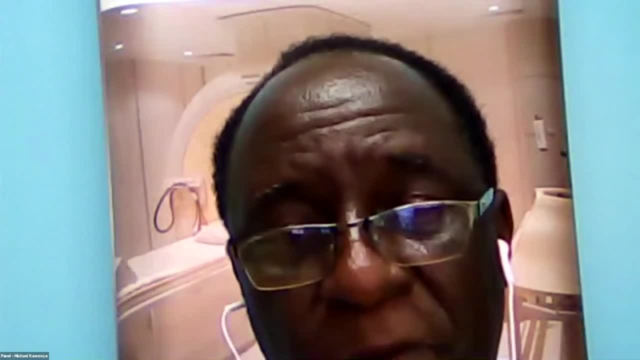 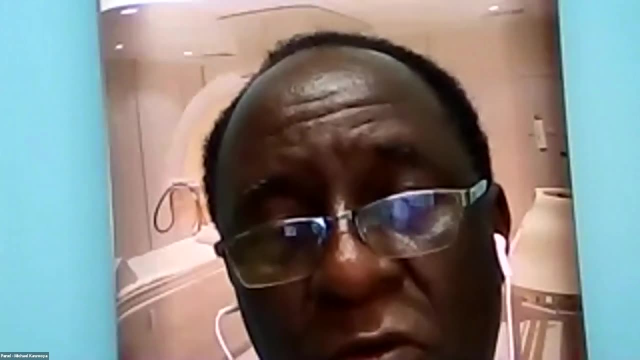 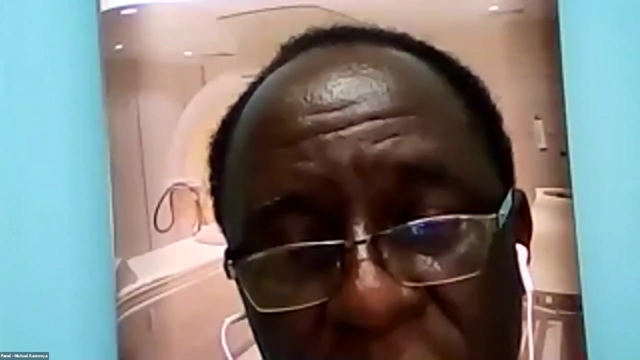 of poor images, of poor quality, and so I think it's very important that, even as we begin, we must ensure that our quality is uniform and that the method we are using is also standard and homogenized. That's all that I can say, because I mean. 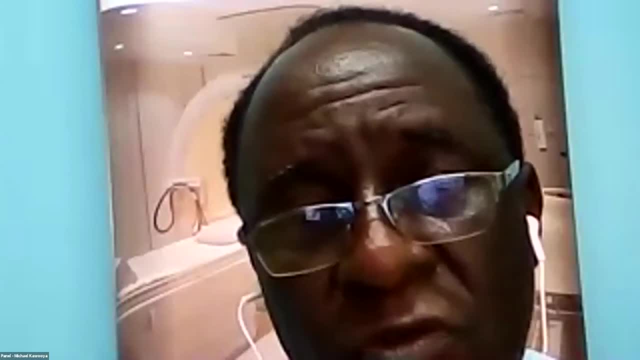 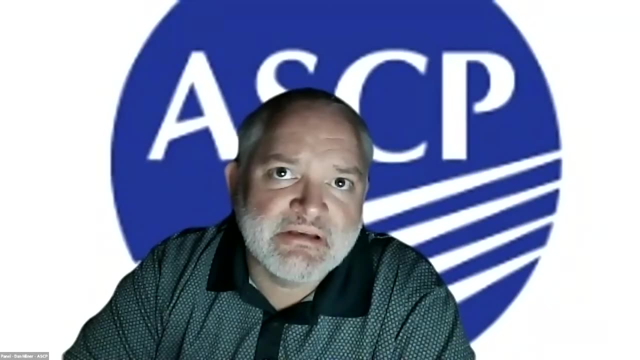 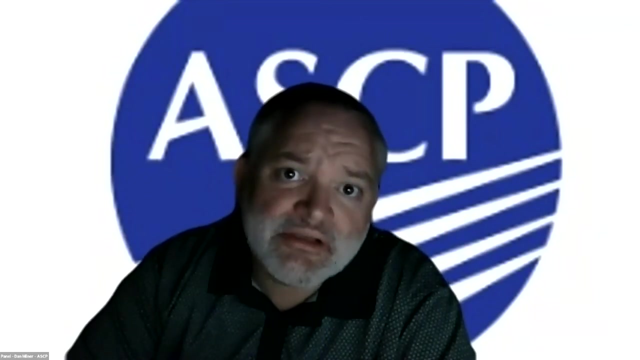 the algorithm will just get confused with images of poor quality, And I can also comment on that, Paul. I think one of the things that it's really important for our audience to understand is the state of the disease they might be wanting to work on. So, if you want to do a project on the data, 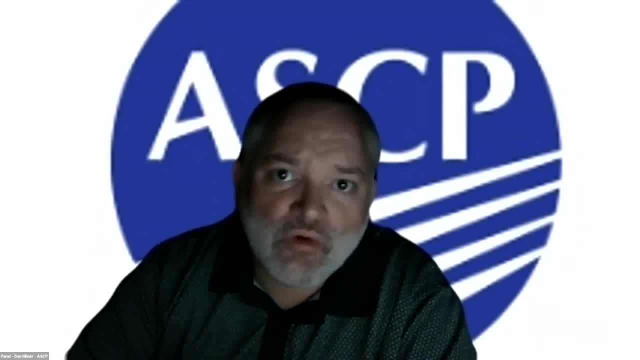 science of tuberculosis or HIV or malaria or breast cancer. one country, or even one center may have more than enough cases to produce a big data set, especially if you think about sequencing or other omics that are going to go with it. But when you start thinking about 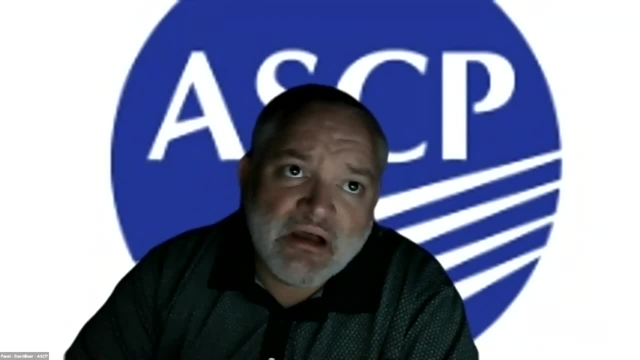 the data science of tuberculosis or HIV or malaria or breast cancer one country, or even one that you're thinking about, producing a big data set is probably not as good, And we'll see the same thing if we think about rare cancers, for example, or rare infections, multicenter or even 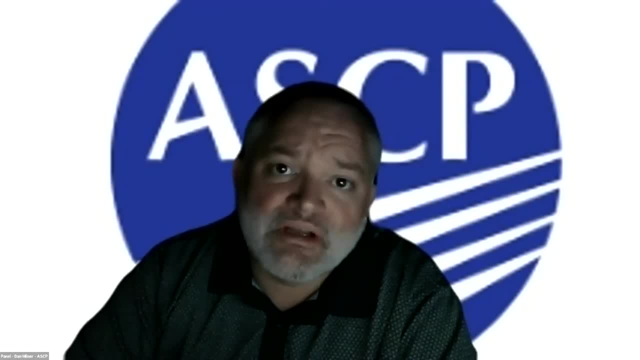 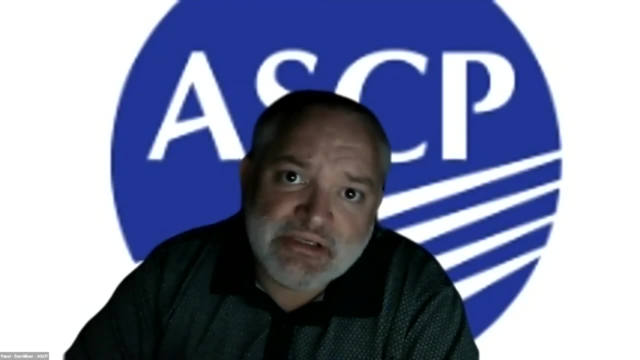 multi-country data sets may be needed in order to have enough images of a given disease in order to actually do that work, And so I think, as you are embarking on what you want to work on or what you're thinking about, consideration of the epidemiology of that disease is really crucial for 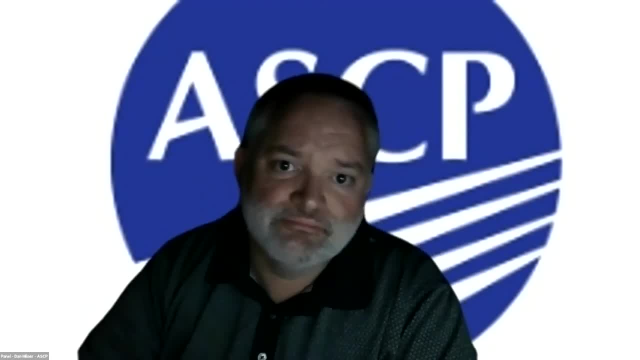 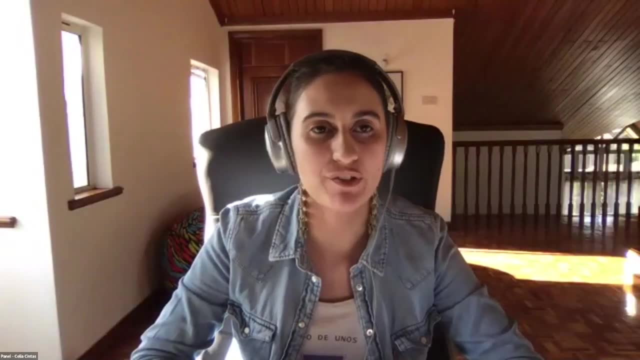 sample size as well as the amount of money that you have for these particular grants. Ana Pereira-O'Callaghan, On the machine learning side, as you saw in this talk, I we use pre trained models. If you're using image based data, you can actually use. 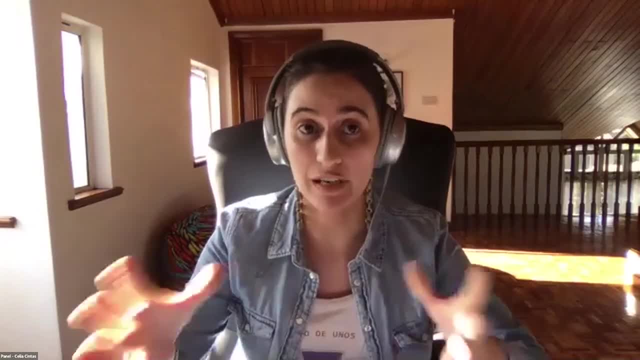 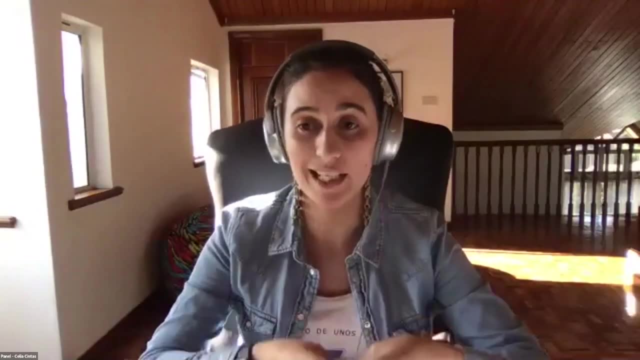 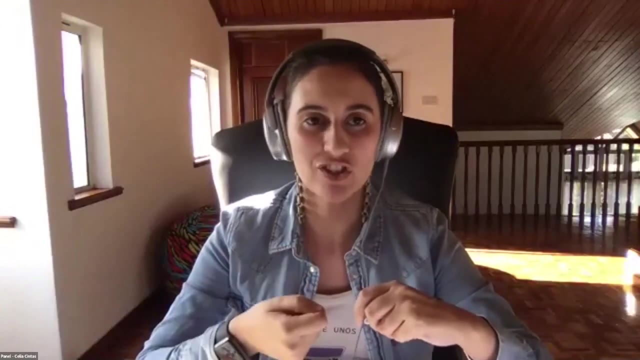 Ana Pereira-O'Callaghan. Training models to based on other data sets more large, and you fine tune to your small data sets, Ana Pereira-O'Callaghan. So this is a technique that works very well on images, because usually these deep neural networks work on the same idea of finding edges or finding features that are common across all images. 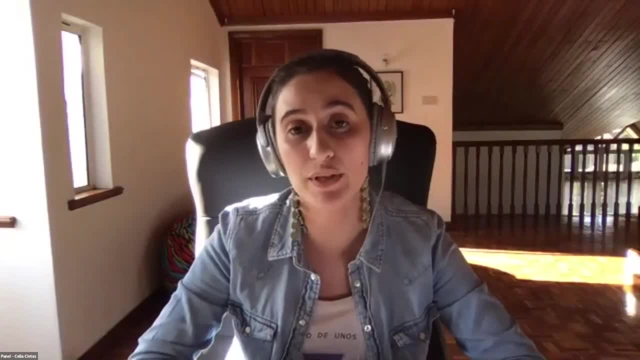 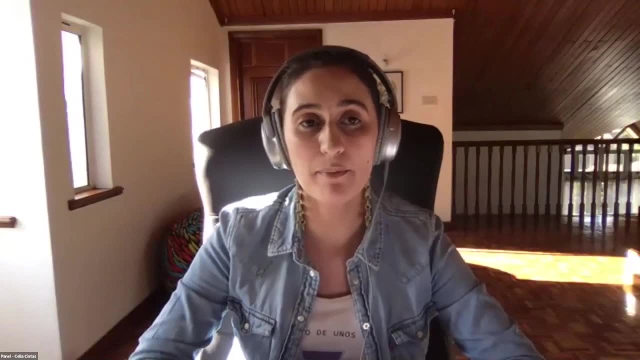 Ana Pereira-O'Callaghan, So you can fine tune your models when you work with a small data sets are, regarding quality, wise. if you have Ana Pereira-O'Callaghan, If you have a much set of flow, quality and high quality samples, This will be an idea. 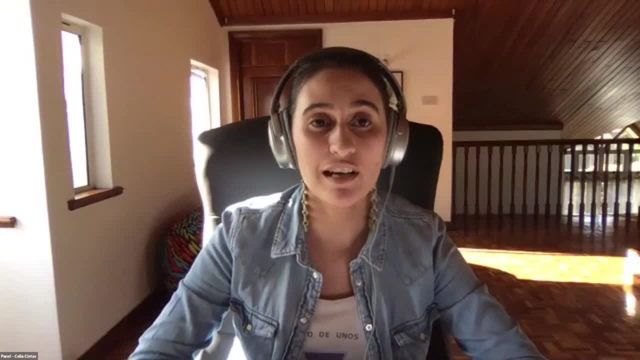 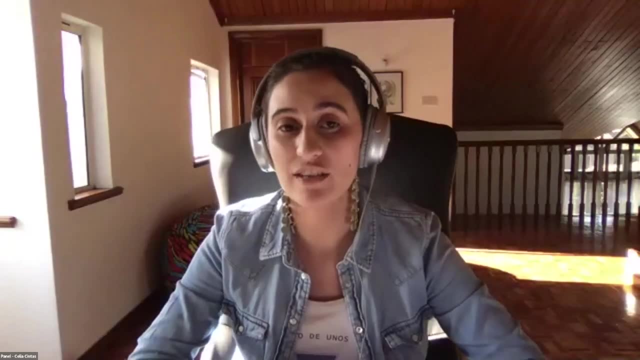 Ana Pereira-O'Callaghan Setting. you can actually train generative models to learn what a high quality image representation looks like. So any low image data set quality can actually be transformer too high, but for these you at least need to have the pair. 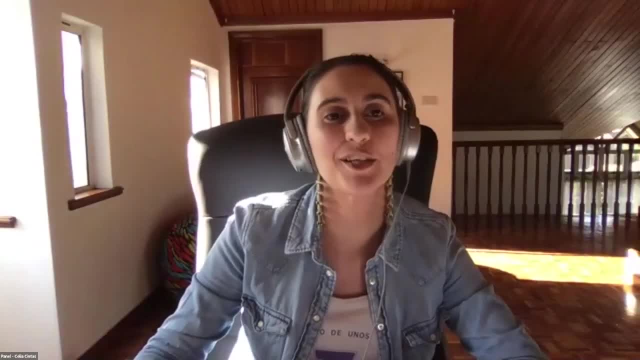 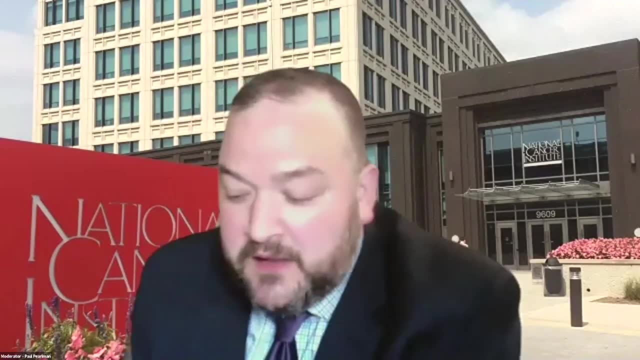 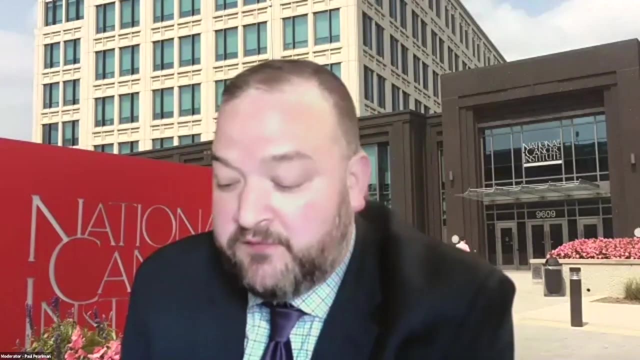 Ana Pereira-O'Callaghan- Of good and high quality. Peter Rushforth- Potentially, another one that we get most technology related panels is Peter Rushforth- You know, Peter Rushforth- As we started to talk about the need to develop sort of new cloud infrastructure and as as people start to think about these grants. 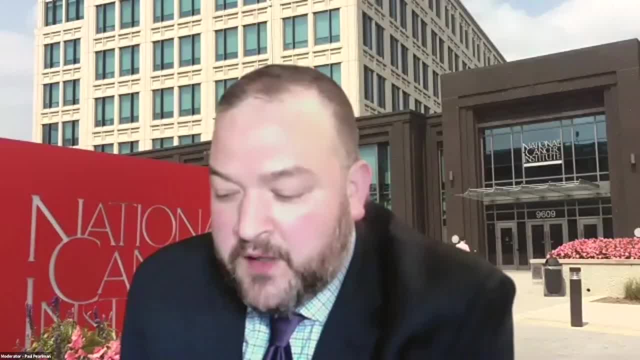 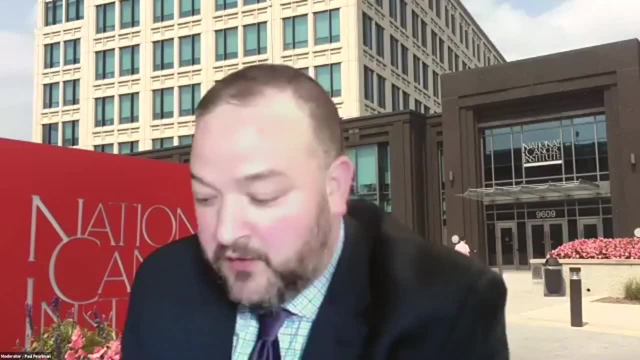 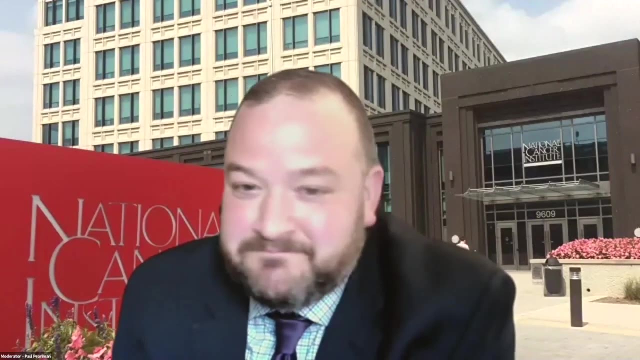 Peter Rushforth- Is: are there what opportunities exist for sort of leapfrogging over some of the fits and starts We've seen and in sort of developing standards and and other issues in terms of generating large data sets? Are there opportunities? to? Peter Rushforth- Learn from our from past mistakes elsewhere. 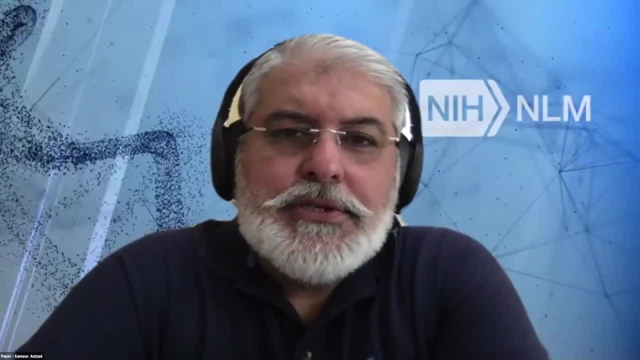 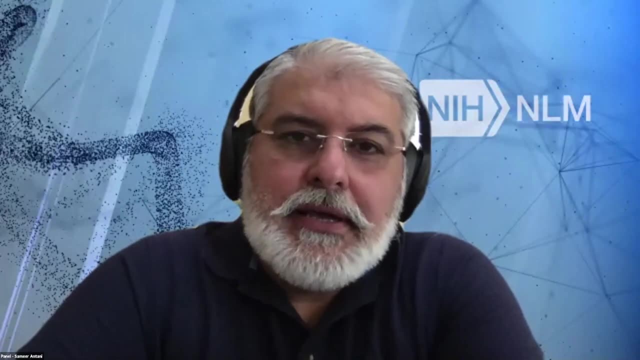 Ana Pereira-O'Callaghan. I'll key off on the word generating data sets. there, Ana Pereira-O'Callaghan, Is that if you are embarking on a new study and you have the opportunity to acquire new data, then establishing protocol- I mean, I'm speaking, not 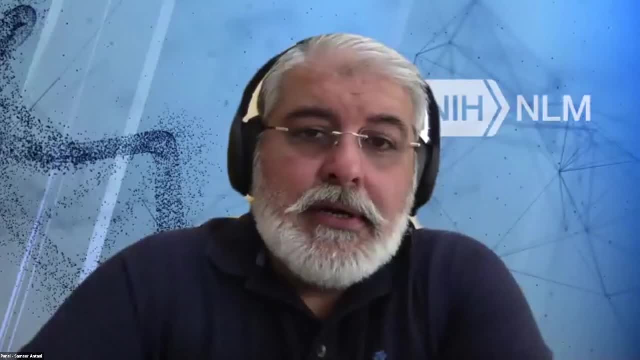 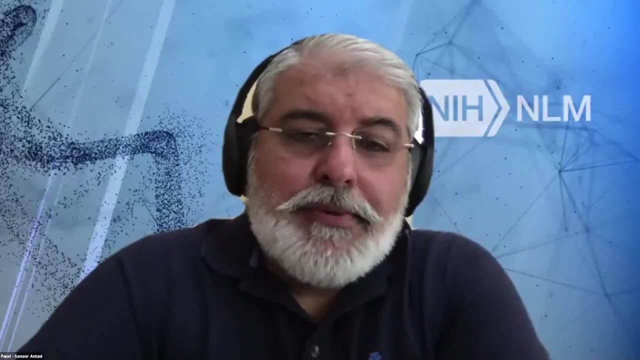 Ana Pereira-O'Callaghan. As Dan alluded to scanning, Mr Technology slides, which is Ana Pereira-O'Callaghan. Well, there are many standards in place and selecting the appropriate scanner and scanning technology may not be the best option. 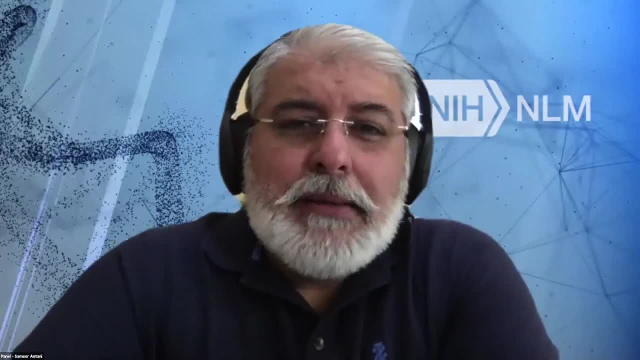 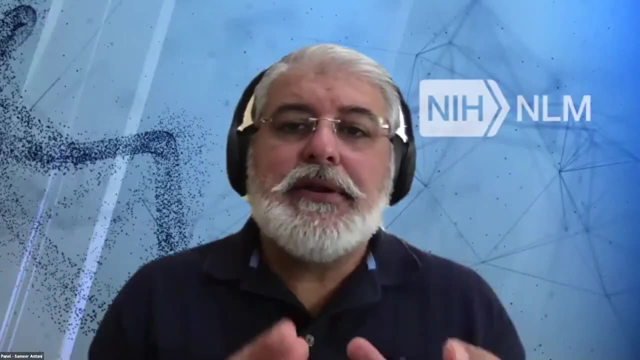 Ana Pereira-O'Callaghan To address some of these challenges. But if you're thinking of acquiring pictures, or you're thinking of Ana Pereira-O'Callaghan, Sampling the population and considering the epidemiology aspects and then considering the critical protocols that are in place so that you don't have the variety, 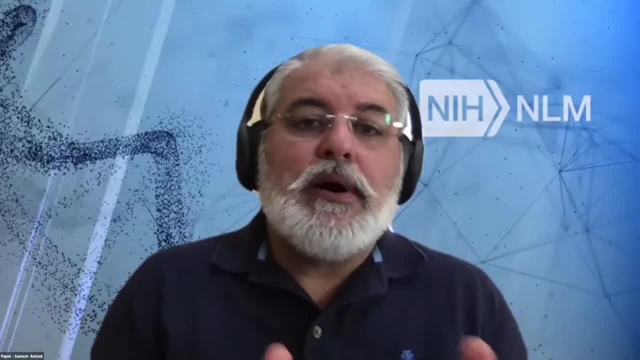 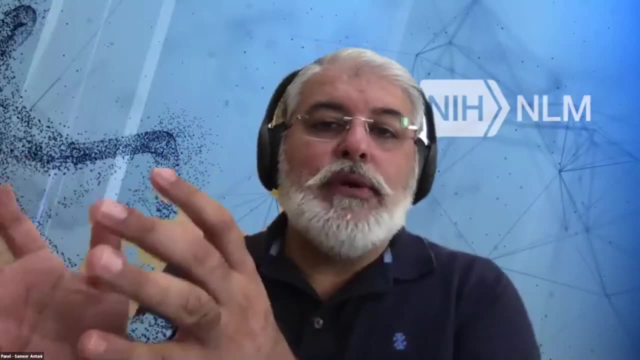 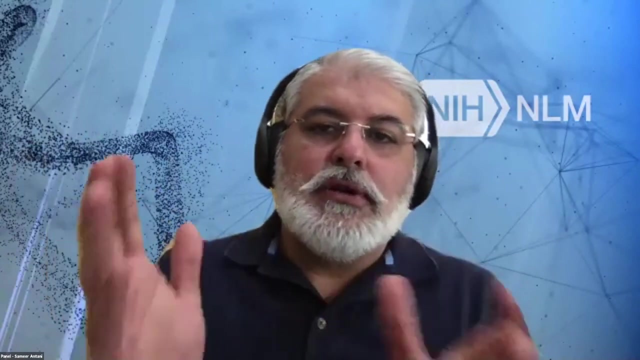 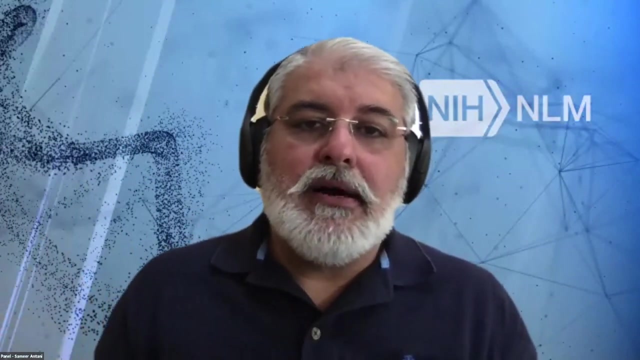 Ana Pereira-O'Callaghan, That would disturb your training. The same time, you don't want to make it so artificial that when you revert back to a natural setting, you have a highly skewed and perfect and air quotes data set. Ana Pereira-O'Callaghan, That is not a representation of reality, So striking a balance between the two. yet if you're pushing the technology forward so that you have a good quality set, 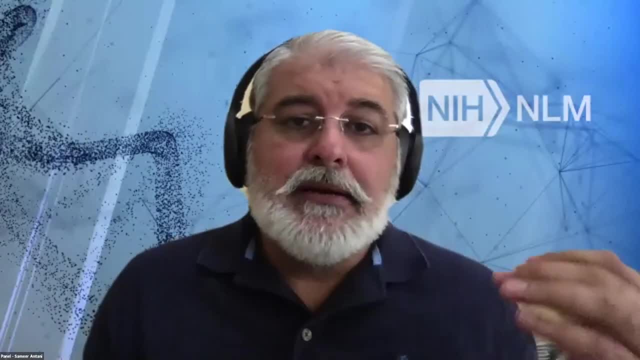 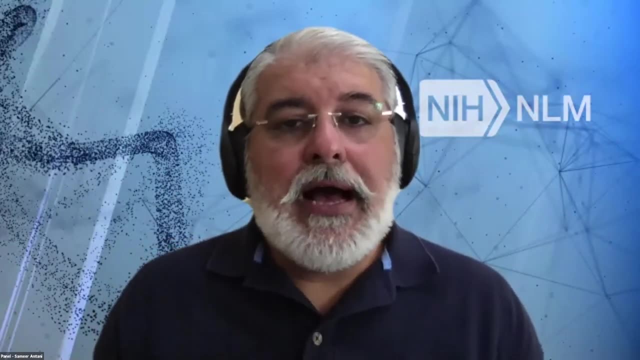 Ana Pereira-O'Callaghan, Giving consideration to this, And one thing we notice is different imaging devices tend to have different imaging characteristics, Ana Pereira-O'Callaghan, And lighting conditions will influence how the picture appears, and human eyes are amazing at adapting at all the variety. 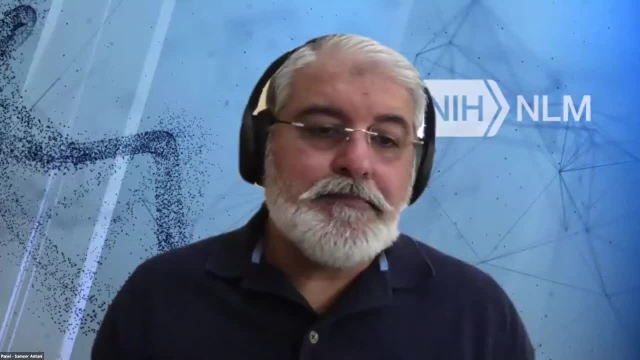 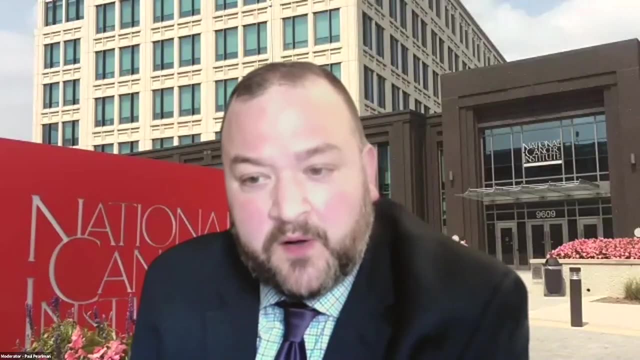 Ana Pereira-O'Callaghan, But computers are still a ways away, Samir Hussain, And I think initially this one's going to be for you, Samir, as well- I want to re ask one of the questions that was asked answered in the chat. 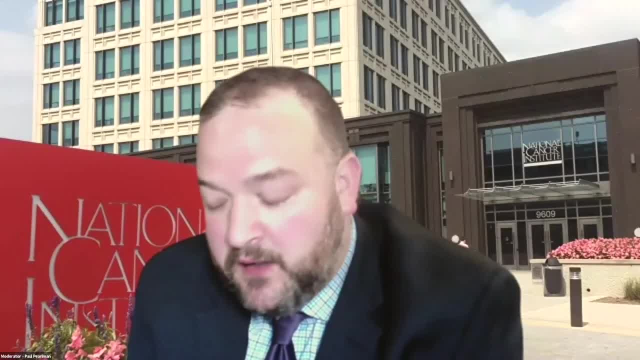 Samir Hussain, And that's: what are the major limitations of deep learning you described and- and I'll add to that: And when we think about deep learning, how do we think about some of the issues associated with the fact that we don't always understand? 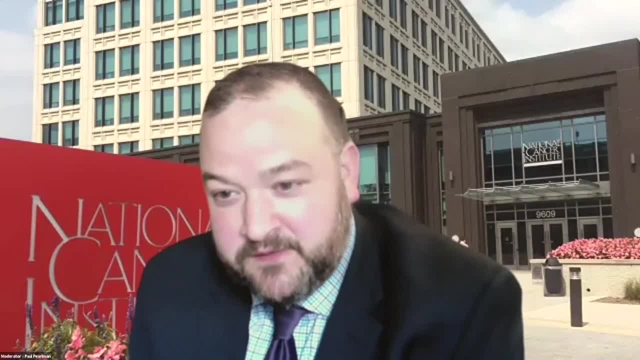 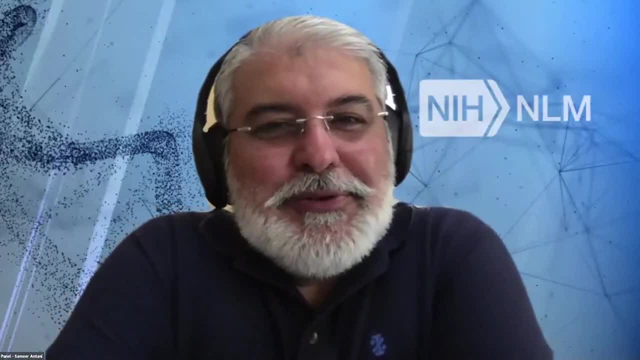 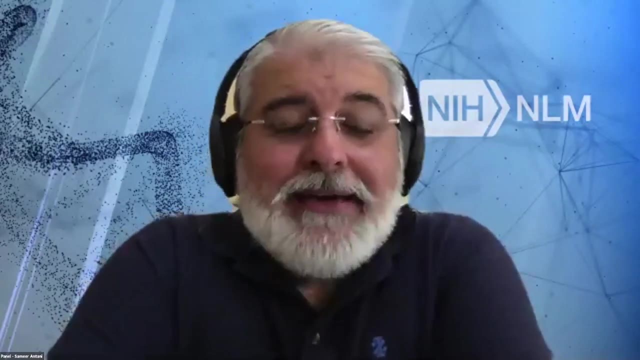 Samir Hussain, Why our algorithms making a certain decision, that is to say the convolutional components, Right, Samir Hussain? That is almost almost entering the space of deep learning. art than science, And this is there is science that you have to visualize the 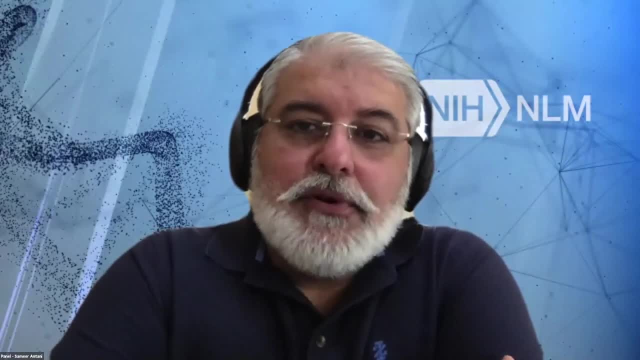 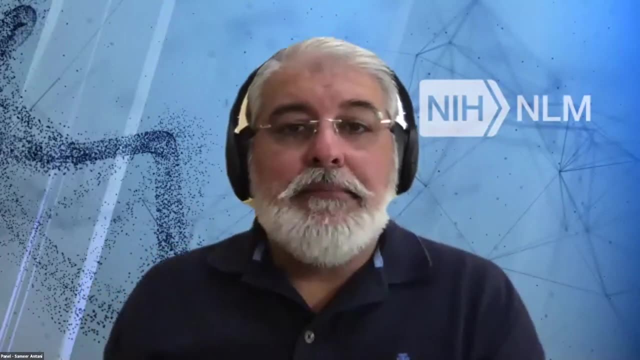 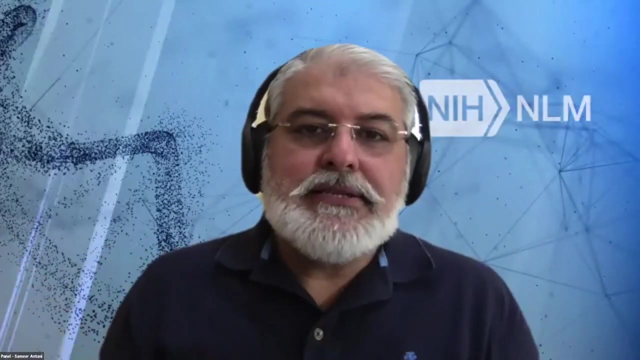 Samir Hussain. What the what the network is looking at and what is focusing on? Now you can artificially Samir Hussain Influence network, Samir Hussain To look at certain regions, using other people in that. So we think of deep learning networks. as decision makers, we can cast. 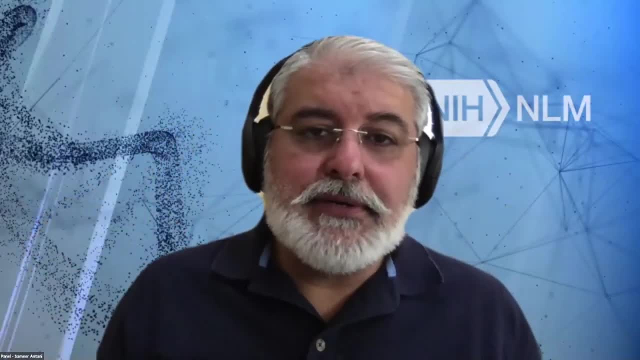 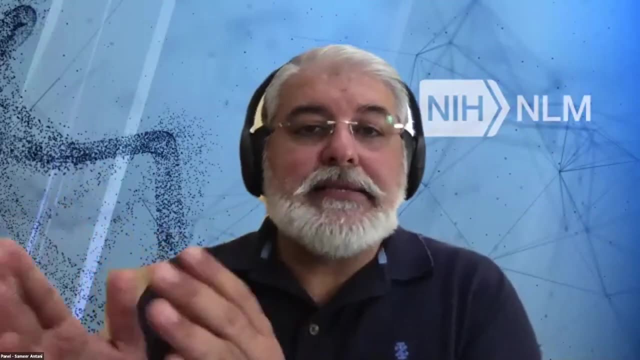 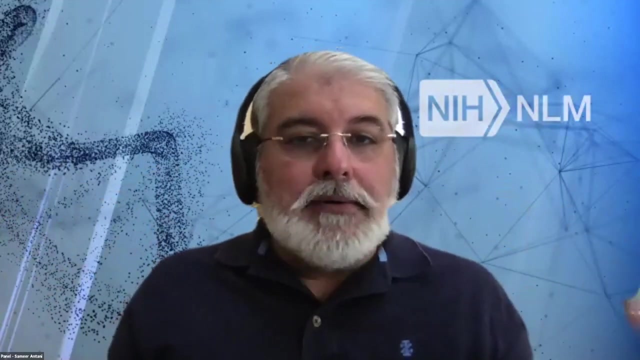 Samir Hussain Segmentation, which is drawing a boundary around an object of interest or recognizing a, an object in an image, as a, as classification tasks. They also are selection tasks. So having a chain of deep learning, Samir Hussain Networks. 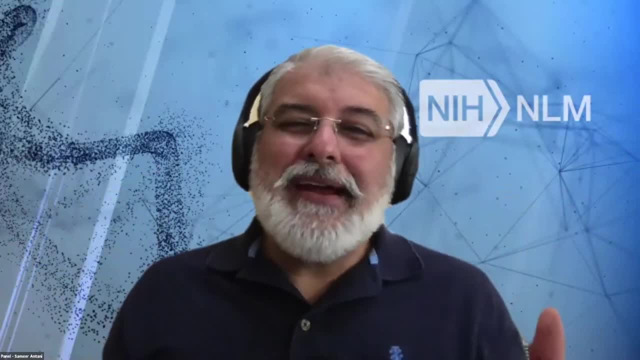 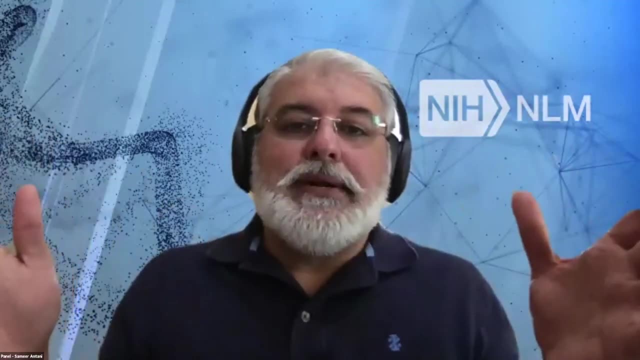 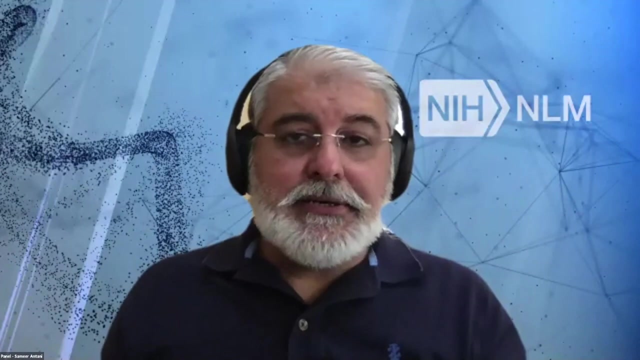 Samir Hussain Can influence them and therefore you are sort of handcrafting a little bit, helping it along and, in a sense, building an end to end system that, given an image, it would, it would percolate through your various networks, resulting in an answer. 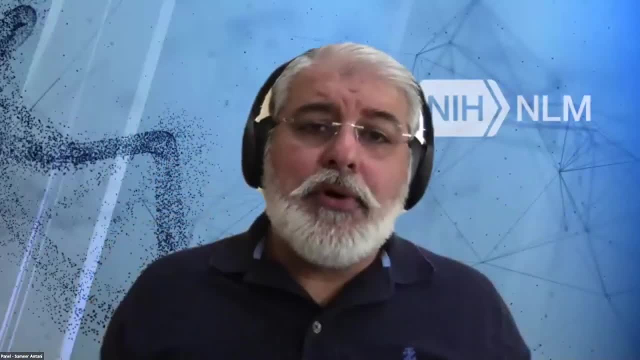 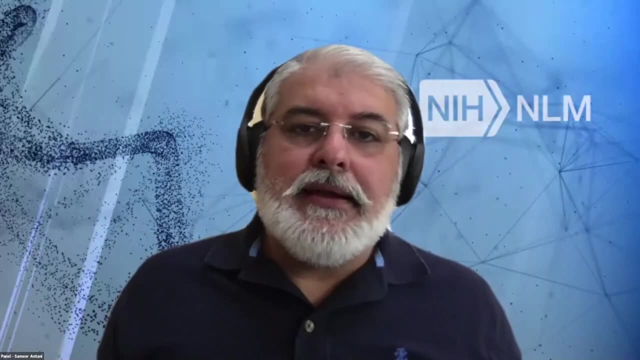 Samir Hussain. But if you think of each individual network, one can put in probes to see if it is being disturbed or distracted from looking at the object of interest and Samir Hussain, And not what you want to look at, Samir Hussain. The only caveat is, if your goal is discovery, that means you have an existing collection you want to find. 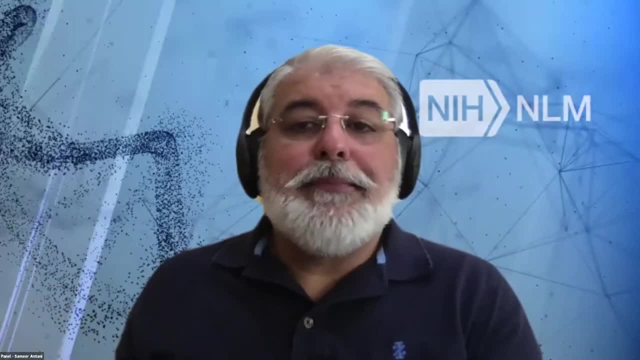 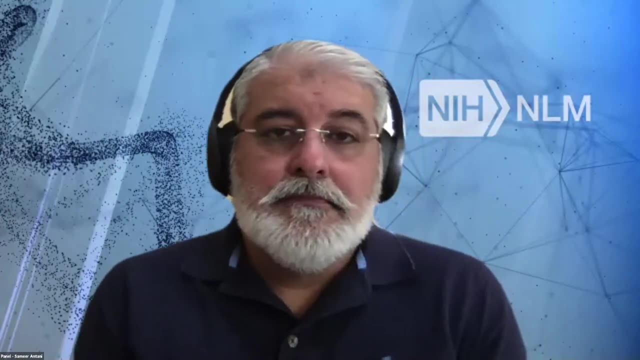 Samir Hussain. Outlier patterns, then there The strategy might not be the strategy, Samir Hussain. So we have a couple questions have come in, looking at the intersection of multi omics data and imaging and understanding the. Samir Hussain. The intersection of multi omics data and imaging, and understanding the. 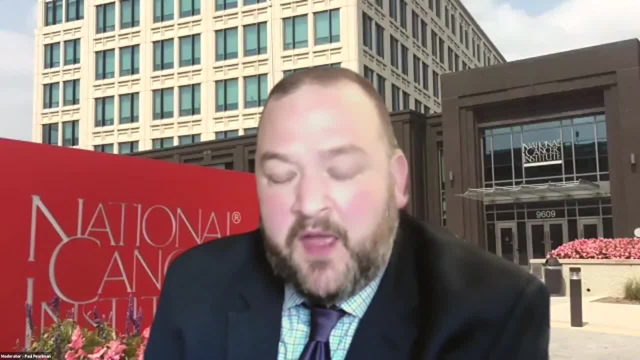 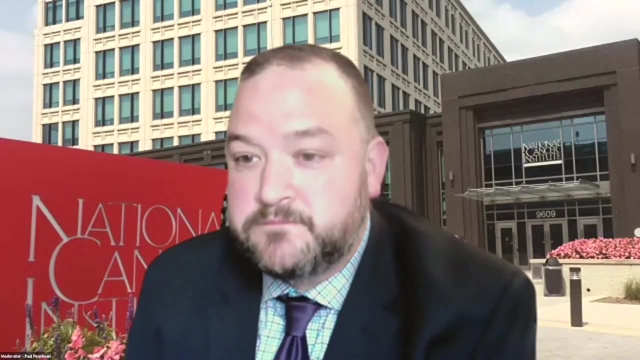 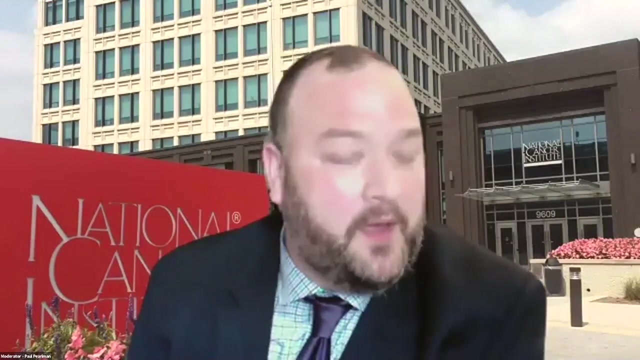 yahoo. yahoo. Samir Hussain btuc, Coa. understanding sort of the value added through adding multi-omics data? I think this question could really go to almost any of the speakers, Anyone So okay, So potentially repeat. could you repeat the question? 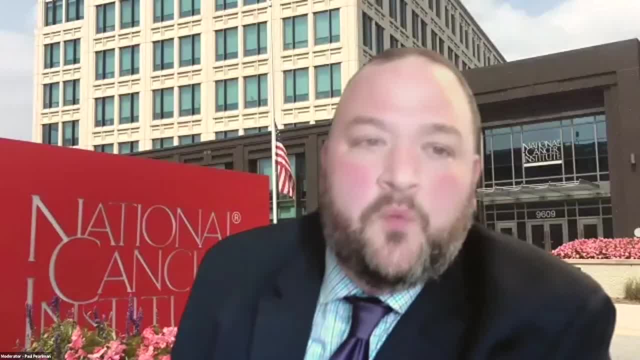 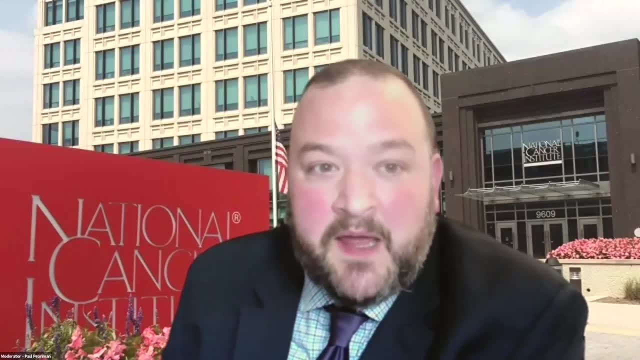 I'm trying to look at it. So the question is: is what sort of multi-omics data has been used in the context of imaging and what is its sort of value added bin, And then sort of what other omics data would be a priority or valuable to increase? 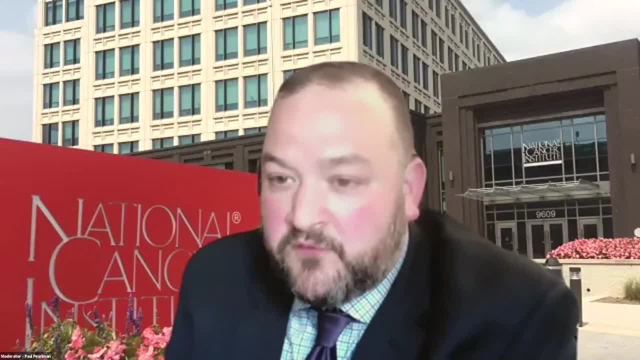 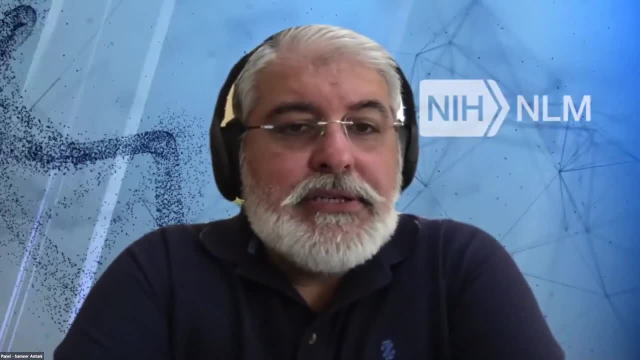 the prognostic value of sort of a machine learning or AI tool. So let me start off and maybe I'll. I'll prod Dan a little if you can jump in, But I think I think he was alluding to this toward the end of his talk. 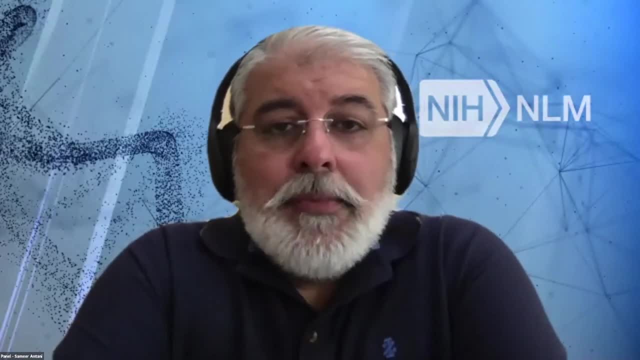 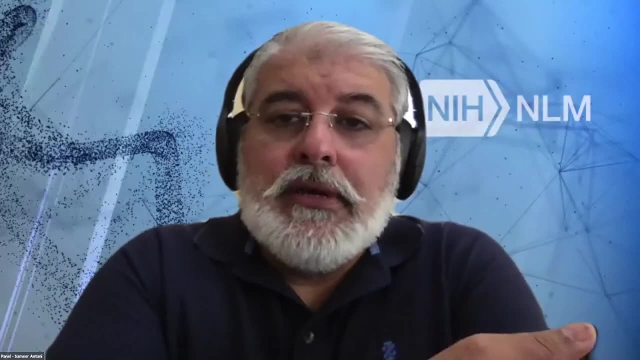 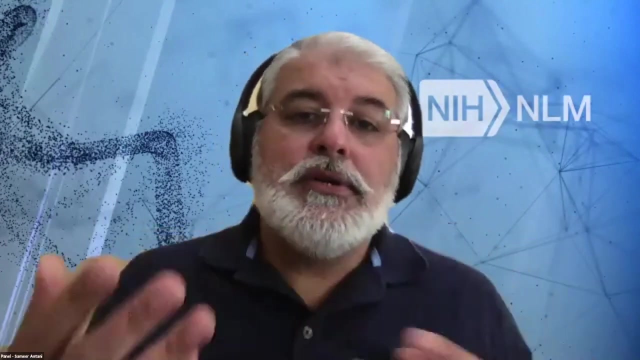 where, for us at least, omics data, as in terms of coming from radiomics, genomics or proteomics, provide a sense of truth, absolute truth that helps us train an image. So, looking at an image alone, you want to. you want the AI to step in and 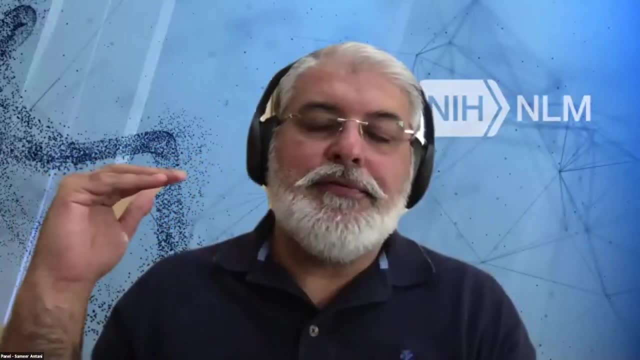 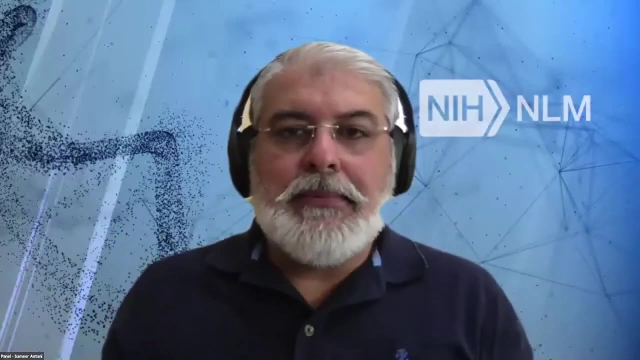 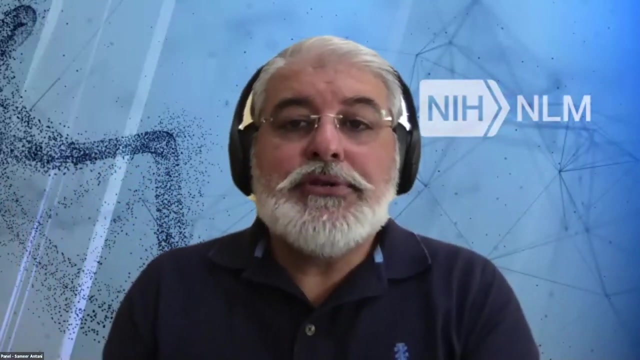 and provide a high standard of truth at a very low cost. point, entry point. So if you think of the cervical cancer problem, where I'd like to use a common handheld mobile phone, let's say, to be able to determine if a 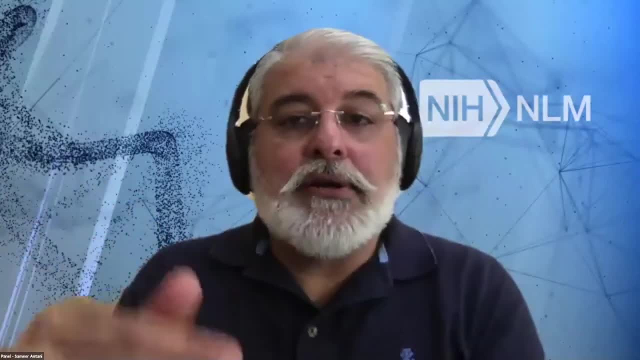 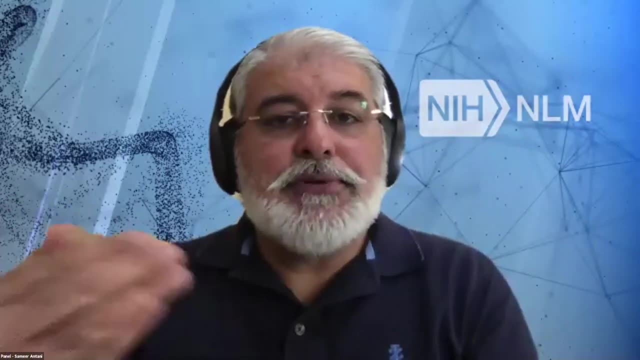 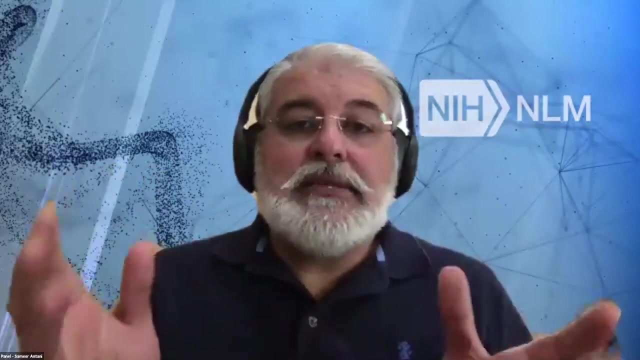 if a woman is in a precancerous, or a stage at least, where she needs more repeated, frequent visits, so that it is, it is, the disease is progressing Now the only way we learned that was true in. now we know that the images themselves don't provide this truth. 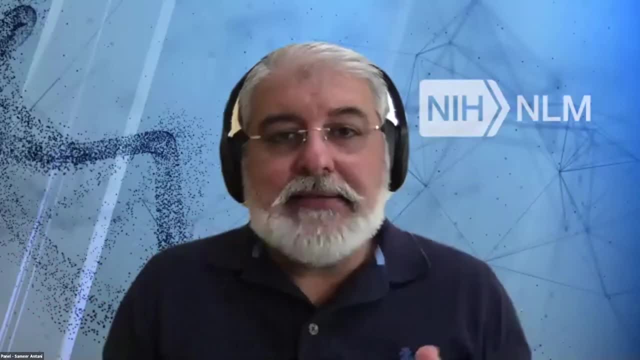 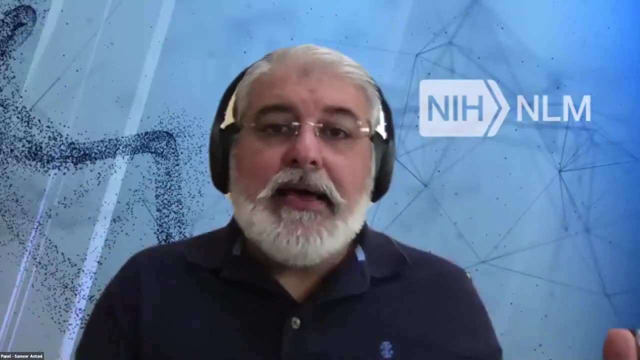 Humans are gloriously bad, but at looking and classifying this. and if you, if you throw the same set of images with the same human truth standard at an AI, it will arrive at the same level, or slightly better, perhaps than human performance. 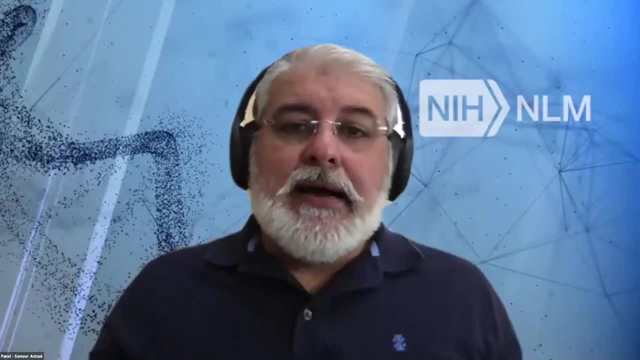 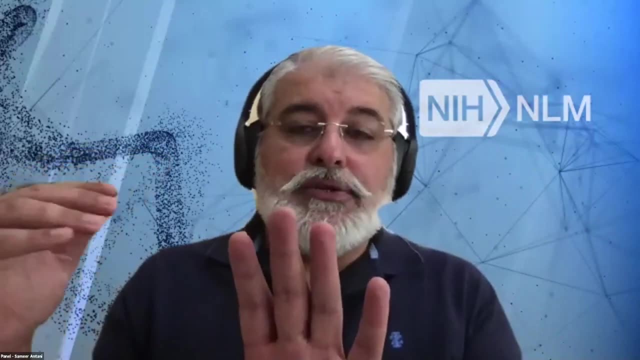 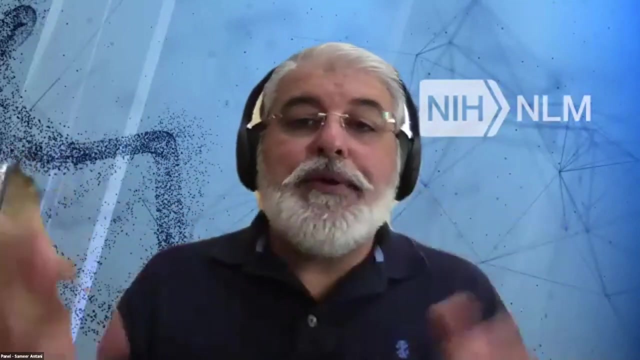 But if you want to advance the AI, then the idea of introducing other omics data as truth standards. So we are telling we are not showing the truth standard to the machine. They're saying that this image truly is positive And now figure something out. 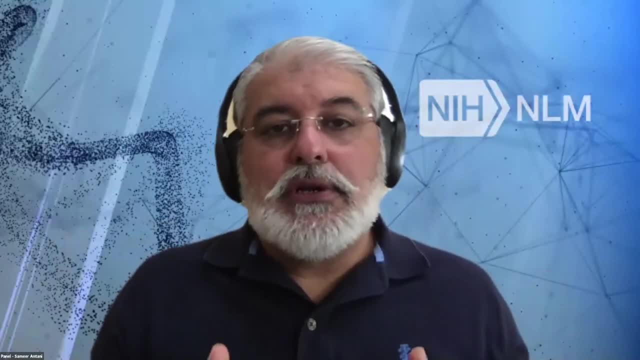 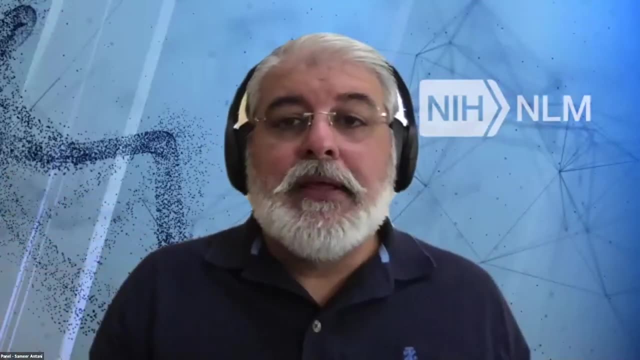 see something more in the pixel patterns that we are sort of abstracting away from so that we can help it. So that's one way is is providing absolute truth standard If you're going to now expand this further and include other health record data. 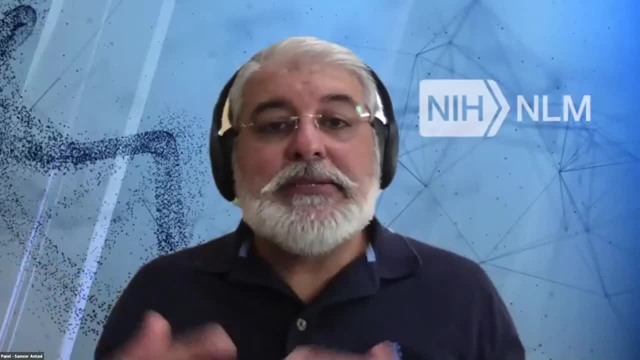 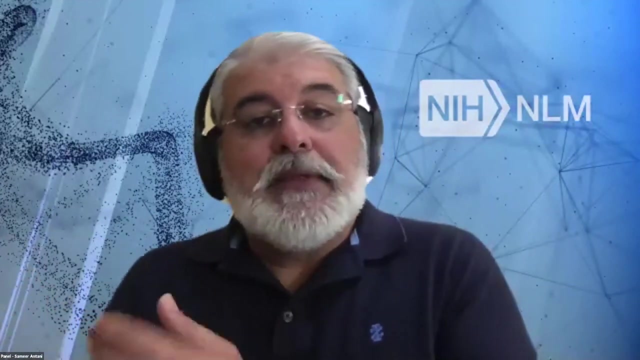 along with other omics data, then you are expanding the kinds of inputs to a much more glorified deep learning network, say, then, so that it can take in multiple input sources and provide, you know, a better level of decision the other way. 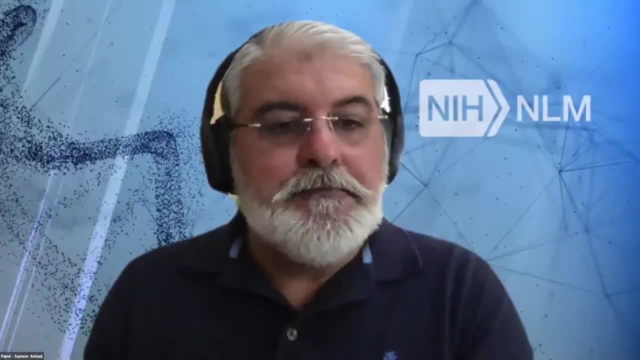 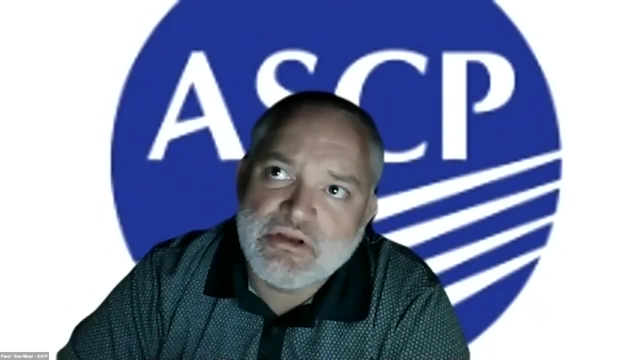 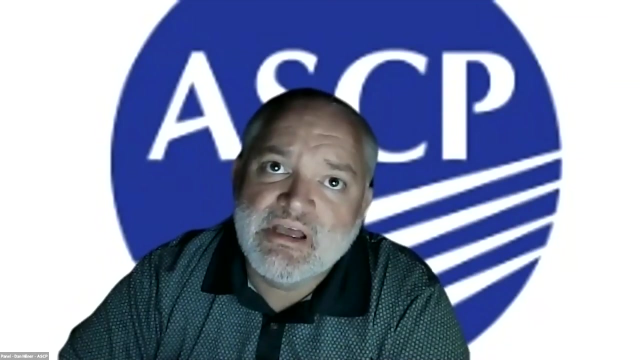 That's one one slant out. Yeah, And I would just add that you know pathology images, for example diagnoses of cancer or subtypes of cancer, mitotic counts, you know classification of tumors to a very high level degree- are often used as the ground truth. 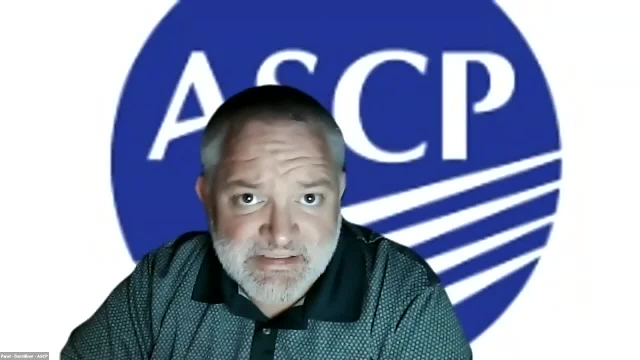 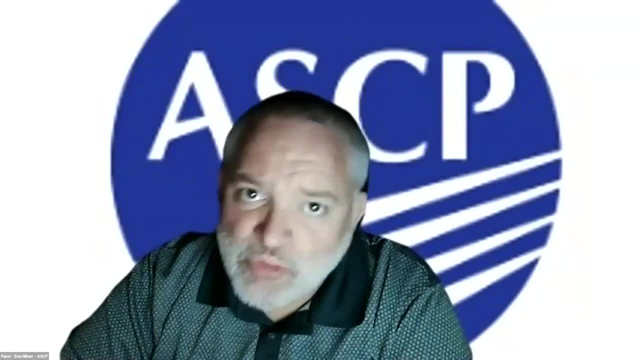 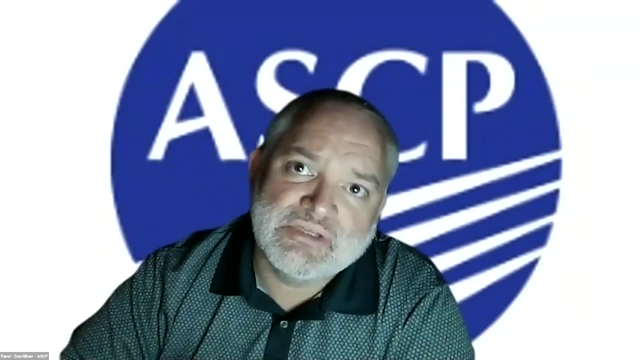 or the gold standard by which to then look at omics, data sets or genetic data sets, et cetera. And I think you know early, early studies, for example, of transcriptional profiling of tumors demonstrated that the transcriptional profiles matched up pretty closely to the histology. 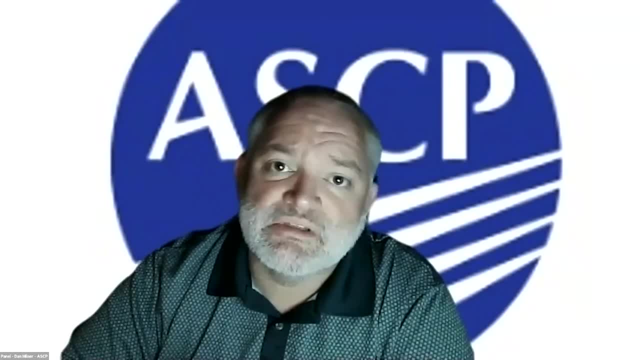 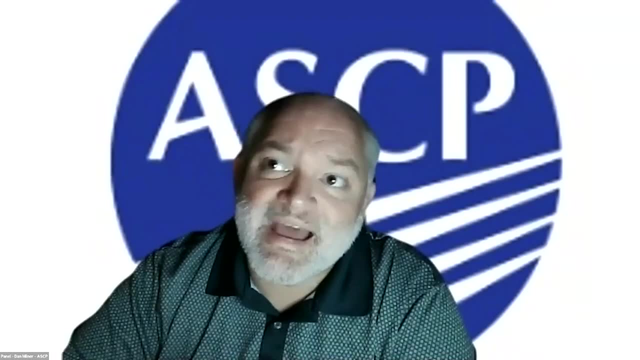 But then, when those data sets grew and became very large, it was clear that within so- for example, adenocarcinoma of the lung- there were subsets of transcription profiles, and that's where new therapies, new diagnostics have actually come from. 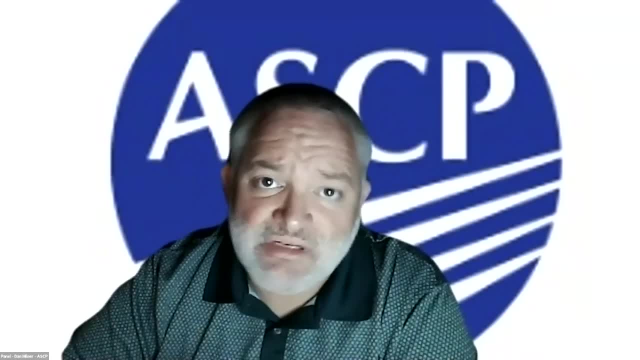 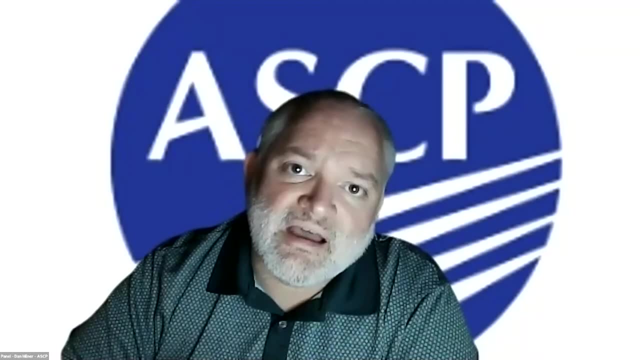 And so I think you, you know you always start with a gold standard, And histology is obviously an excellent one if you have high quality, as I was describing, But the goal is for the, the AI or the, the research that you're doing on the image analysis. 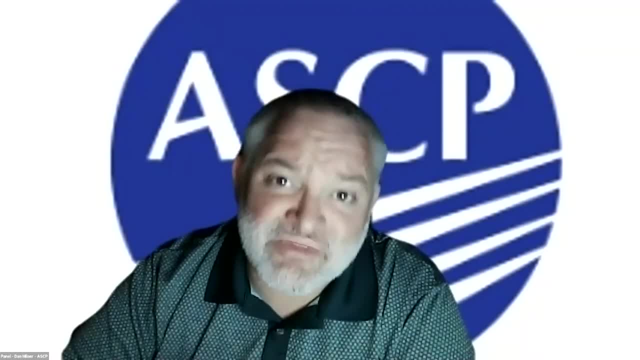 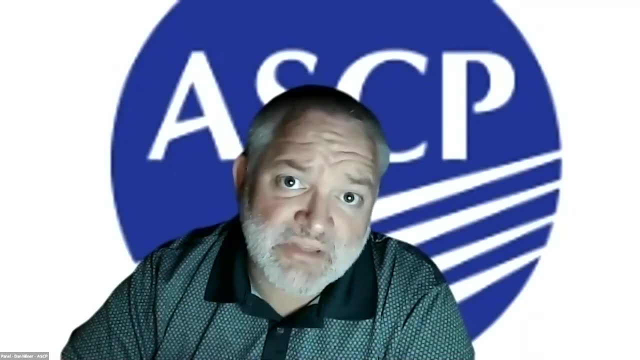 to supersede that and to tell you something new beyond just what that gold standard told you. And I think, as you add more omics data sets to a given grounded data set in pathology, you learn more and more about those images and ultimately come up with better diagnostics. 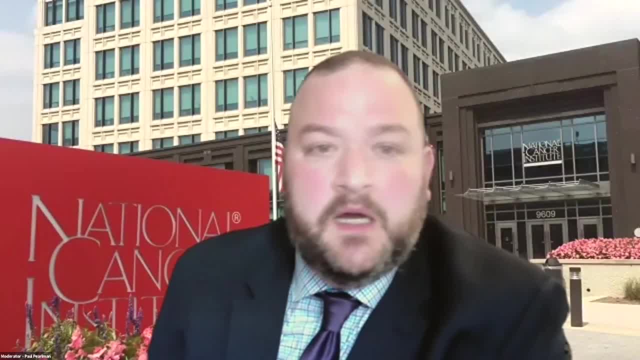 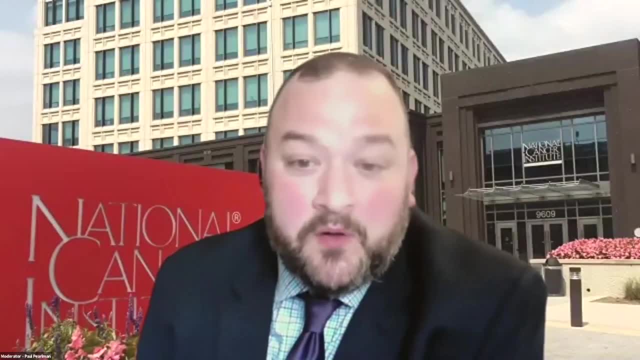 Thanks. I think this one is is for Celia, And so this is a question around sort of how you approach achieving an equitable AI tool, That is to say, and the question goes further to ask whether you use a multi-model, sort of per country. 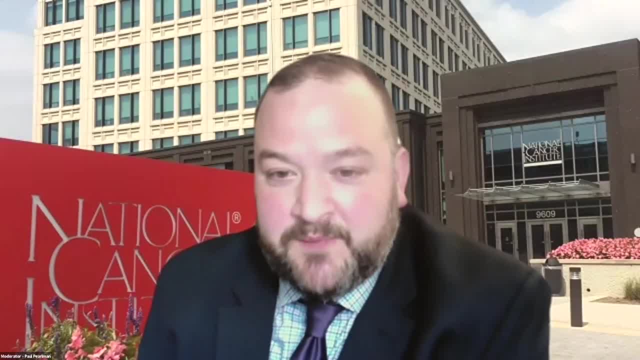 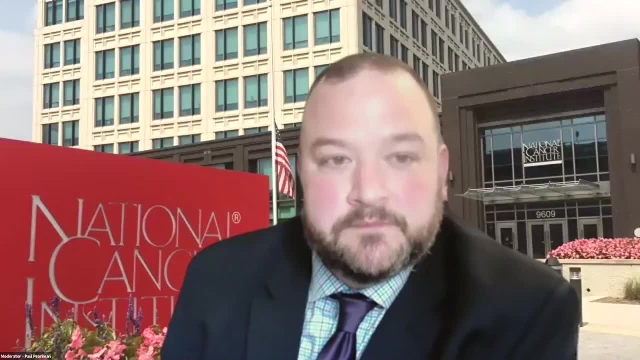 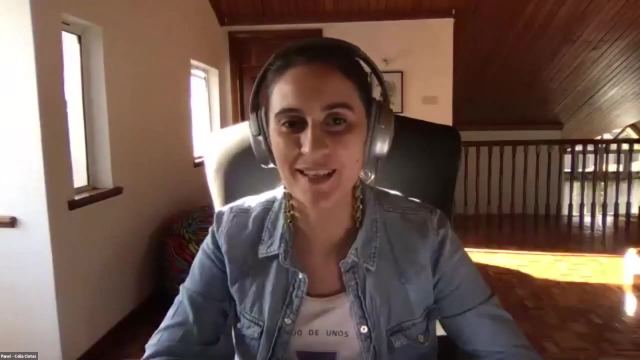 or per population approach, or a single model attempting to be more general? That's a good question. What we learn, at least for our specific problems, is always by population base. Right, Because you will not have a one single model that will tackle all different populations. 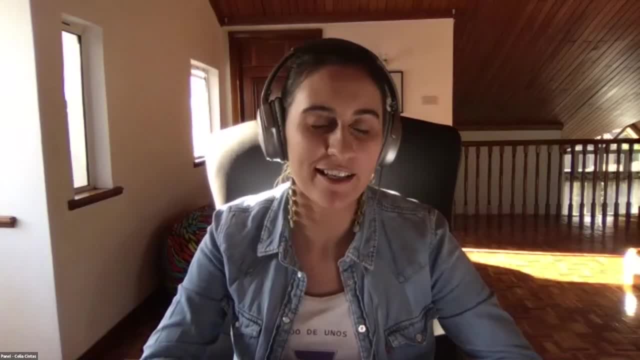 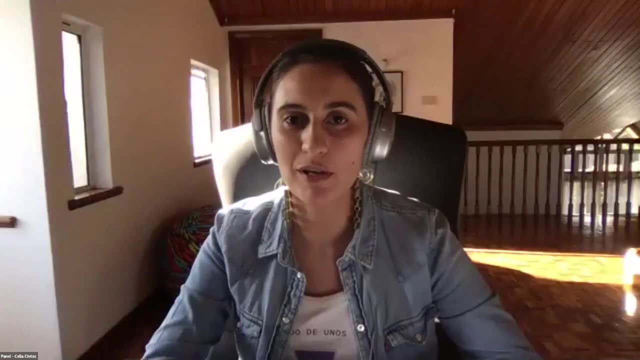 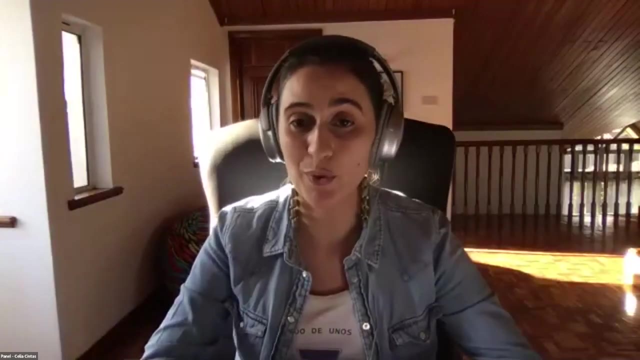 Regarding fairness and equitable machine learning, I think the first step is be transparent about how the model was trained. what is the population that was working on, as when other other researchers in other cultures or other side of the world are adopting this, already trained? 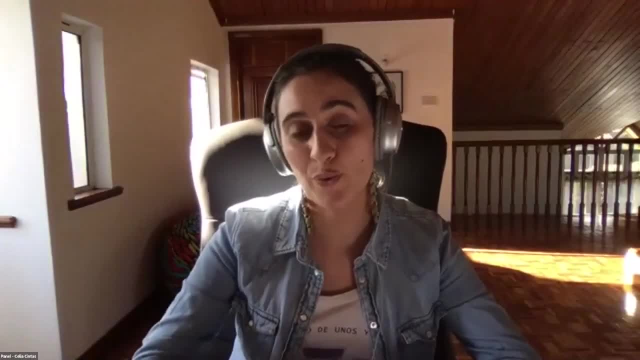 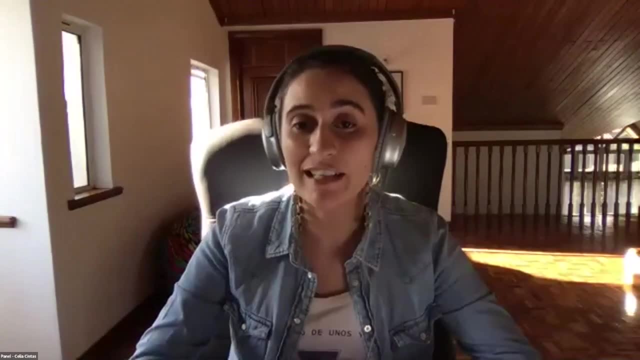 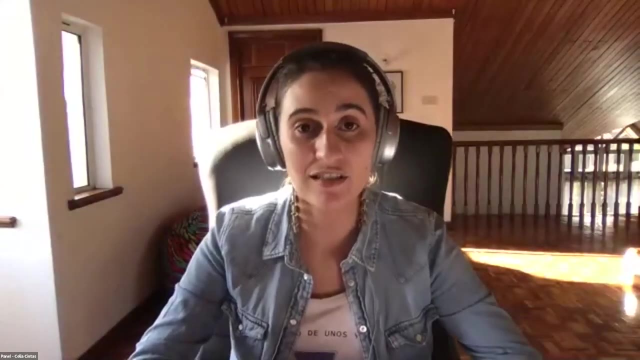 model, To what extent this model will work for my problem. So the first thing it will be to be transparent, And then one very interesting comment is: how can we introspect these models? One of our panelists showed the ground cam visualizations. 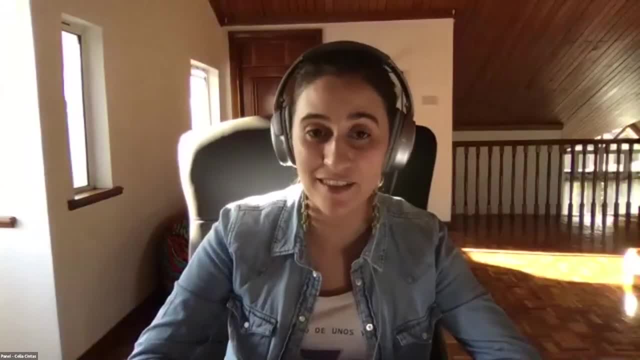 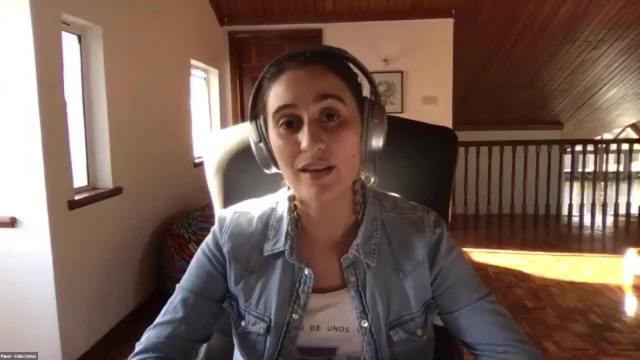 These are things that help you understand how the models makes the decision, So you can have- you can have a notion on why that's important, And I think that's really important. Yeah, Yeah, So I think, introspection of the model and be transparent on on on the limits, on how. 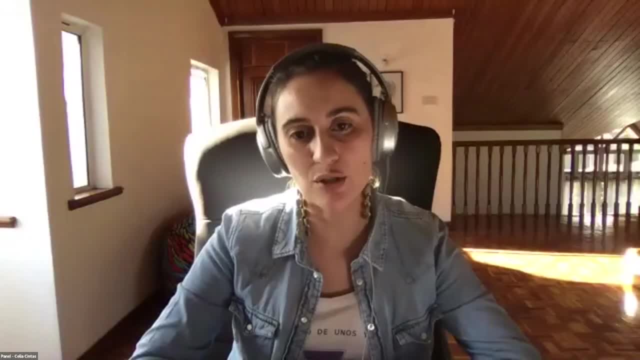 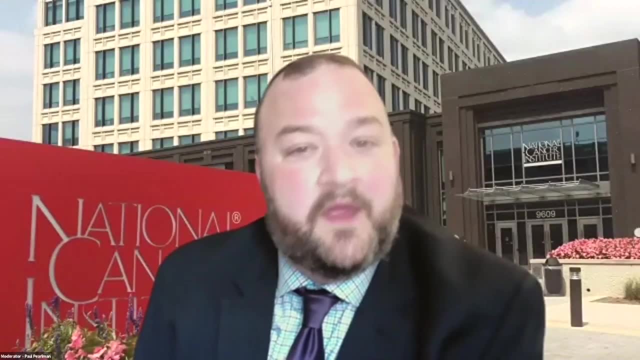 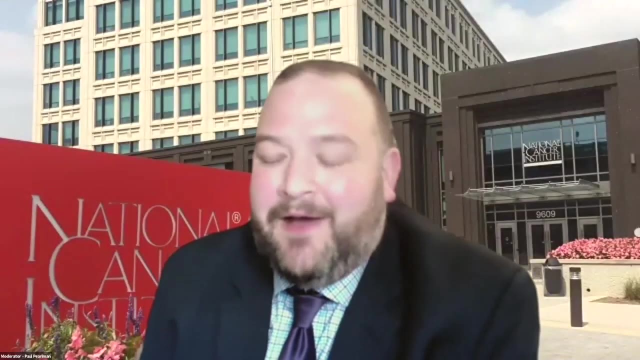 was trained and the performance is done is super important to to build better machine learning solutions And thank you. And our next question is for Michael And the question asks: sort of how big of a data, sort of a collection of data, do you? 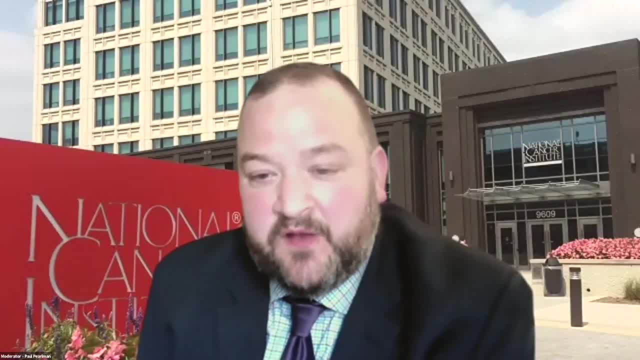 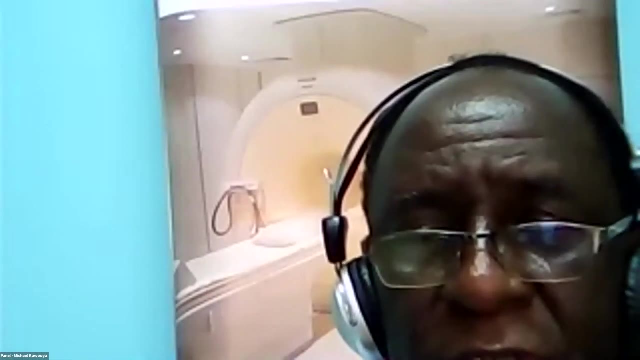 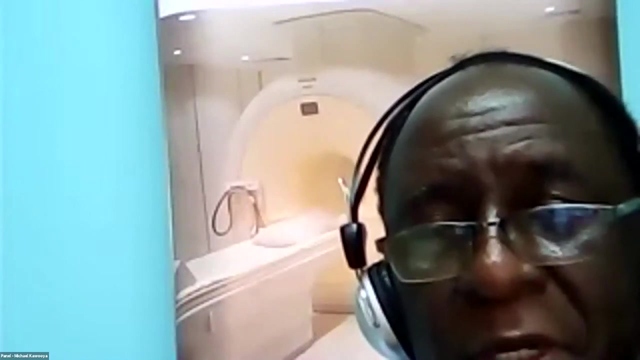 need to start thinking about image analysis and AI diagnoses in the context of ultrasound. Ultrasound can be very tricky And, depending on, for instance, if it's something like a gallbladder stone, where it's a yes or no, then you may not need so many images to train that. But if you're 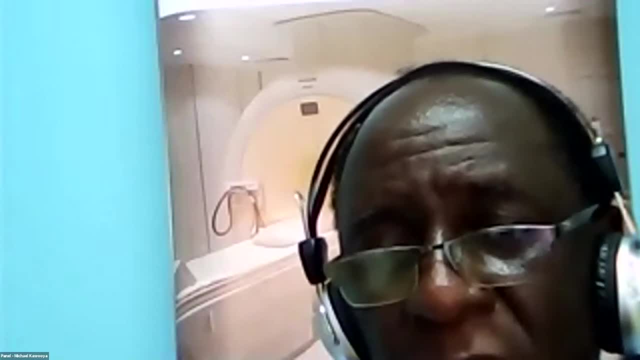 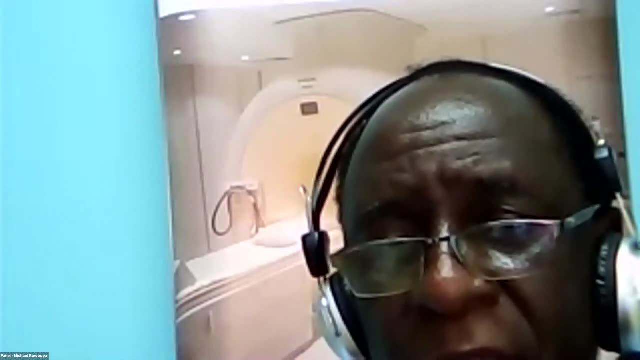 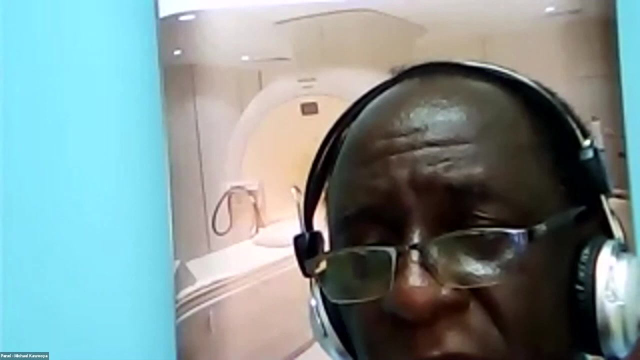 looking at something a little more complicated. for instance, if you're looking at a breast cancer, where there are different varieties depending on the virus, then you would certainly need several hundreds of pictures to do that, So it will depend on whether it's a black and white. 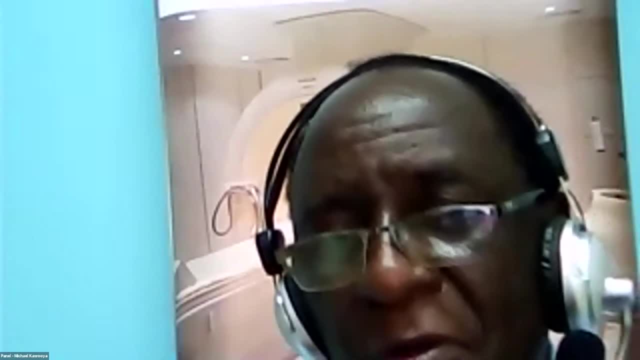 like gallbladder stones. are they there or they're not there? Or whether, if you're measuring a gallbladder stone, are they there or they're not there. Or whether, if you're measuring a gallbladder stone, are they there or they're not there, Or whether, if you're measuring a gallbladder, 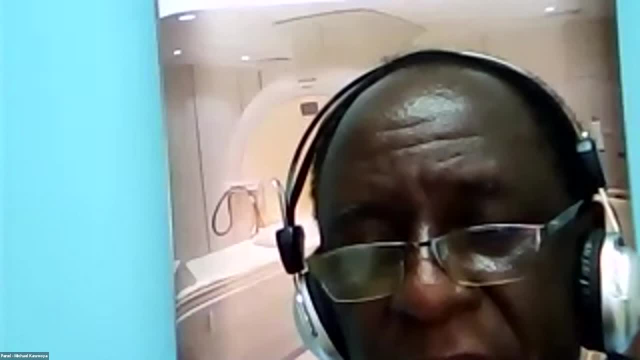 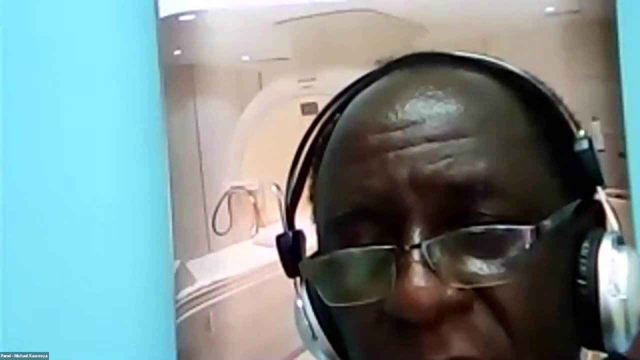 stone: are they there or they're not there, Or whether, if you're measuring, for instance, bipyretic diameters in a fetus or the femur in a fetus, that's a little more straightforward, But where there is a little more heterogeneity, where the image is more complicated. 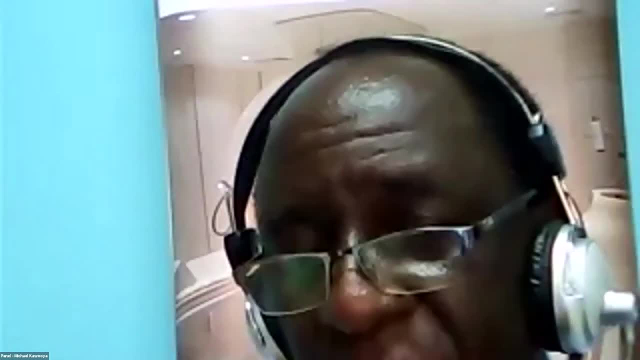 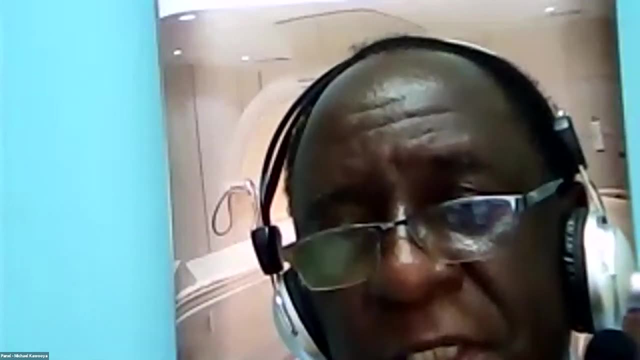 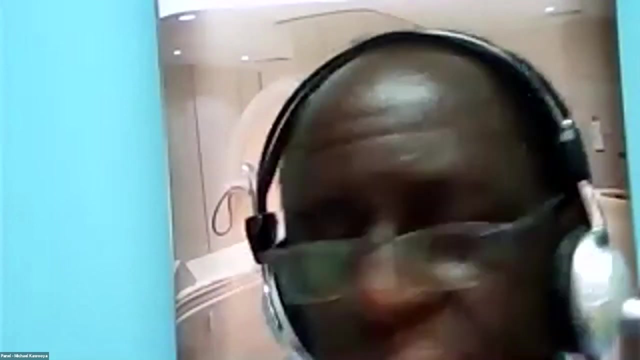 then you certainly would need more models because there are several varieties of that disease. But usually the ratio is to have about 70 training data sets to about 10 or 20, of testing and validating. So that ratio, one should attempt to have a big training data set. 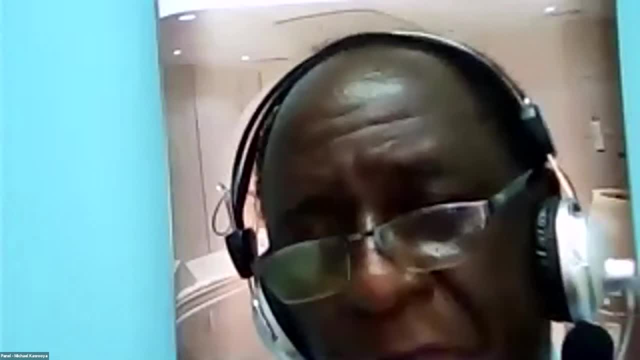 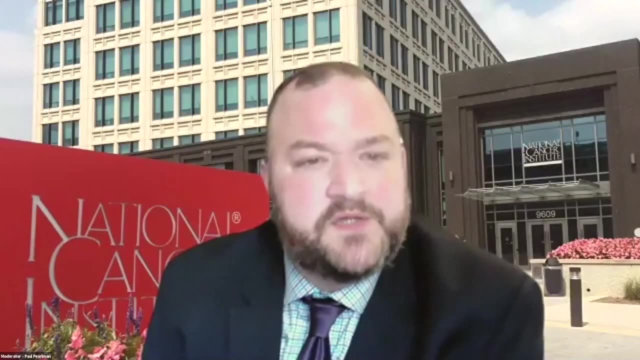 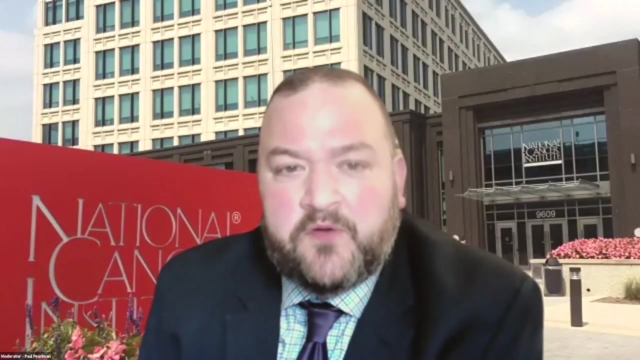 and then about 10 or 20% of that as testing and validating data set. Thank you, I think this next question could be for everyone And it asks whether there are international standards for characterizing images that could be helpful for having good data sets, And. 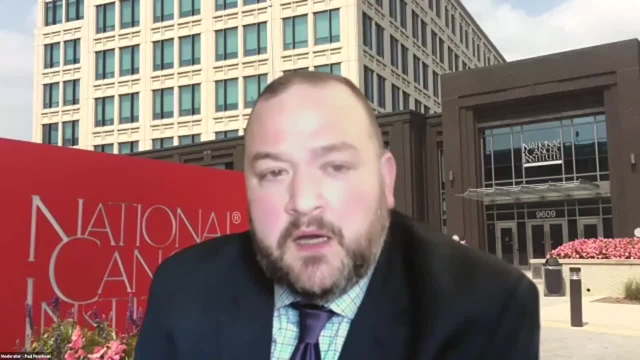 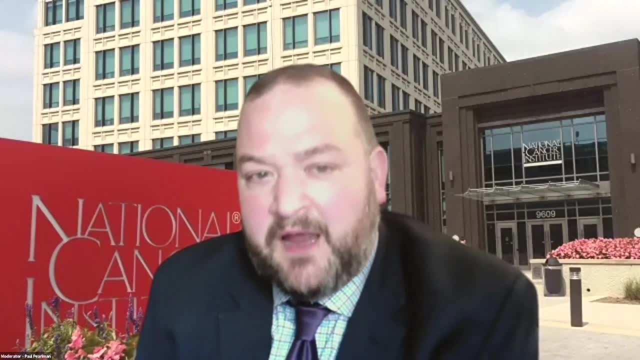 then there's a second part to the question where the person asking the question is concerned, that, based on the discussion we've had so far, that each research group would really have to collect their own initial images to make sure that they're sort of clean or conform with what is needed for the 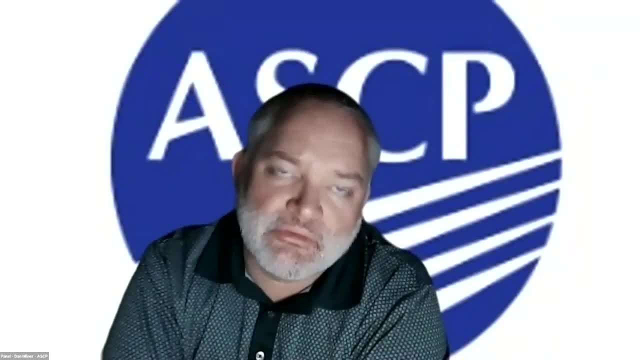 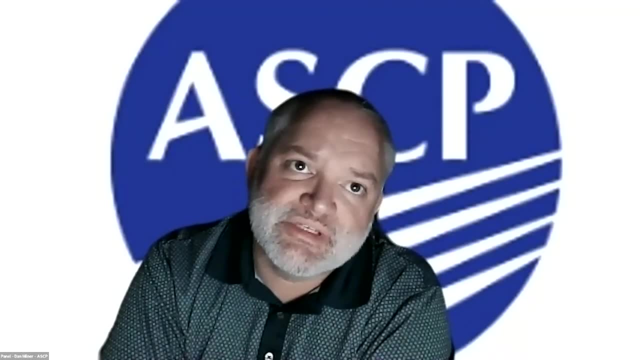 algorithms. This is Dan. I'll just comment very quickly. For pathology, there are, as Samir alluded to, there are standards for how to use full-slide imaging systems to collect images. There are also standards for how to use full-slide imaging systems to collect images. There are also 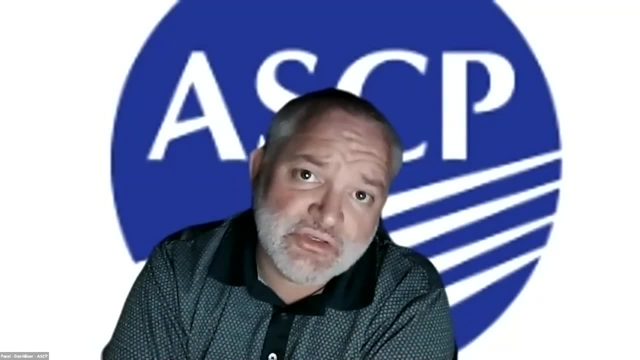 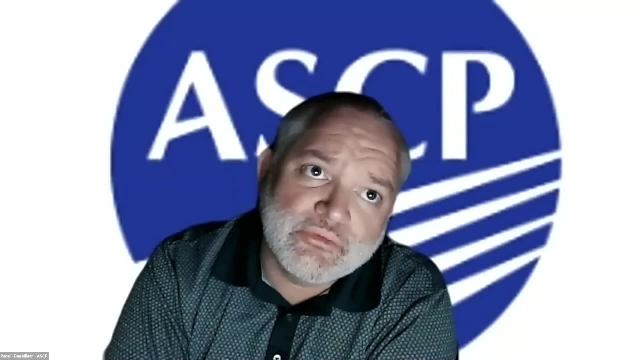 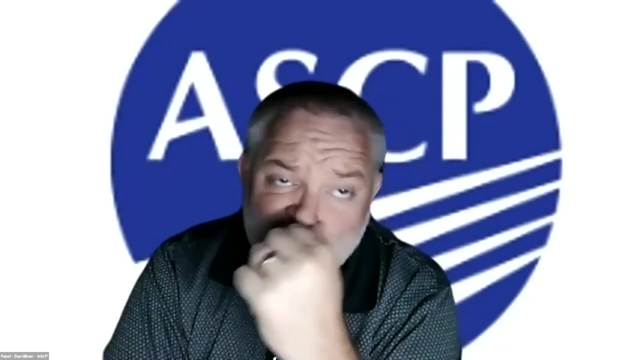 standards for histology quality, cytology quality, et cetera, And those are sort of large and complex, But at the end of the day, when you are doing, for example, an oncology project or a clinical trial, as could be done in this grant program, and you need a correct diagnosis, there are standards for. 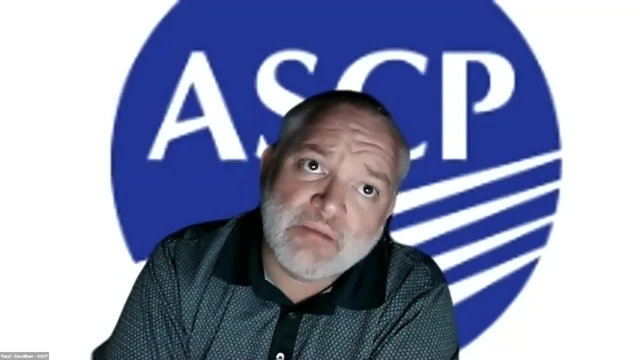 reporting of cancers, which include all the different features that come from the image, but they aren't about the image itself, They're about all the other things. So there are quite a few standards out there, And for the second part of the question, there are standards for 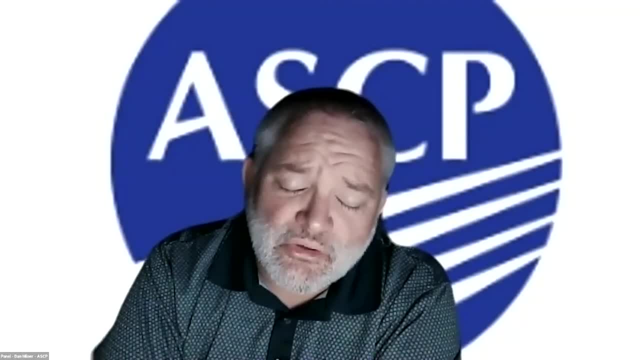 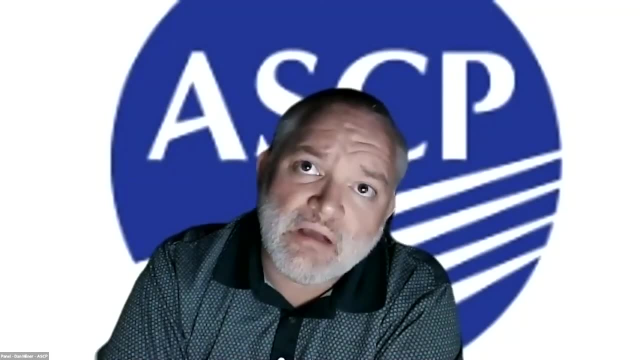 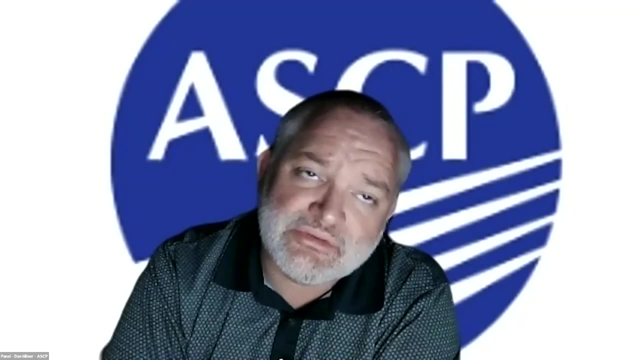 collecting data. And for the second question, I think if you are going to collect your own data- and I think Celia's point is really well taken- if you're going to collect your own data, likely someone has collected a data set like that before And so seeking out those existing data sets to use. 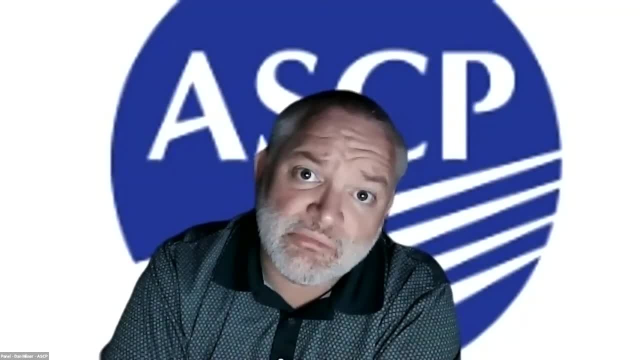 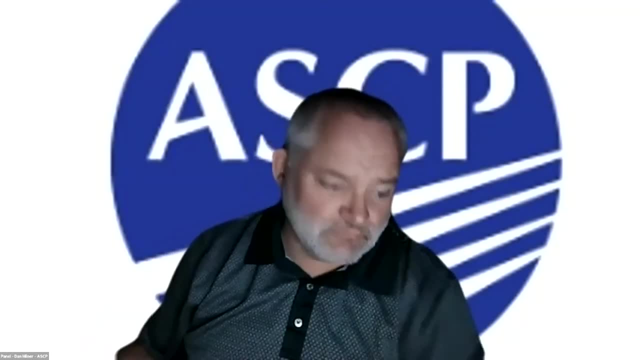 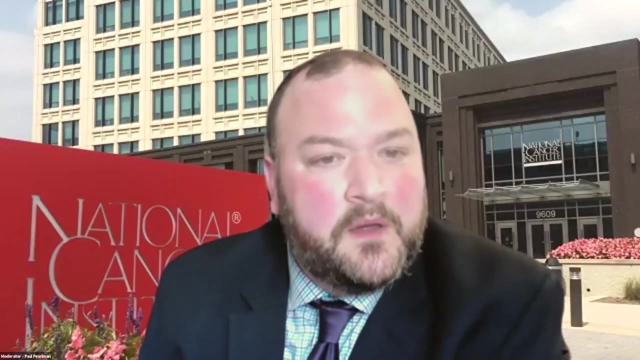 as a comparator, to use as a high-quality gold standard against your images, is probably the best way to normalize your data set and correct any problems early on. Okay, thank you. So our next question is what- and I think this is for the whole panel- 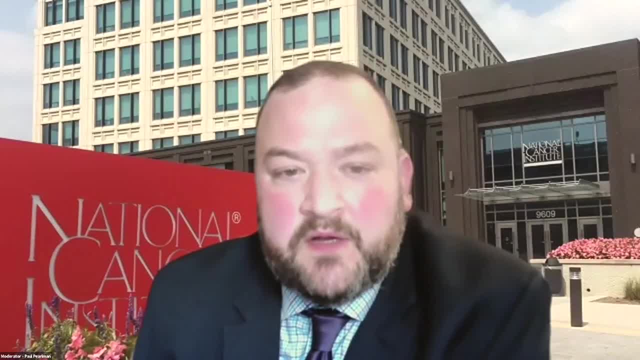 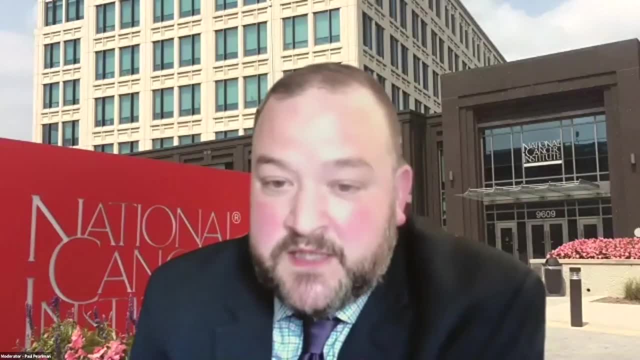 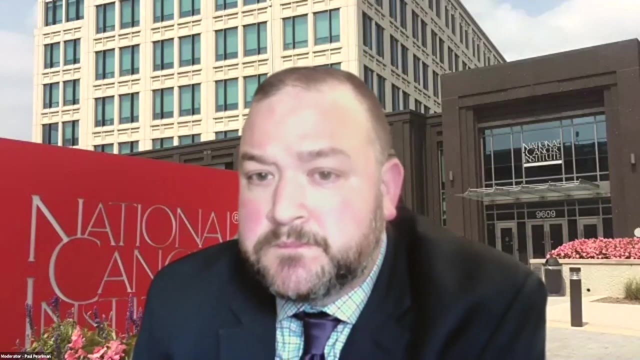 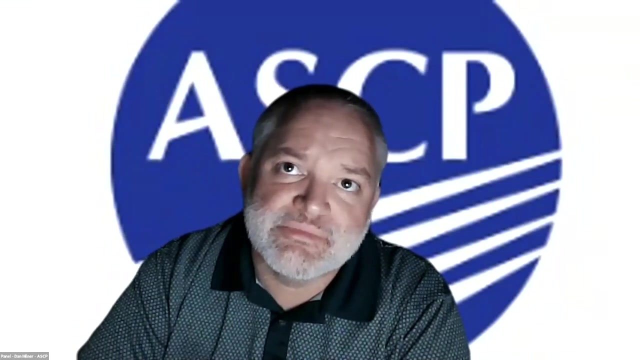 potentially as well. what are your thoughts on the utility of crowdsourcing or other similar strategies for annotating imaging data or pathology data? So the potential role of citizen science. I'll just add really quickly, Okay, Okay, So part of what we do at ASCP with our telepathology virtual support system is each country where we 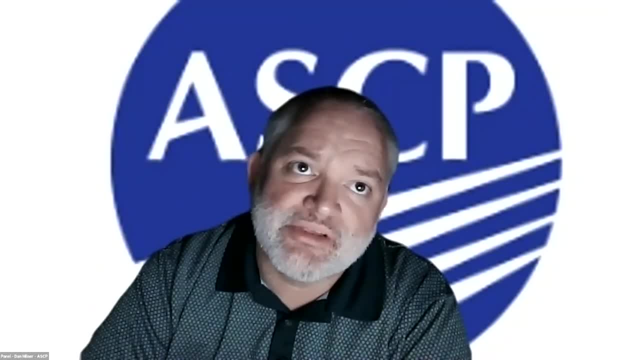 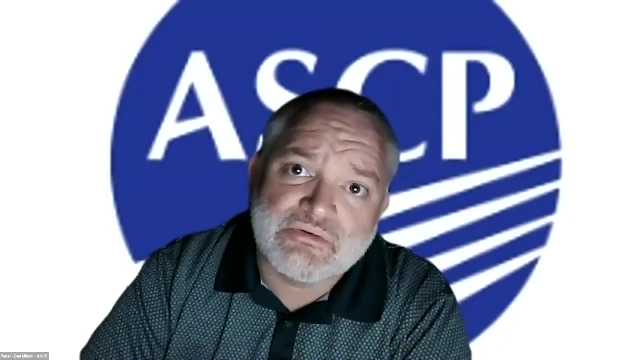 place whole slide imaging equipment has a team of 15 US-based pathologists that review those images with them. So if that site decides to engage in a research project, they have automatic crowdsourcing of 15 experts to review their cases. For those of you who are planning on or thinking about pathology, 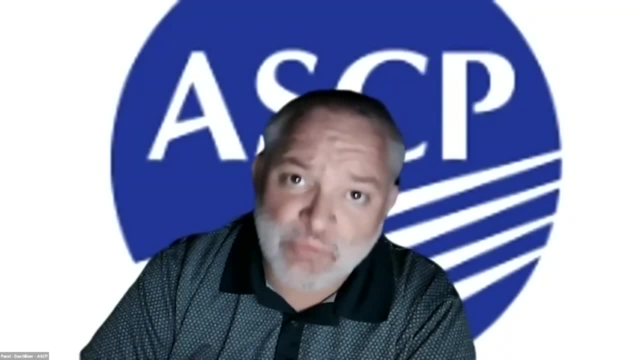 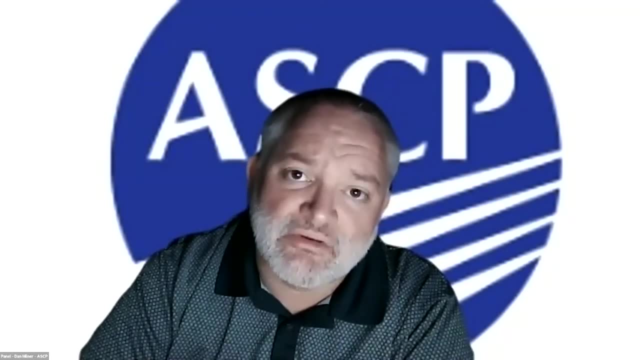 I can offer that ASCP would fully help to support you in that regard, if that's something that would be helpful for you for image validation- And I think it is a very, very vital way to make sure your images are high quality. If you have one pathologist, look at a histology slide. they're. 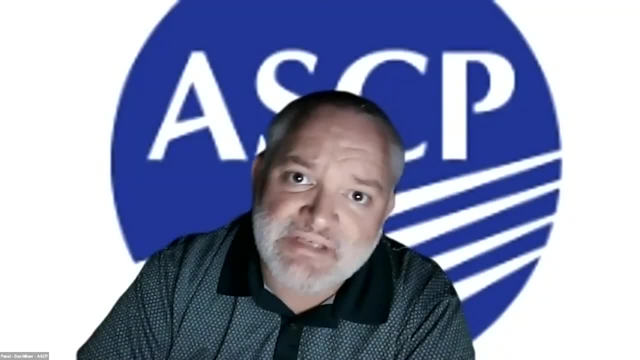 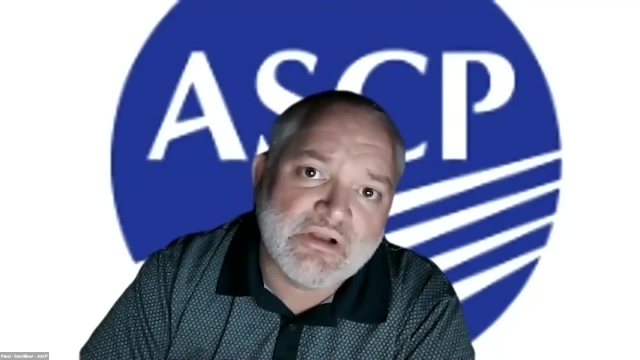 about 60% accurate. If you have two, they're about 85 to 90% accurate. If you have three, it's a 99% accuracy on the diagnosis. So crowdsourcing is really crucial, especially for complex cancer cases or difficult histology. 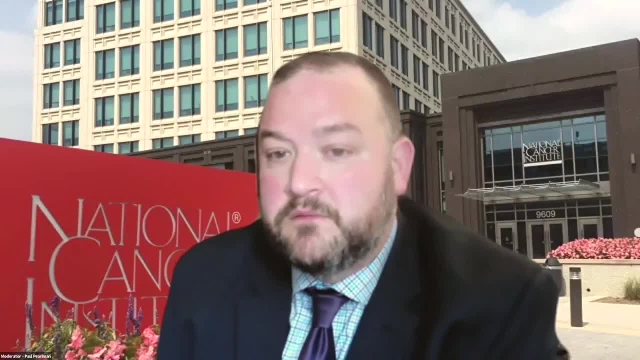 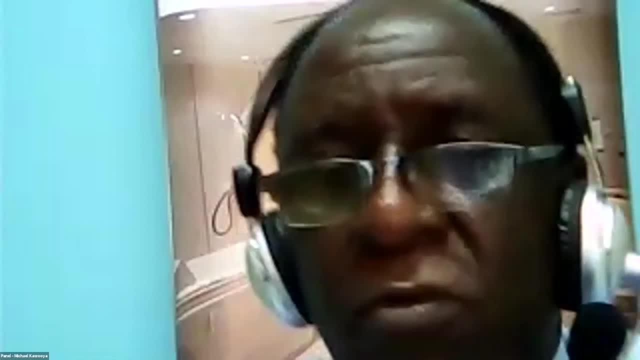 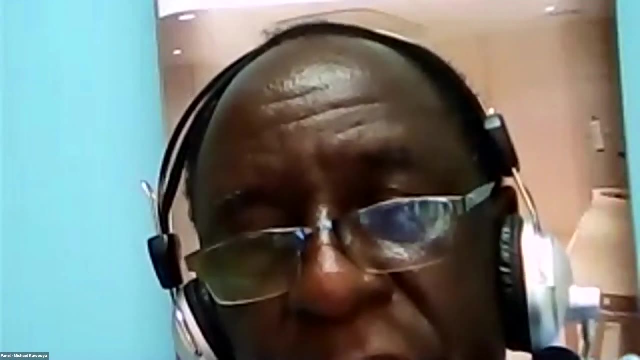 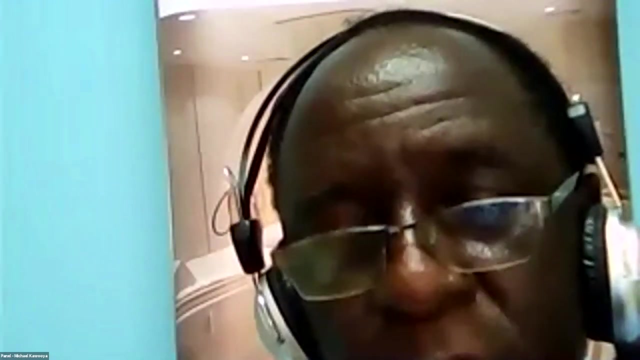 Any other thoughts. Okay, In Africa, where you have limited expertise, certainly would need to have some other person look at it and validate the imaging, And that's why it's important for us to have colleagues in the US or elsewhere who have experience in that disease condition or who see. 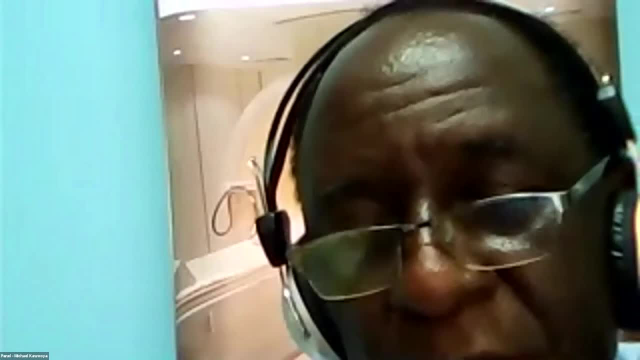 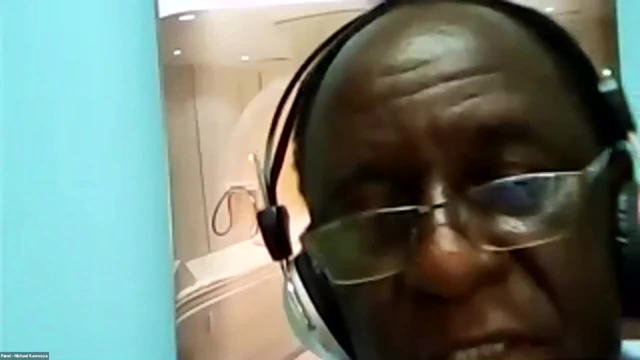 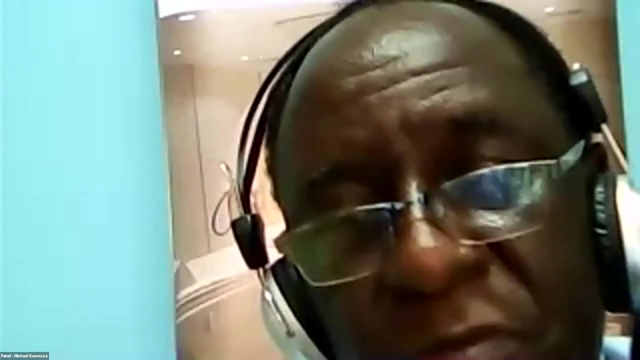 many of those pictures So that together then we can have a higher degree of accuracy or validity for that image. So for us in Africa certainly it's important that we team up with another university or another research centre where they are also seeing many of those images. 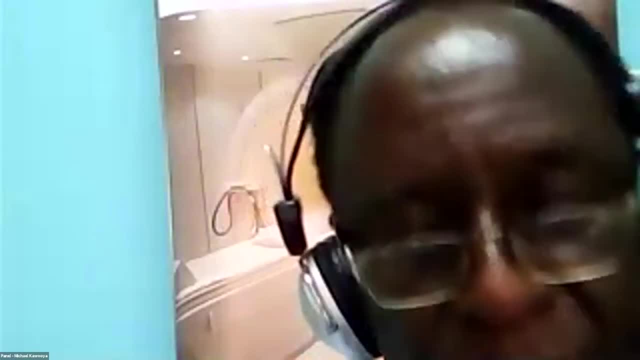 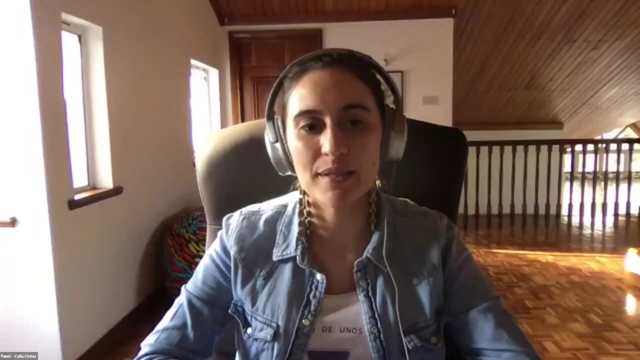 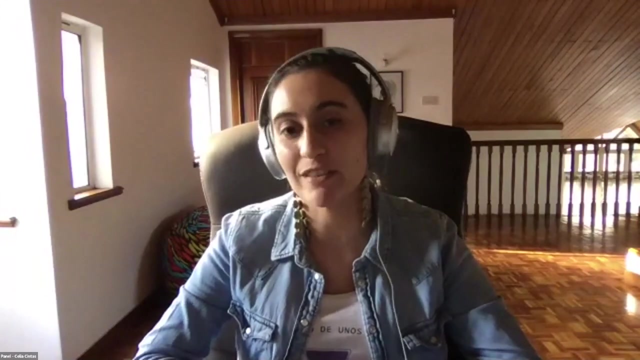 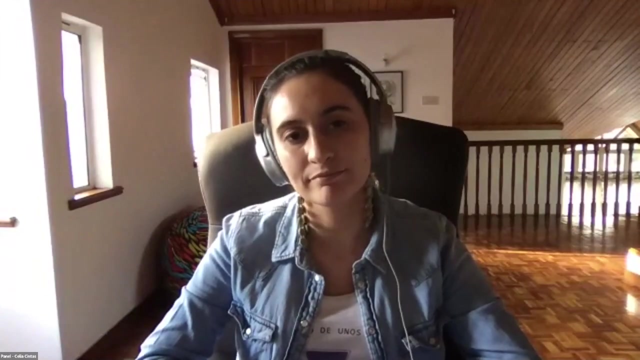 and have more experience than we have. And a small addition to this will be to always keep inter- and intra-observer measurements, where we use crowdsourcer to be reported next to the data set and the labels. okay, I'm afraid dr Milner is gonna have to drop off of the panel. 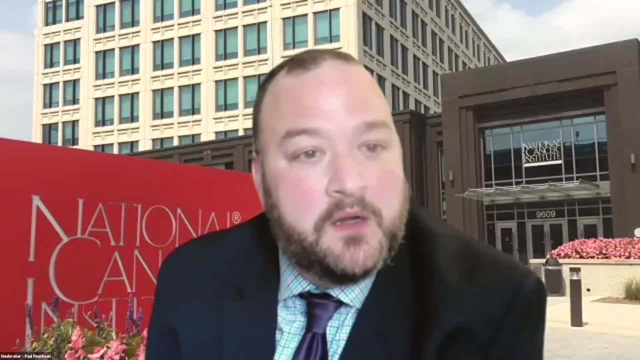 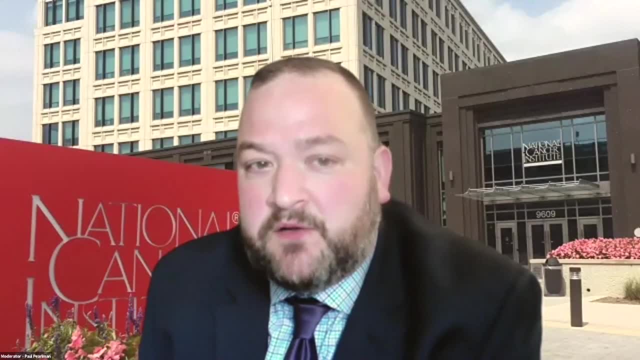 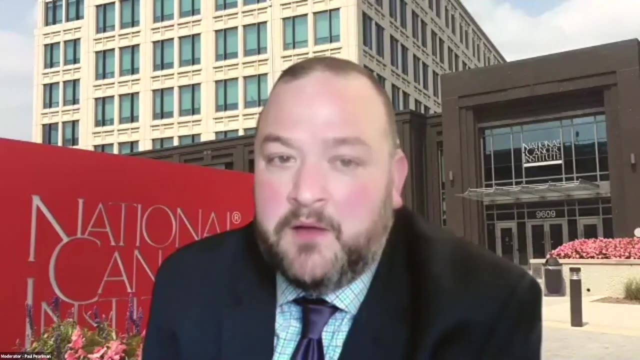 from this point I want to jump into our next question, and that's: it seems so. the question is that it seems that good machine learning predictions can often disagree, and the question is whether any new disease mechanisms or insights have been derived from ML- machine learning predictions that allow. 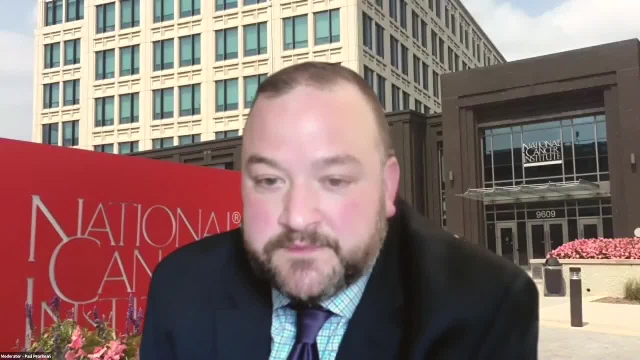 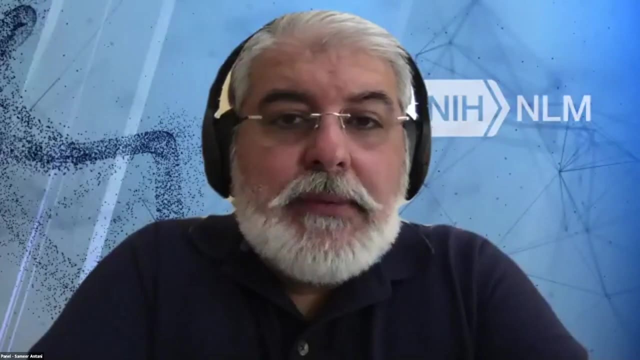 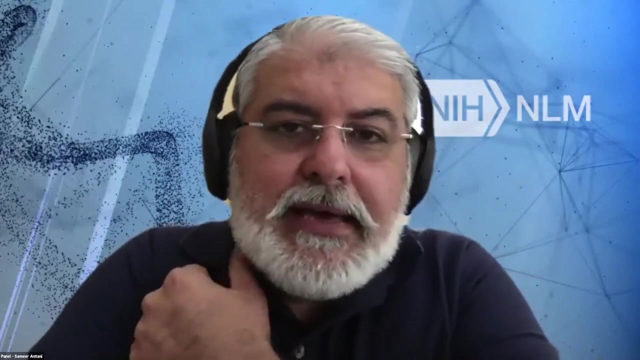 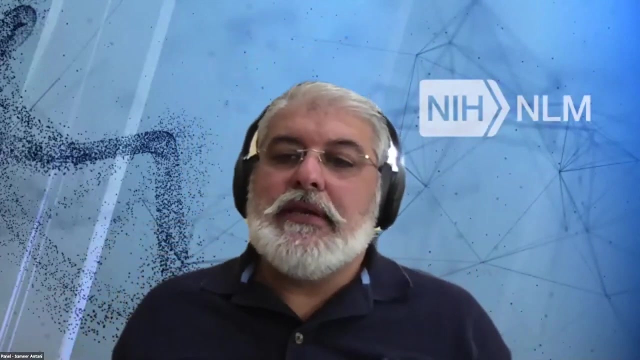 pathologists to assess sort of new ground. true, I can't answer for pathology- dumbing Dan's dropped away, unfortunately- but in a in a in a in the limited experience I have with finding so question is the way I would cast this question is if different ML predictions disagree, is the disagree if? 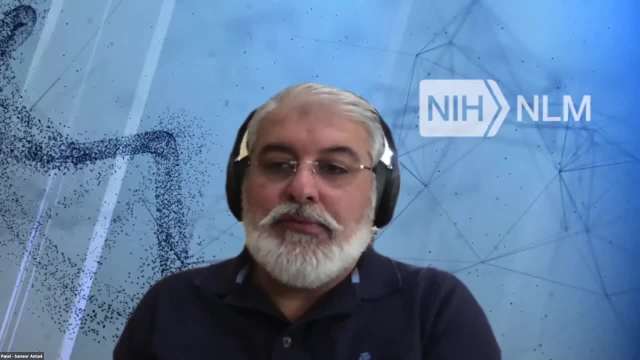 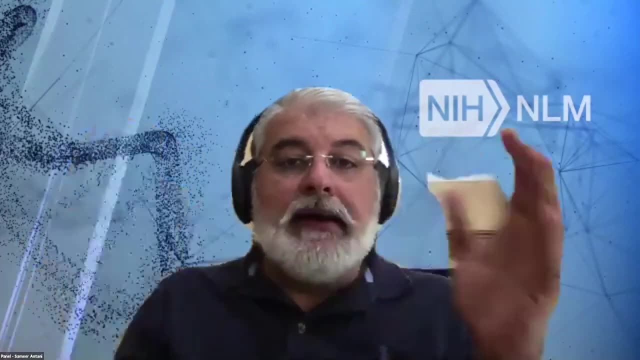 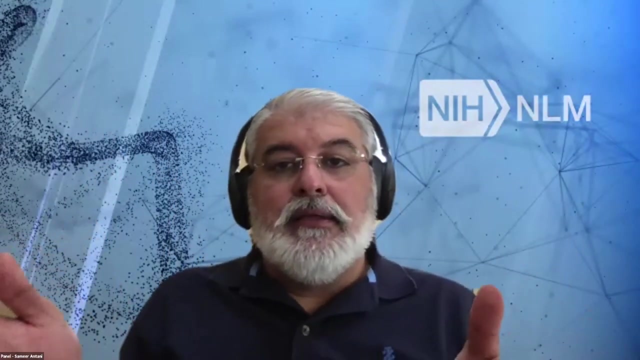 and we agree that what it has found obviously deviates from ground truth. unless a ground truth was, it was a, an aggregate label, so you don't know where the disease is, but that this entire image represents disease somewhere, then the disease is. peut en yuván expert. is could step in and and verify if the 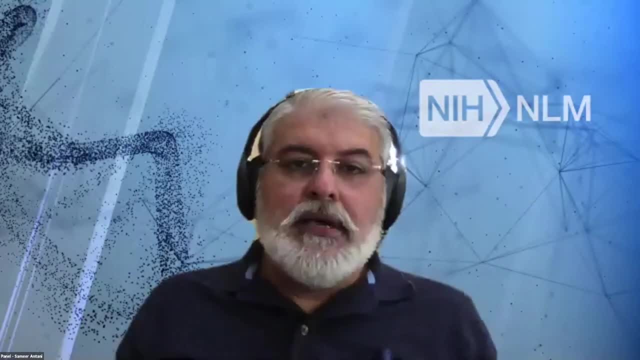 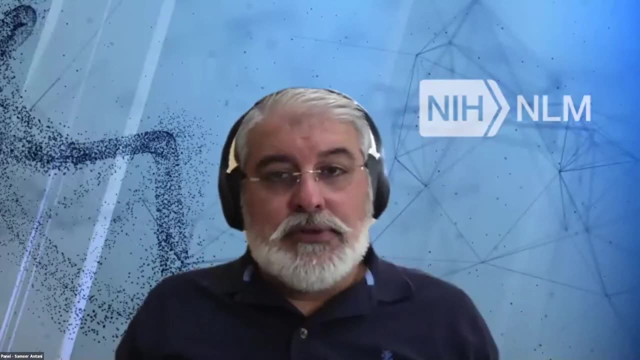 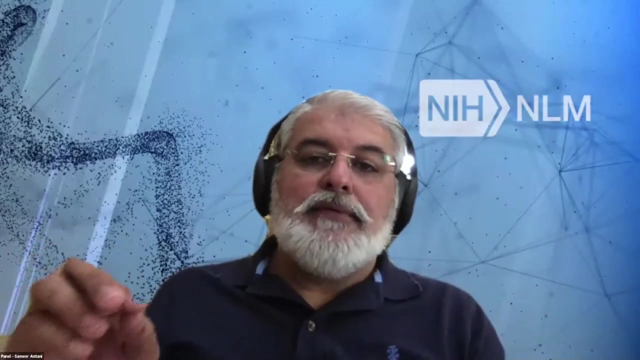 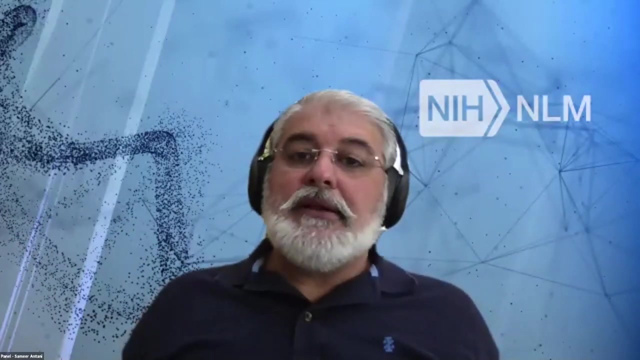 you win. expertise could step in and and verified if the in Suzanne series or in the collaborat vaccine has found some other region that is a surrogate or a or an alias of the true region. is it really a false positive or is it something indeed new? 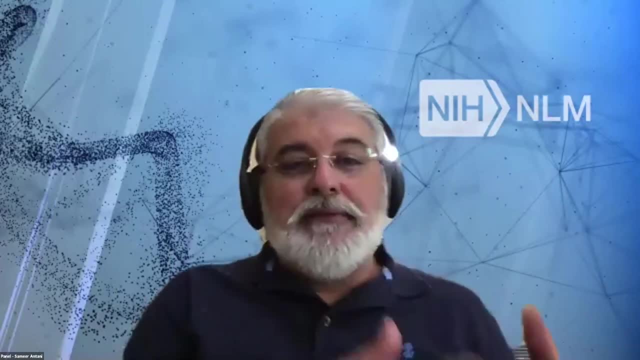 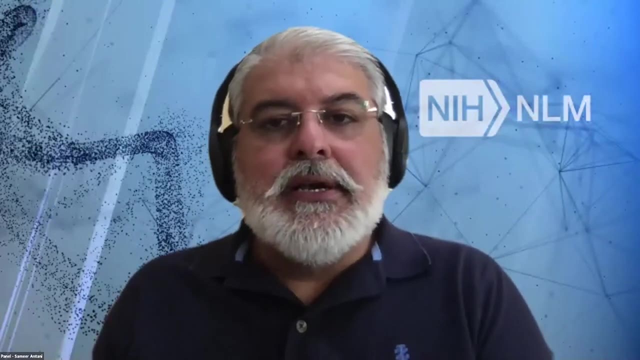 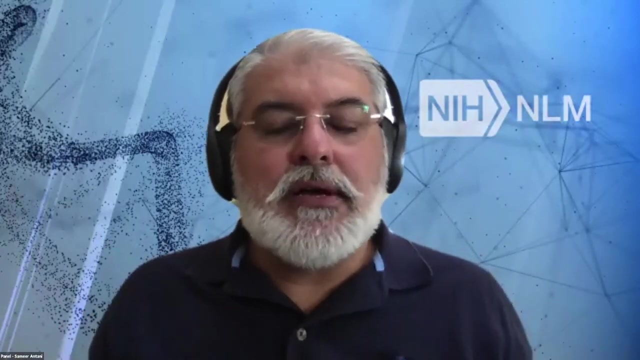 Is it a correlate? And that again goes back to away from computer science and data science into interaction with clinical experts or biomedical experts to see if this is a prevalent condition that is seen widely across the population of data being analyzed, or is it an outlier. 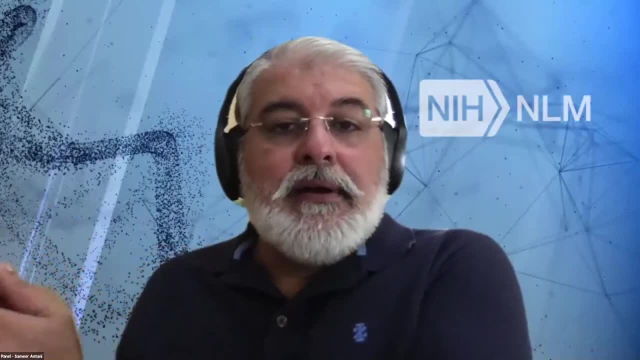 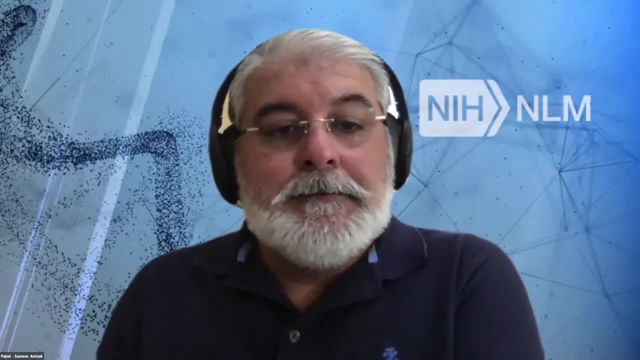 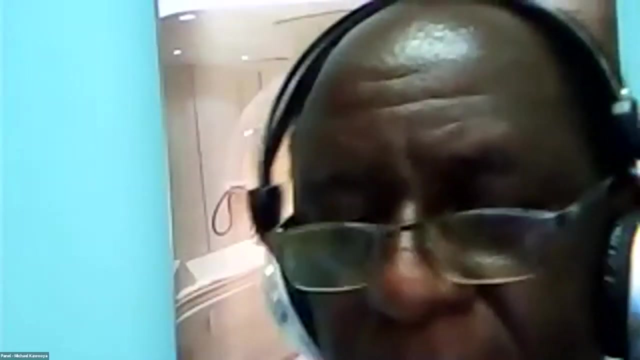 And if it's an outlier, are there other information in other records, other tests that might suggest that this is a meaningful fund? Okay, if I understood the question, in imaging, for instance, there's been a lot of progress with glioblastoma. 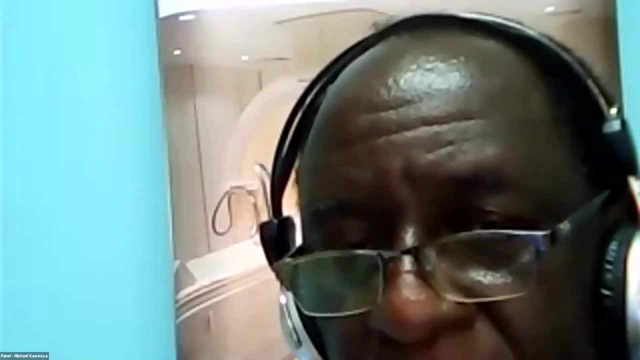 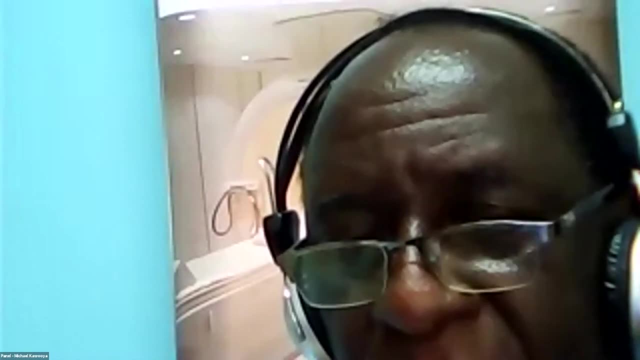 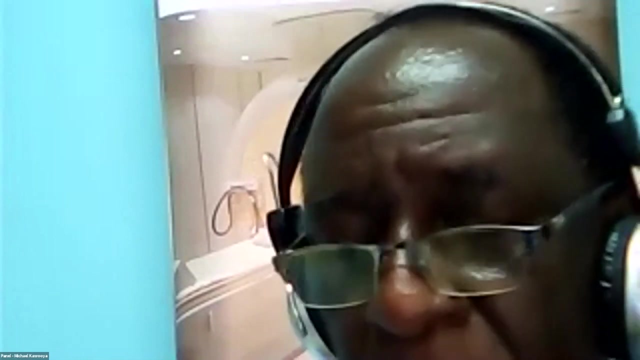 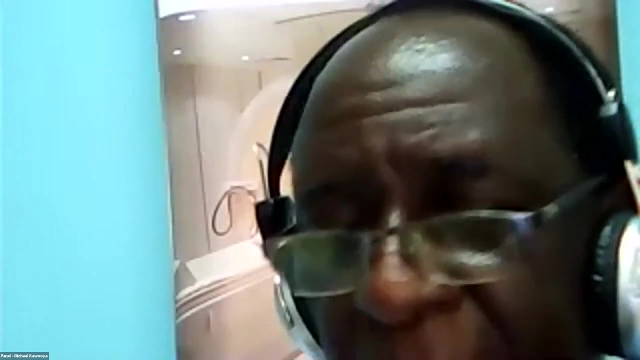 which is a tumor of the brain, in MR, And we see now that MR may help to make a difference between the different type of glioblastomas- the mutant type and the wild type- using machine learning, And the naked eye may not be able to pick those differences. 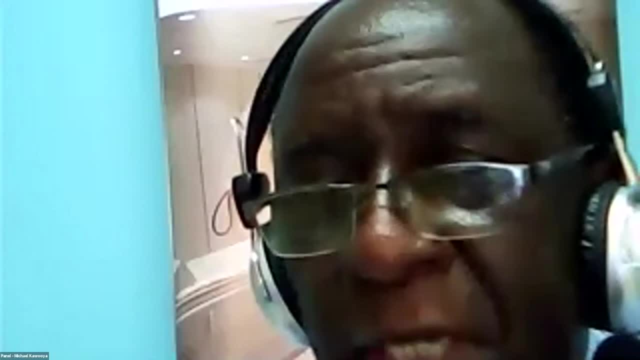 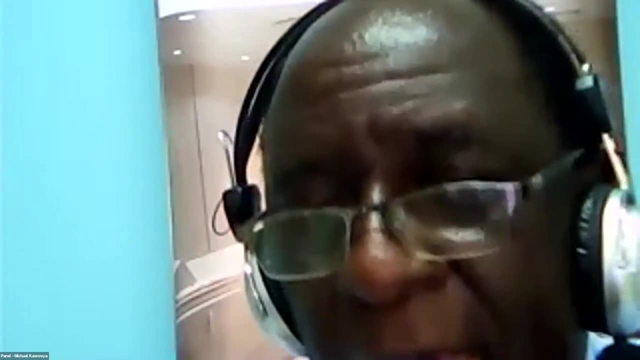 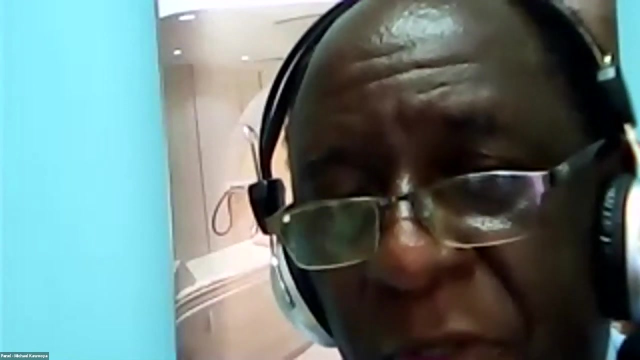 between those mutant varieties. So, in other words, machine learning, artificial intelligence, sees what the eye cannot see, and this correlates very well to biomarkers in molecular imaging, because the biomarkers for the mutant type of glioblastoma are different from the biomarkers. 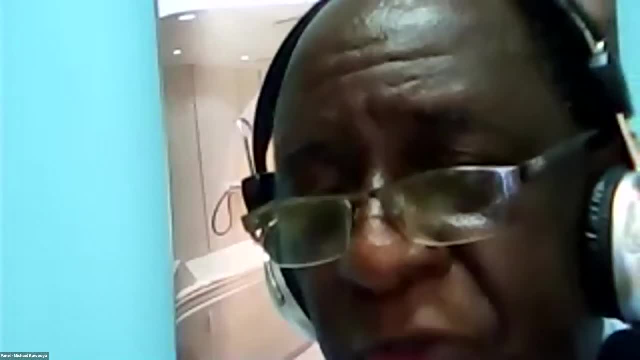 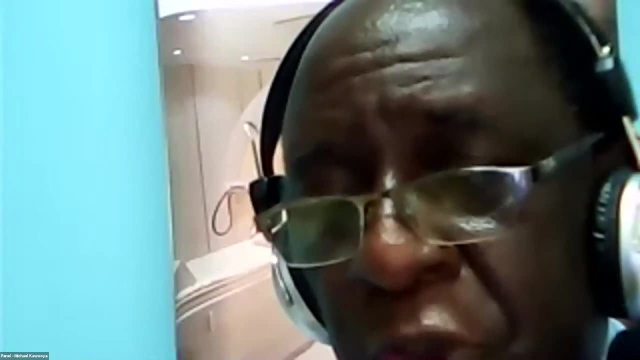 for the wild type of glioblastoma, And artificial intelligence can help us to sort out this, whereas the human eye may not be able to make that difference between these two varieties of glioblastoma. So this is a very important point. 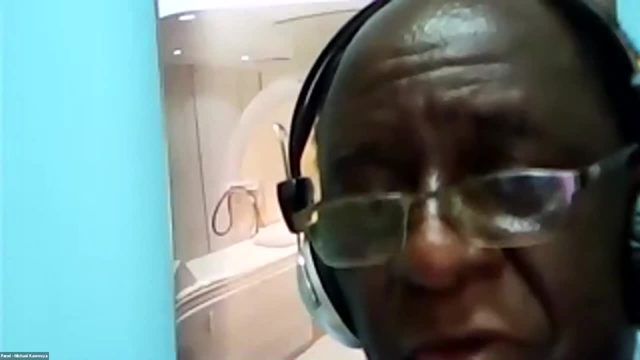 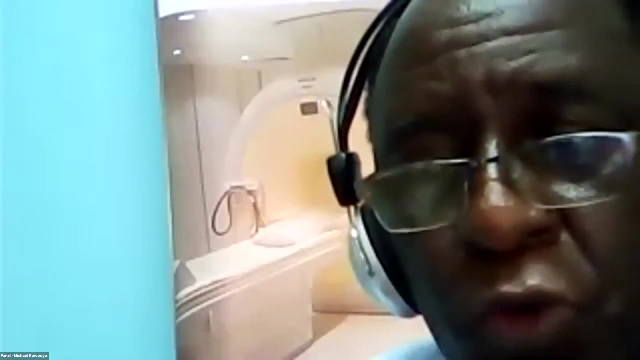 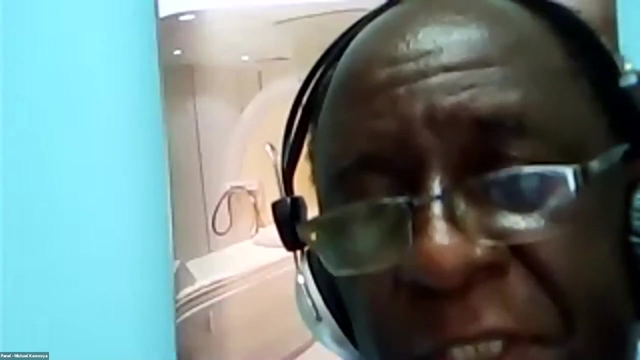 So there are areas where artificial intelligence has gone a long way to see what the eye cannot see and helps us even to be able to predict what the molecular type that may be, whereas the eye cannot predict that. So I've got another question. 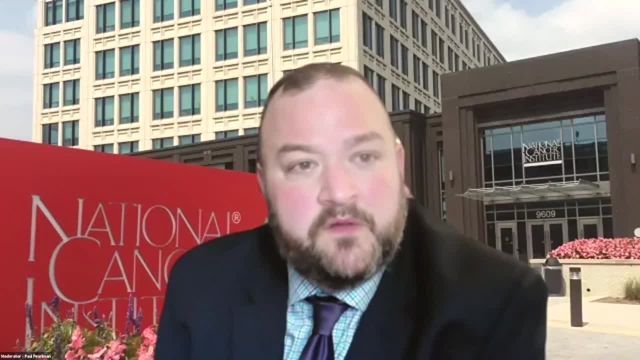 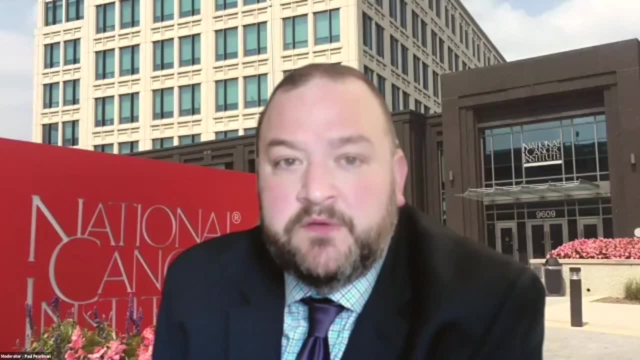 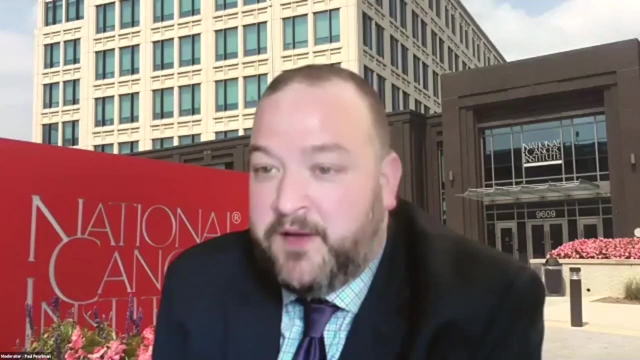 and I wanna start with your view on this, Celia. The question is where individuals can go to learn to build some of these machine learning models, and is there computing capacity in Africa for building and interpreting machine learning and AI solutions? Yes, definitely. 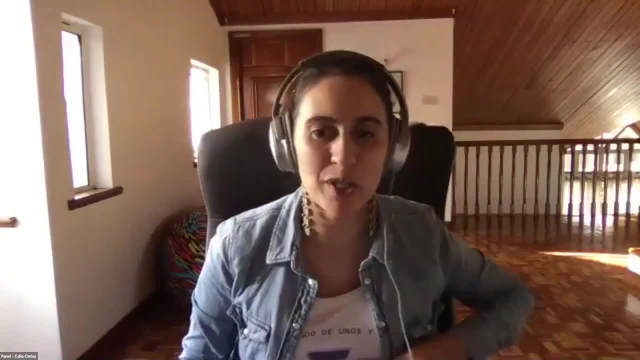 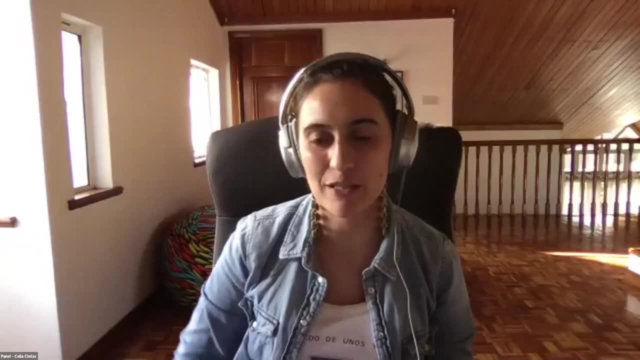 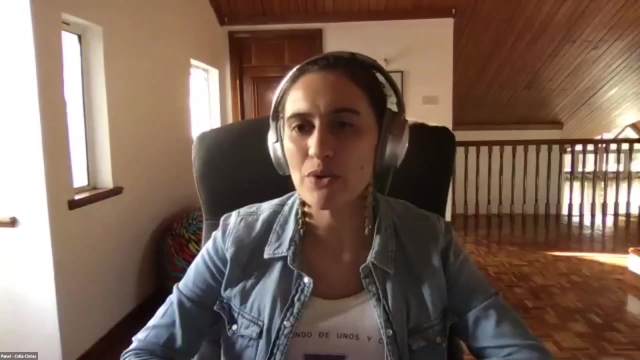 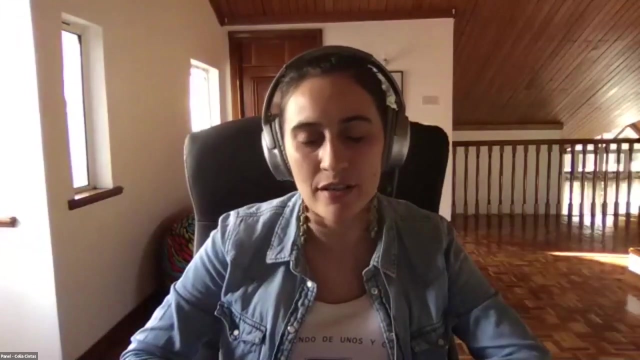 So our lab has a stronger relationship with the School of Engineering in CMU in Rwanda. We always have great master's students from the university, so I will definitely recommend those programs. IBM also hosts several courses with machine learning basics, also blockchain and other similar topics. 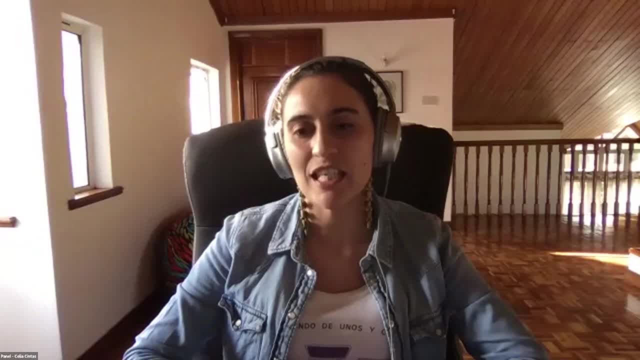 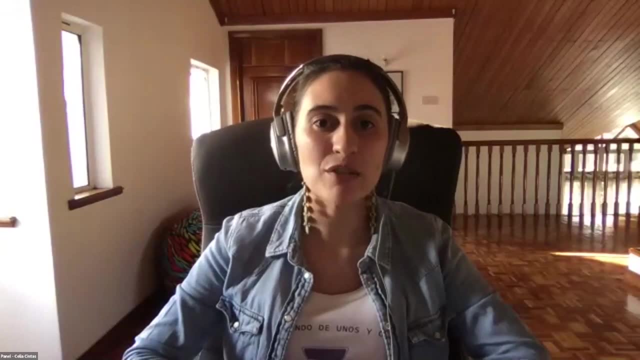 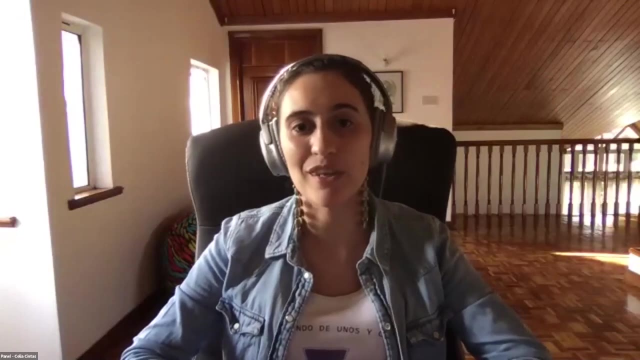 Hopefully. year by year we see that all these models are being able to run in cheaper and cheaper hardware, So this is great for everyone that doesn't have access to big, big clusters and so on, that can still with a few notebooks or a small CPU. 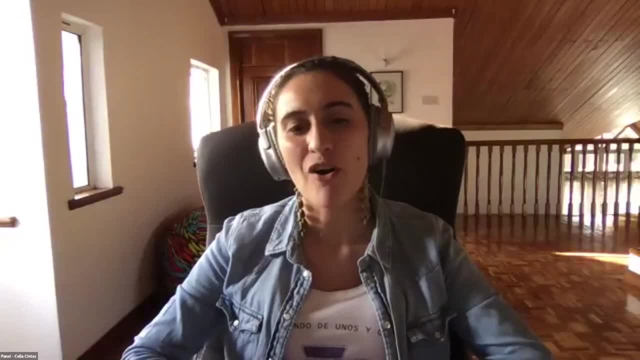 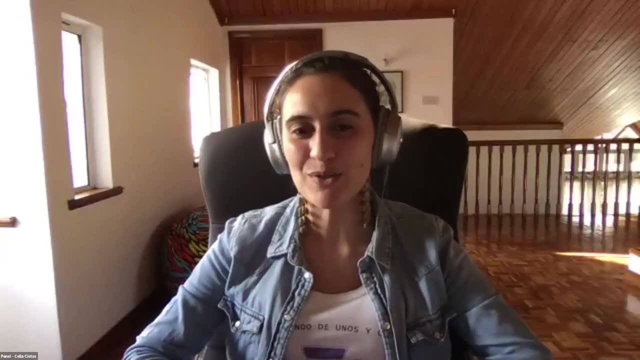 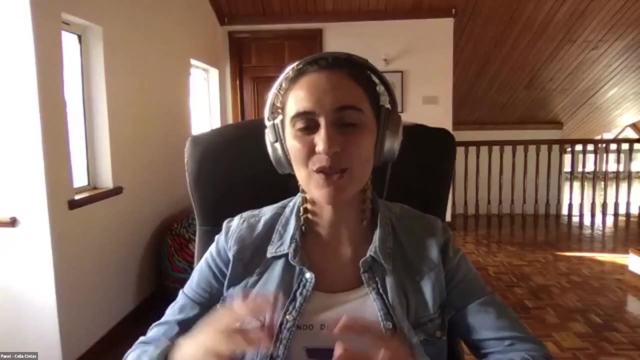 they can still run experiments. Also, all the pre-trained models that we can access, all those neural networks are being running for weeks and weeks in millions of millions of samples and we get those fine-tuned matrices values in our computer with zero computation cost. 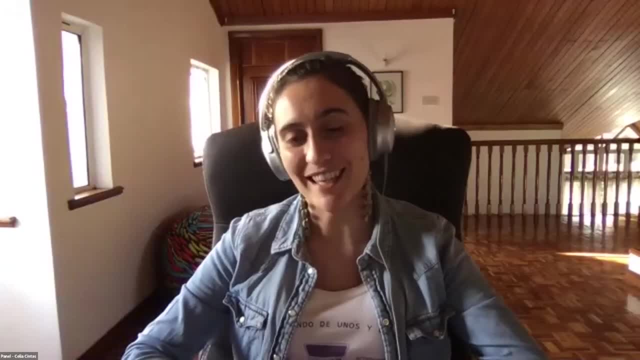 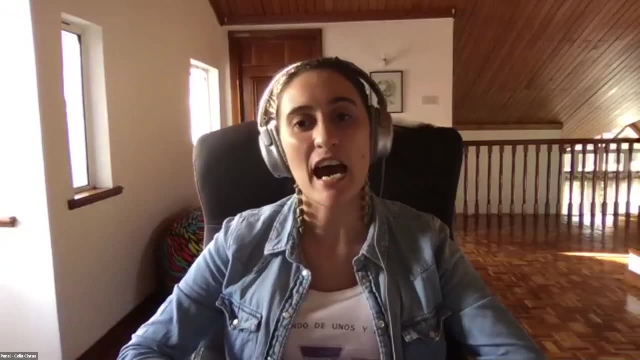 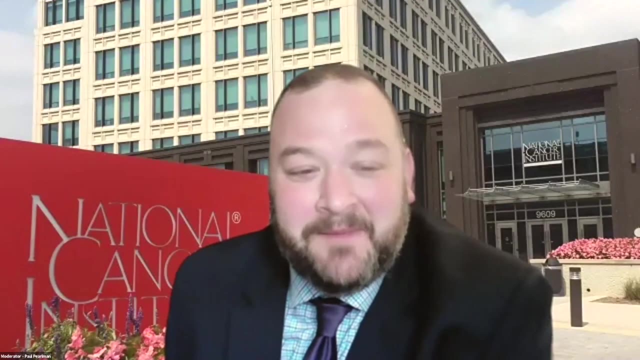 And usually we will train with the smaller data sets. So I will say yes, for small runs, of course, we have the capacity, and for bigger, of course, we have the cloud, Thank you. So I'm gonna ask one last question. 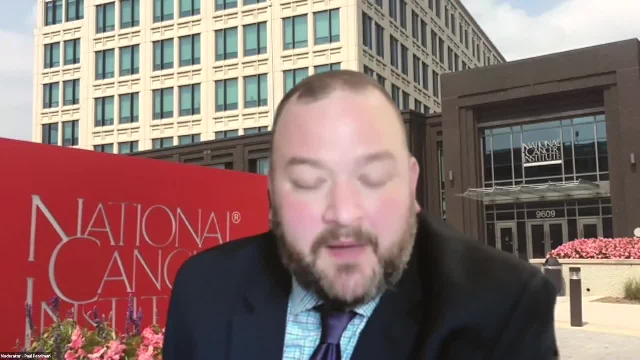 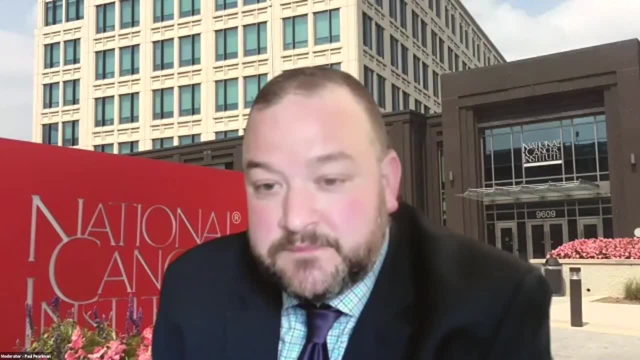 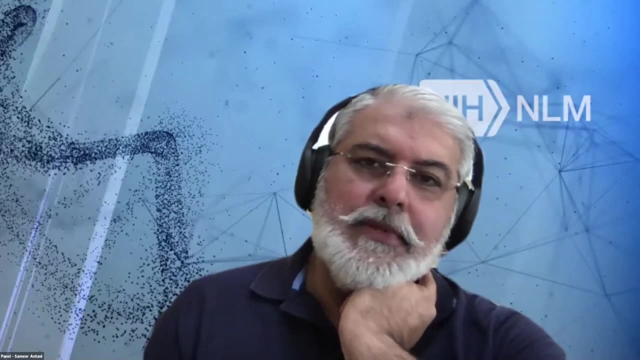 and it's. the question is why, by and large, are many of these machine learning and AI tools not yet being used in clinical settings? That's a tough one to answer, because a lot is, I think, in between technology. 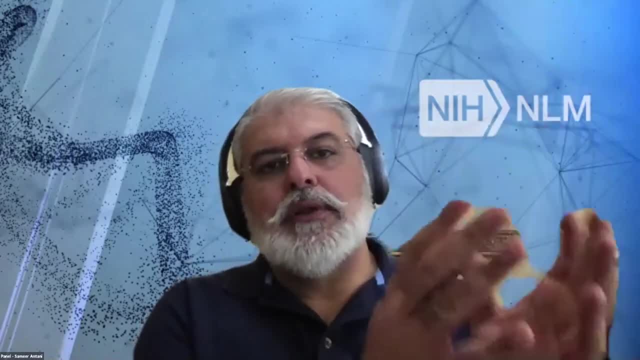 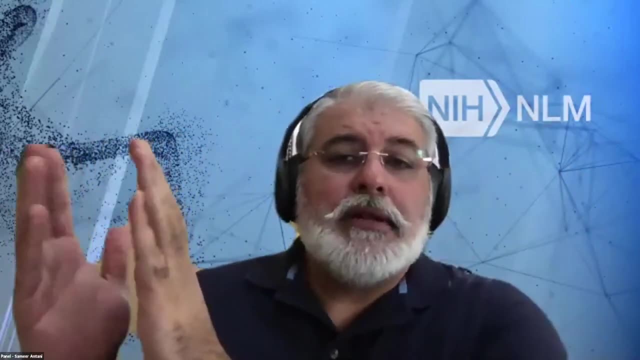 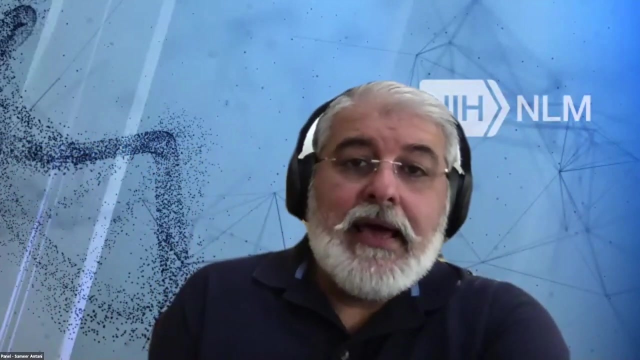 that is, the developing a machine learning tool, developing even, say, a product to it, fitting into a particular clinical protocol. There are many steps and they include approval from, in the US, the FDA or appropriate health ministries agencies. 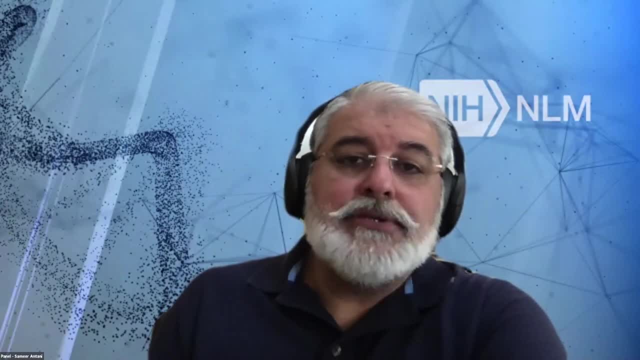 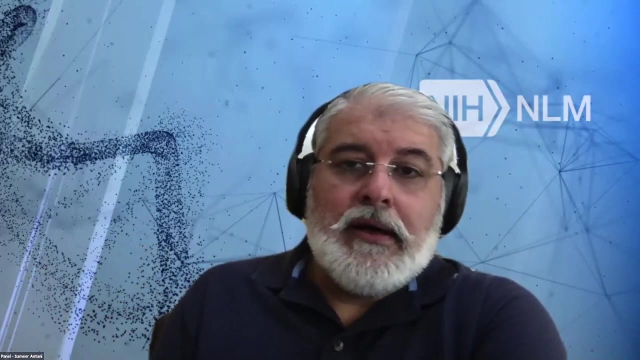 in respective countries acceptance by the community of how they would translate results from a machine learning model to clinical practice. Is it merely a classification score or is it a prediction of risk to the patient that would suggest an appropriate intervention for, say, the right? member of the community. 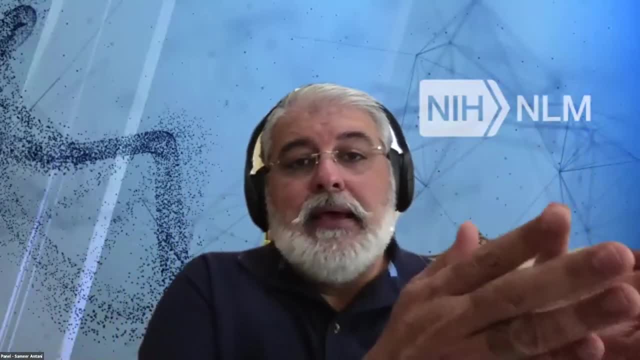 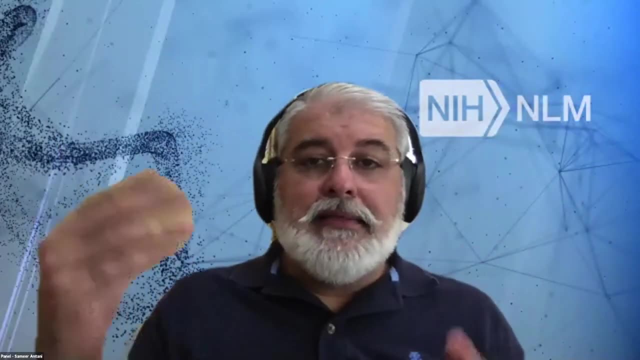 Is it, for example, from a pathology standpoint? it might be as naive as highlighting regions to look at, which, of course, reduces the time, And there is a performance metric there- and but the if you skew away from missing any cases. 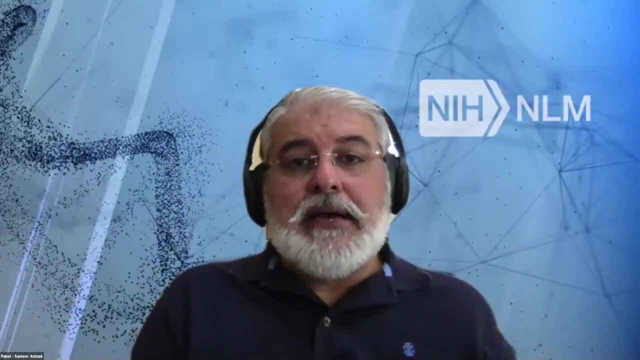 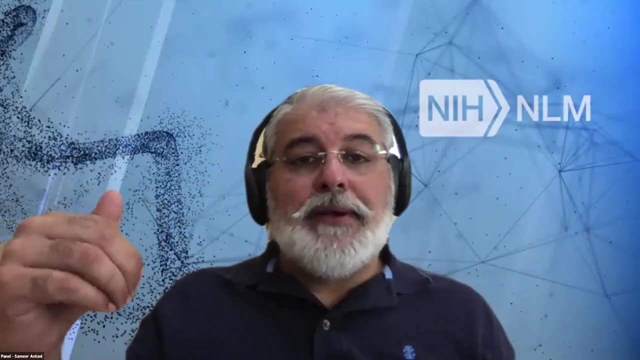 you allow false positives. You still have saved time, but you will not risk losing the patient. However, intervening from a surgical standpoint, when the patient doesn't need to be intervened or you are in the midst of a surgery, you can imagine a live system as an AI system. 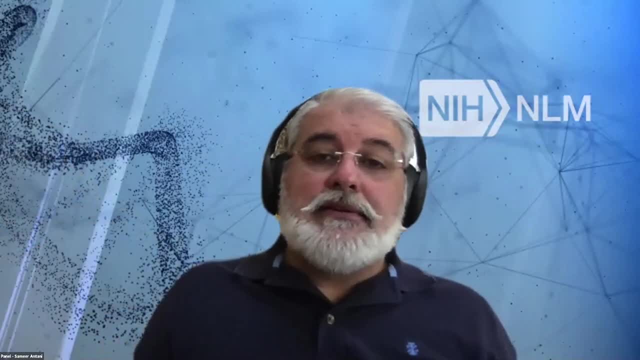 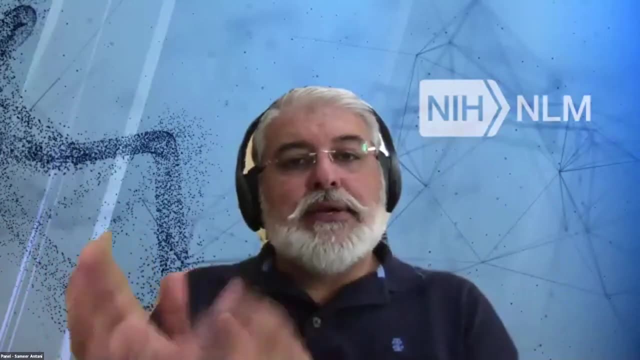 that is serving as a guide and you have an unnecessary decision. Now the risk is much greater. So there are several factors that play into it, that mostly allude to risk approvals and acceptance by the community and other factors. 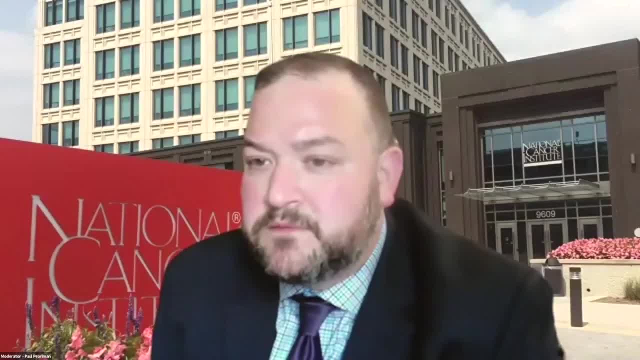 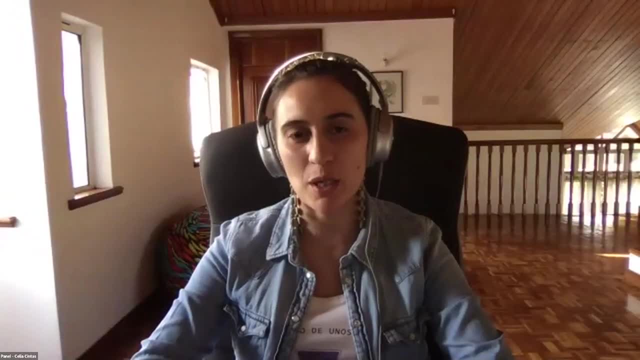 Anyone else want to add to that? Yes, I think for a machine learning perspective in clinical settings, I think we will get to the point to help professionals to make decisions, But currently we cannot allow machine learning models to make their own decisions. 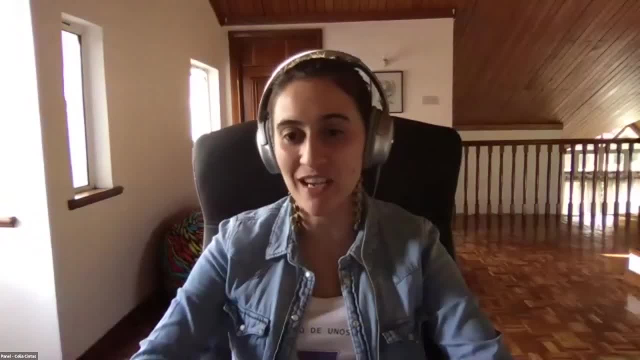 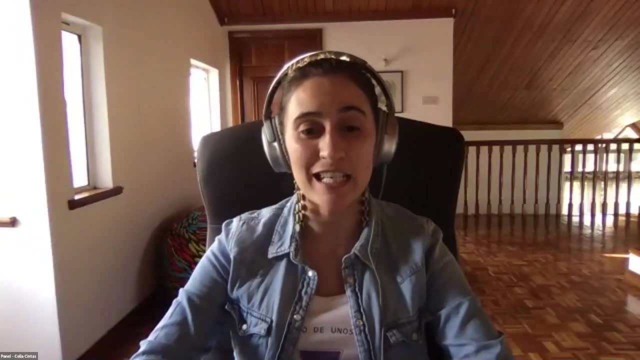 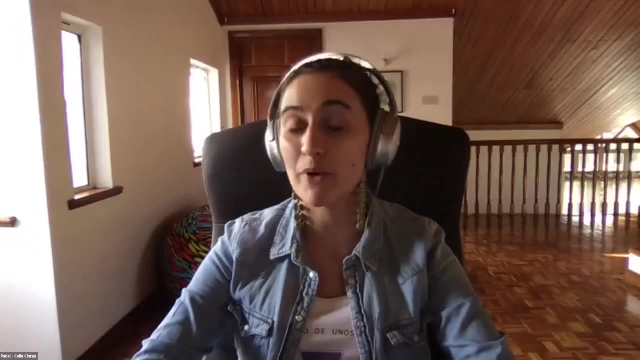 as we don't have clear transparency on how the decisions are being happening or over under what population this model was trained And given the, I think that health is such a critical thing. We can hope for these type of models to assist professionals to see different patterns. 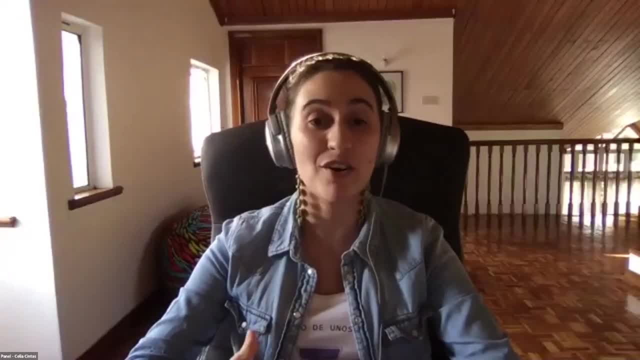 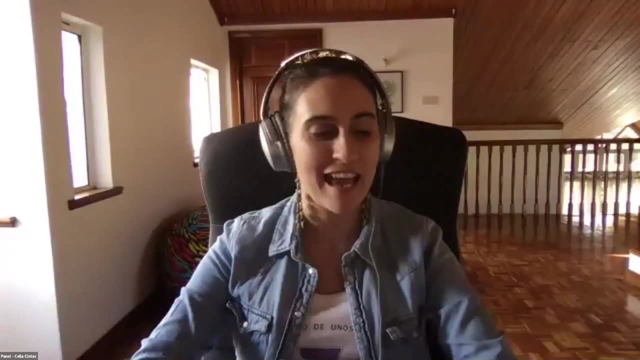 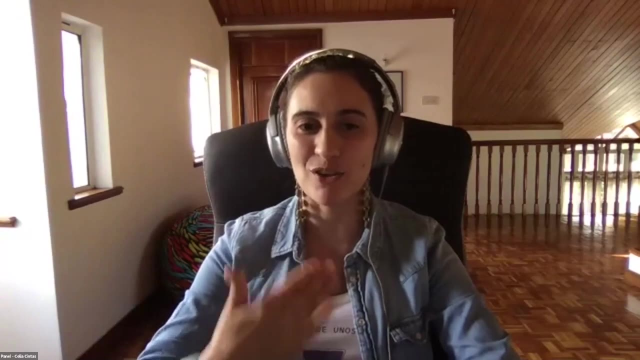 that maybe they wouldn't have access to or see other second opinions. let's call for machine learning models. I think that is going to be more liable. but as any other process here in Kenya, you need a Cranberry approvals, you need to go over a process of ethical 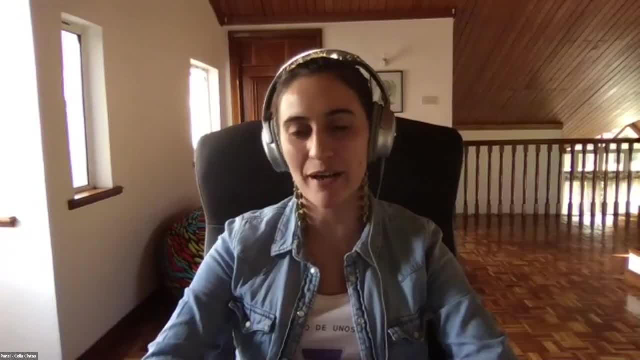 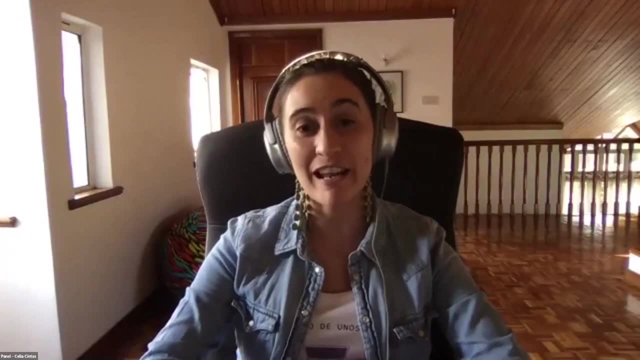 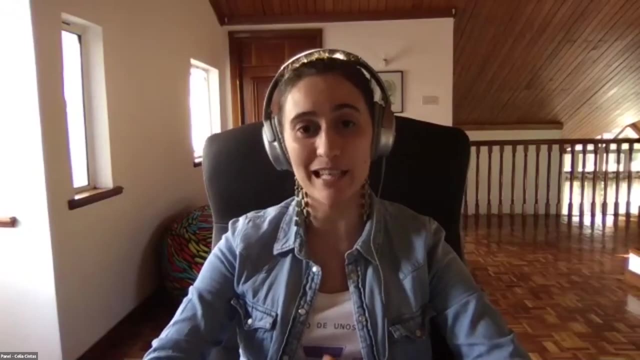 consult to see that you are compelling to everything, as any product, as anything that gets to a clinical environment. There are a lot of regulations and we need that the models that we deployed are being transparent and know the limits of their support. So I think I'll 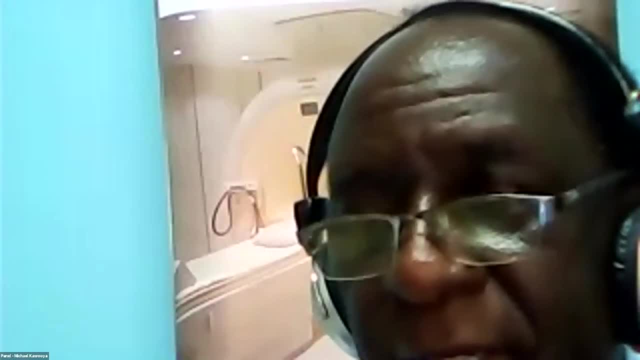 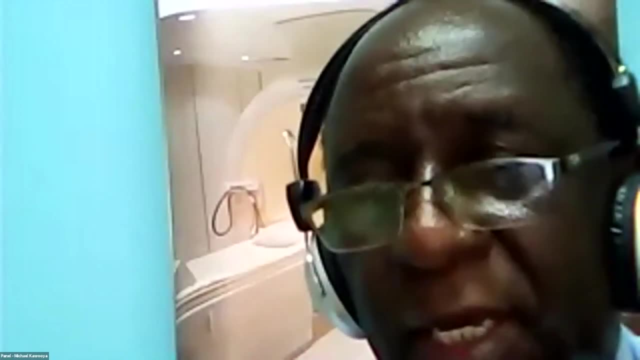 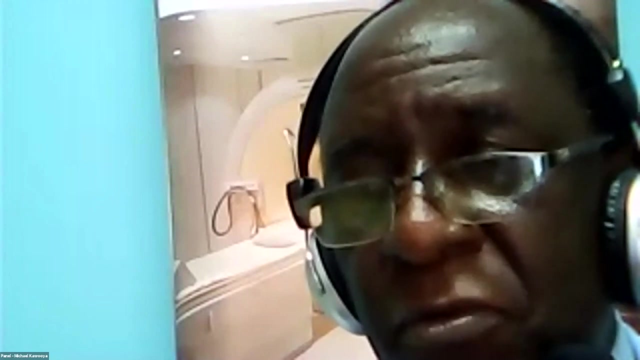 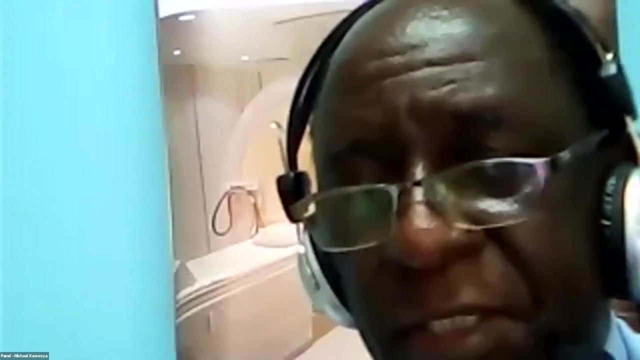 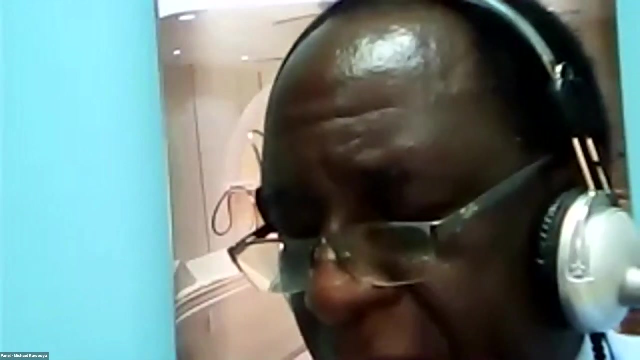 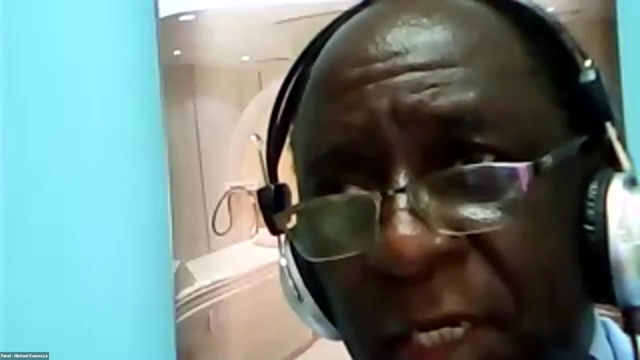 I also want to add that the The. So I think that training is important. And then, secondly, it's also the relevance: If it does not address a clinical challenge, a clinical problem which I encounter every day, then I'm not likely to use it. 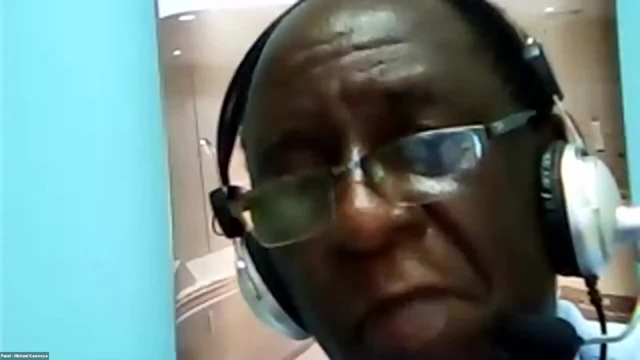 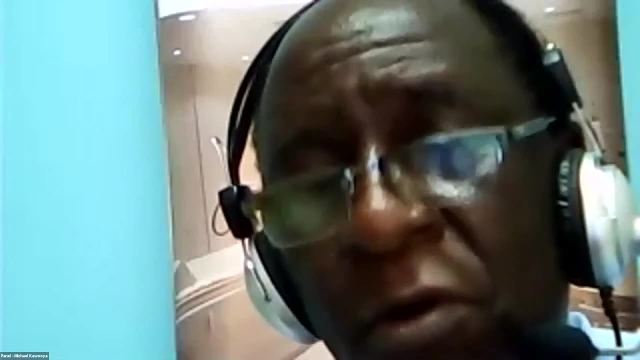 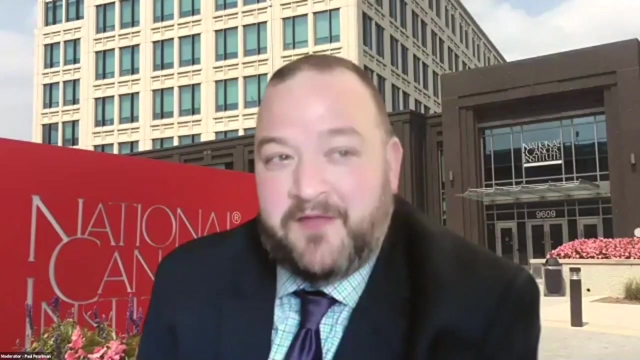 But if it addresses, if it's relevant to my setting, my healthcare setting, then I'll take that up, Plus, of course, the ethical legal implications, as already noted. Yeah, I guess I would take the risk, as a moderator, of adding a thought as well. 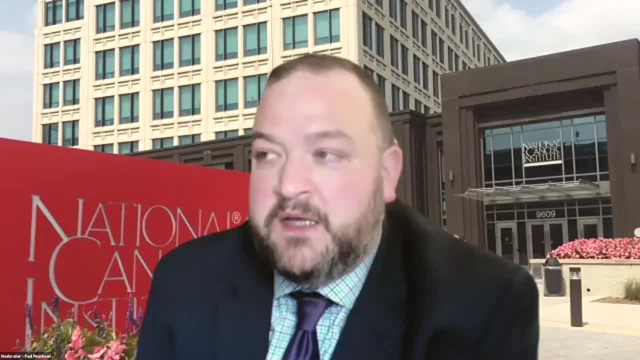 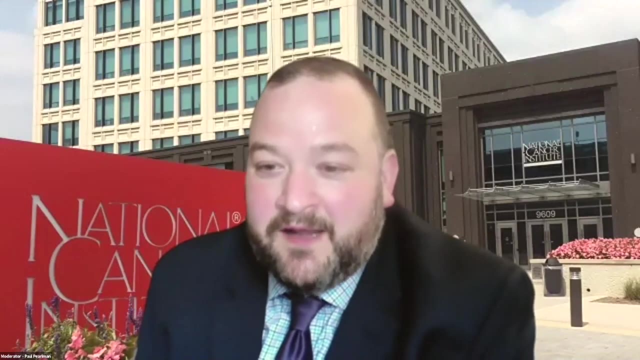 And that's That the regulatory science is really developing in parallel, And only recently have we seen sort of machine learning and AI-specific regulatory pipelines from our FDA, And so a lot of this is still happening in real time. With that said, we are out of time for new questions. 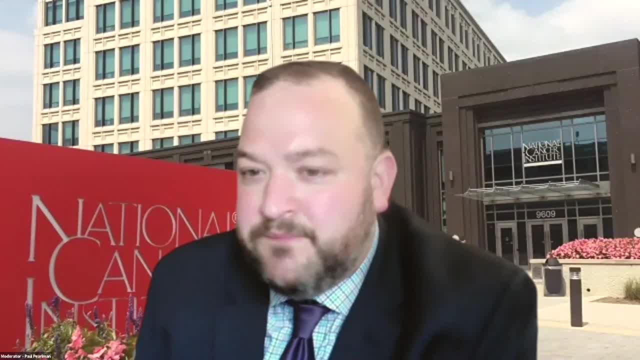 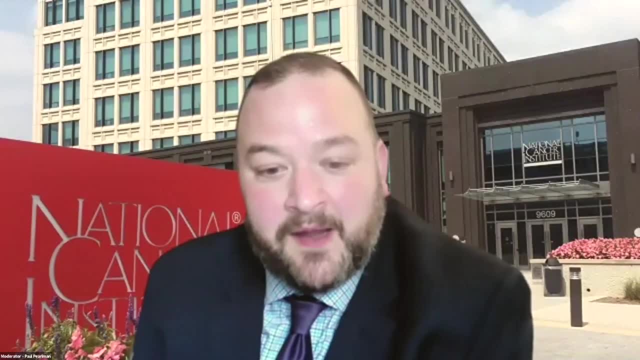 I want to invite each of the remaining speakers to maybe add a final thought, if you have one, on the session as a whole before I turn it back over to Maggie. Well, I think I'll quickly end the silence there. I think this was a wonderful session. 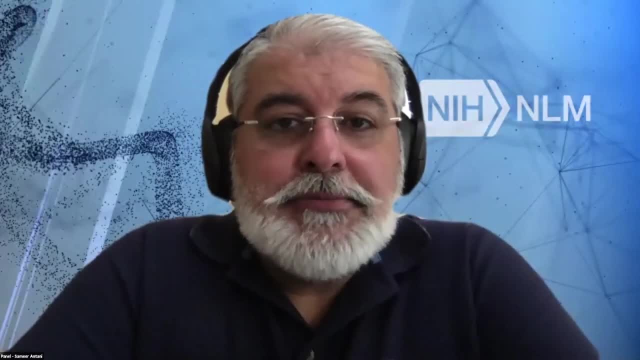 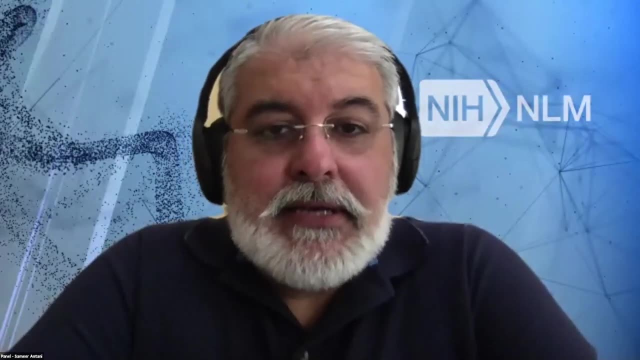 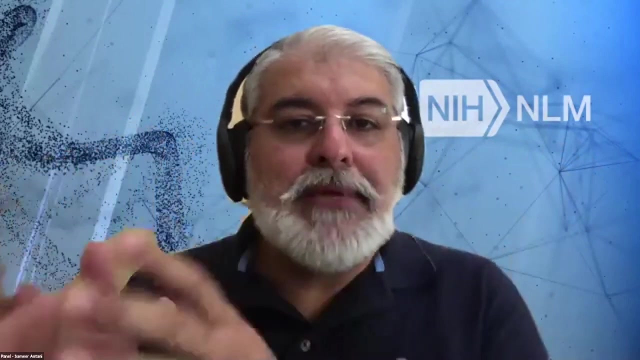 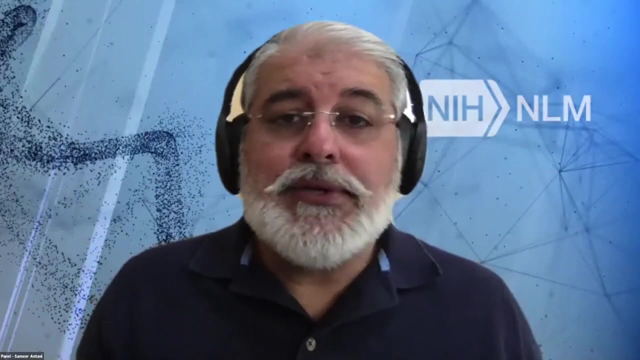 I particularly enjoyed it because it provided a broad spectrum of opportunities, challenges, close interaction between data and design, the bridge between computational sciences and biomedical sciences, toward improving patient care overall. That is our ultimate goal And there are many steps toward that, which are broadly data science. 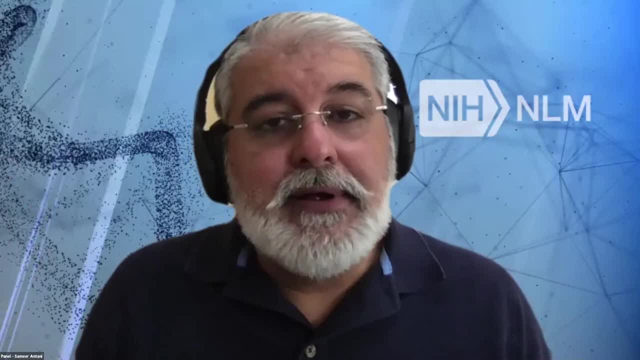 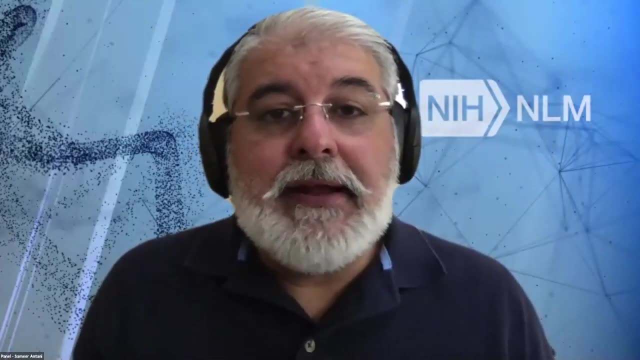 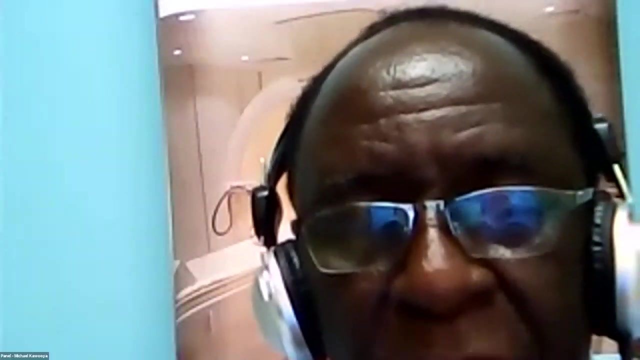 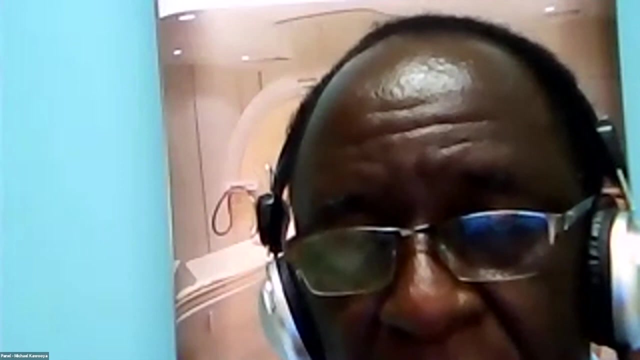 So I hope that the attendees have been inspired and the opportunities that NIH is providing would be taken advantage of over time. say that, yes, we have embarked on the process to bridge the gap between the high and low and middle income countries with regard to data science application. It's a small, fast. 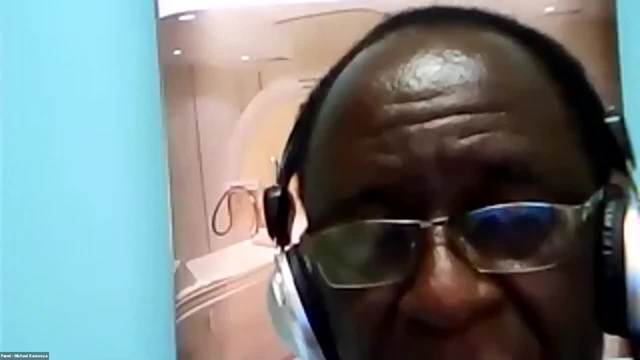 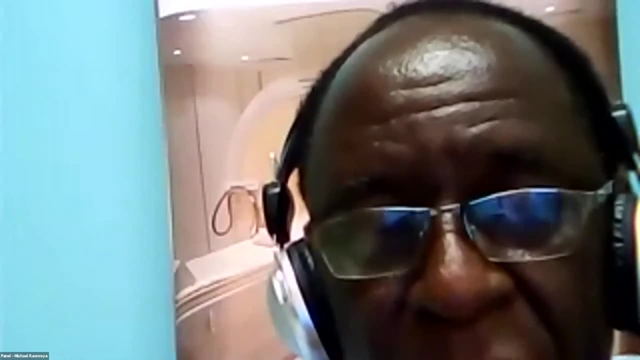 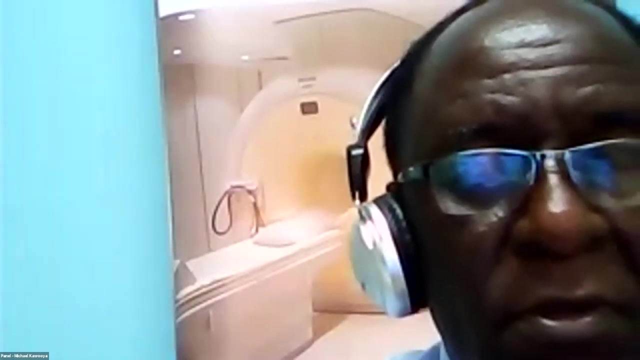 baby step, but I think it's a very important baby step and we should have as many people on board, as much collaboration as possible, to make sure that this works this very fast baby step really works. Some closing remarks on my side. Thank you very much. The panel was super interesting. 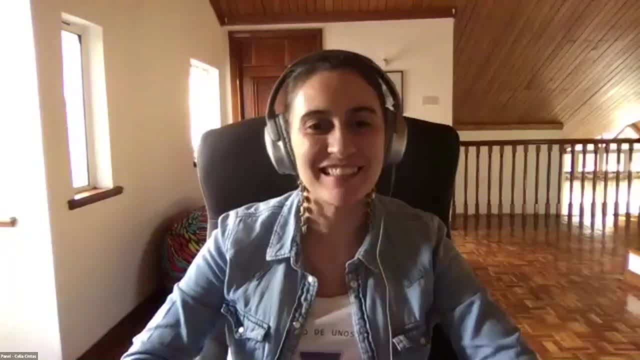 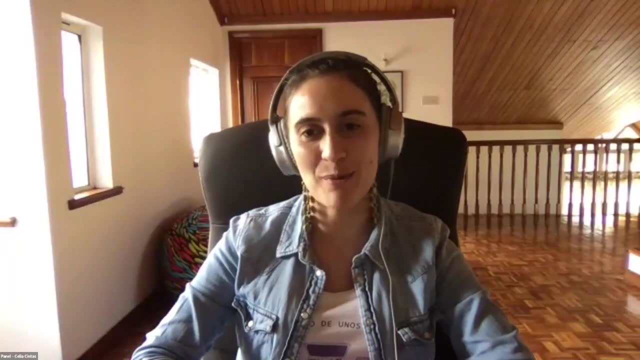 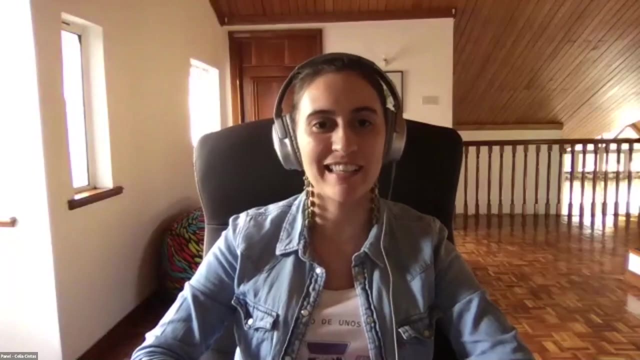 I learned a lot too. Something that I will very highlight and reinforce is: all these machine learning solutions are done with the main experts side by side. As computer scientists, we cannot sit alone in a lab, get a bunch of data, mash it together. 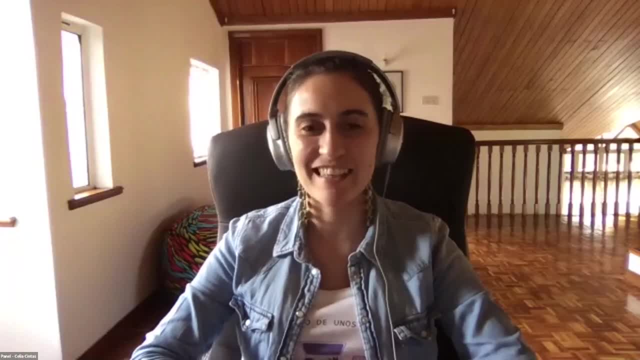 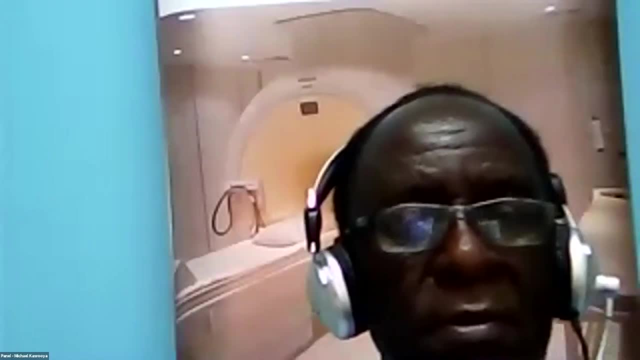 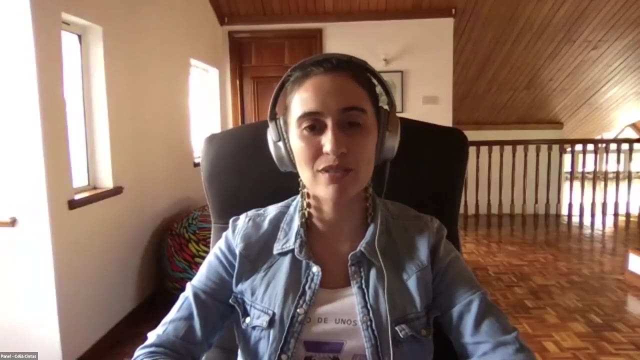 To a deep learning model and publish that. that is not sufficient. We always need a domain expert showing us new patterns on the data, or new patterns even on the insights of the models. So my highest recommendation was always to work with the main experts in any problem. 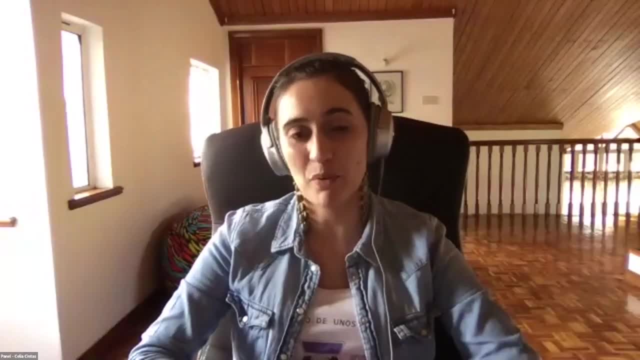 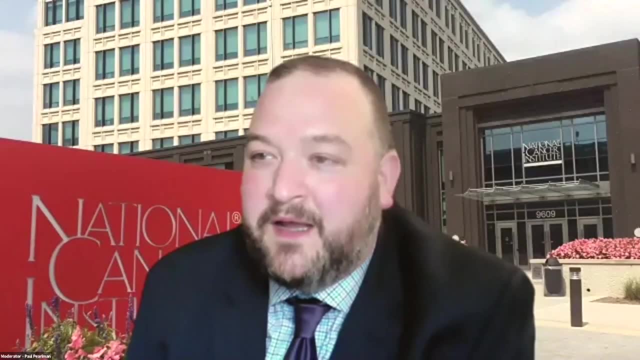 that you're trying to solve And especially with the community that you're working on for sure. So I want to thank our speaker, Thank you. I want to thank our speakers again And I want to thank our attendees as well. We had 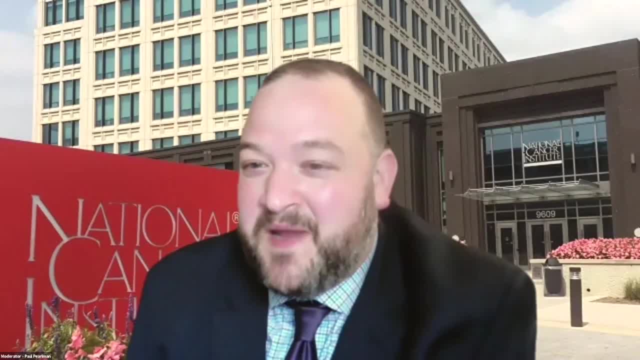 well over 100 participants in this session, So I think there would be a booming round of applause happening right now if we weren't virtual. And, with that said, I hope to see all of you in the networking lounge And I'm going to hand it off to Maggie, who will explain. 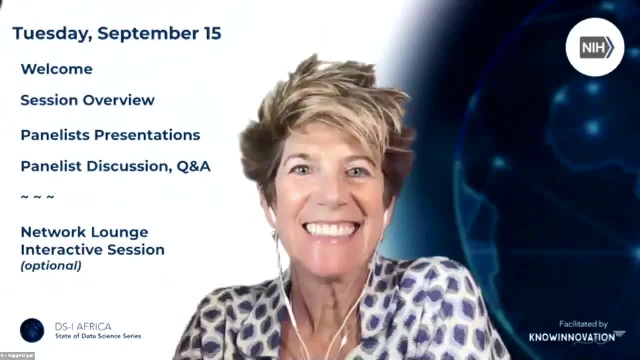 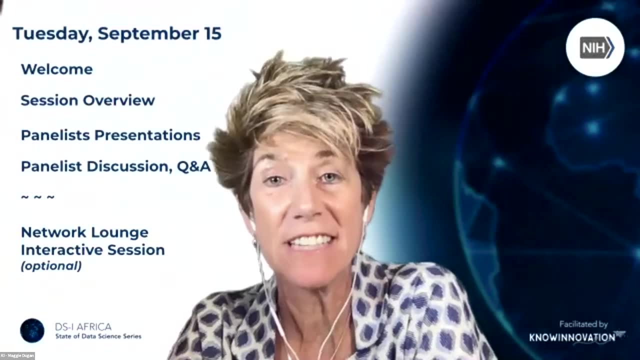 how to get there Exactly. Yes, we have come to the end of this webinar, but we are not necessarily finished. You are invited to continue the conversation by joining us. Thank you for joining the interactive networking session in the network lounge, And I am going. 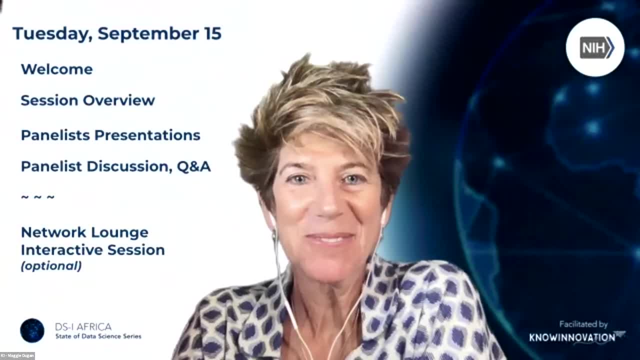 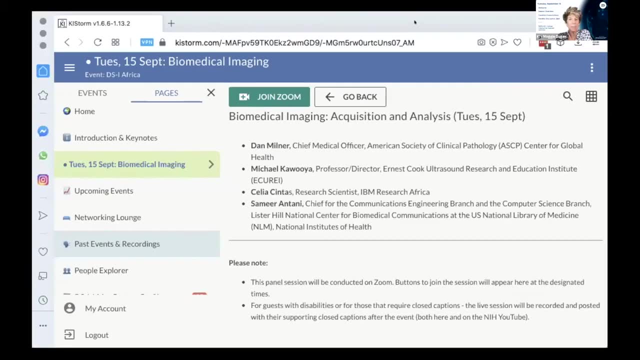 to give you a little demo of how to get there. So I am going to imagine that you are probably. if you go back to KaiStorm, I would imagine you're on this page. This is today's page for this session. This was the Zoom button that you joined to get here, And if you just 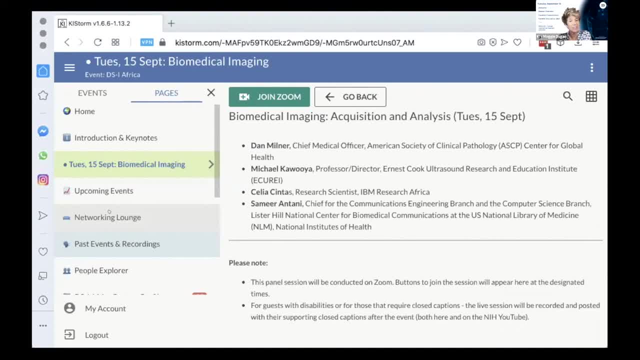 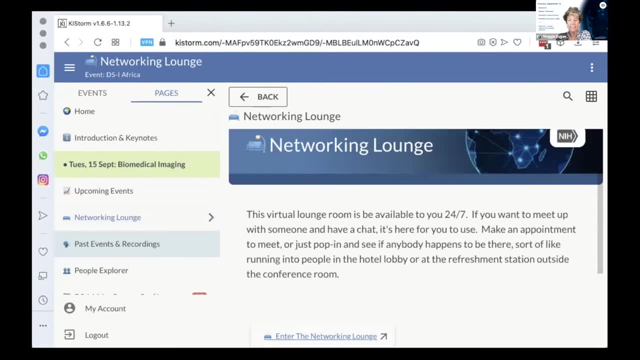 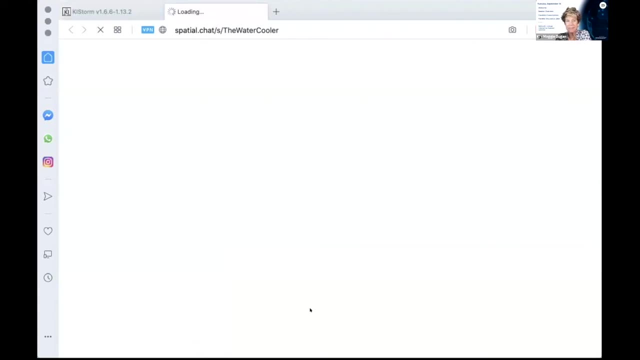 go down one, two pages, you'll see the networking lounge. That's where we invite you to go after you leave here And when you come into here you will see that there is a button to enter the networking lounge. It will take you into another interface called spatial chat. You. 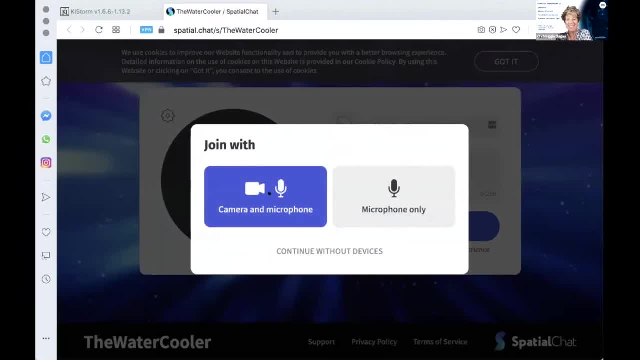 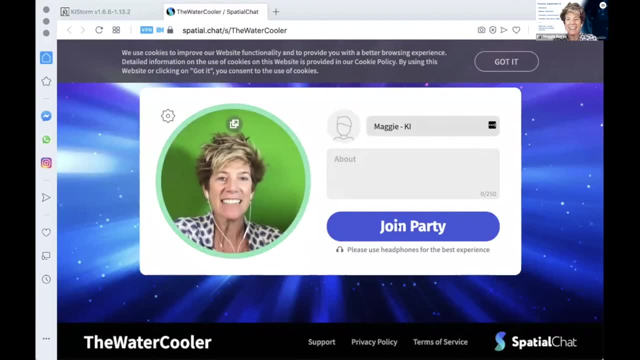 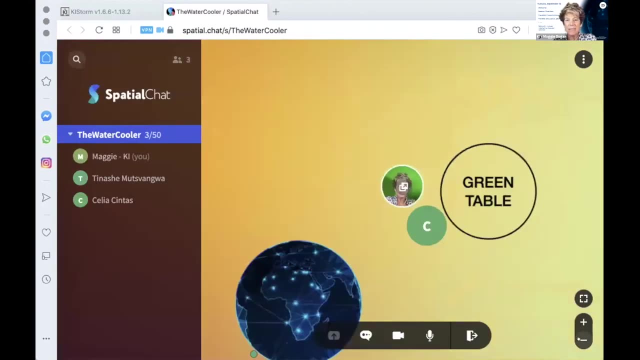 can choose for your camera and microphone. I would encourage you to do that. You can do microphone only if you want, but it's nice to do the camera as well. You type in your name here and then you can join the party And then you see that you are in the lounge, If you hit the little negative sign here. 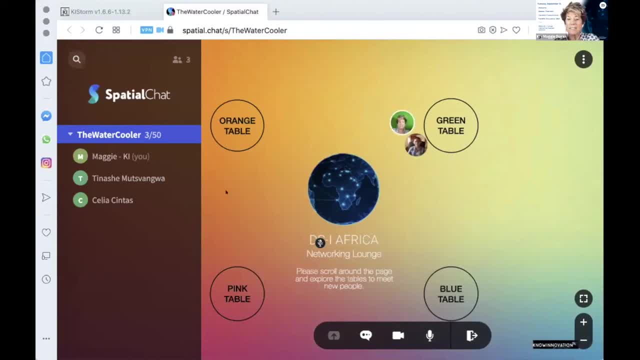 it will make the screen change for you, So you can see that there are several tables. You can also see who else is here. Got a couple of other people here with us already, And what we've asked our panelists to do is to place themselves at tables. So Samir is going. 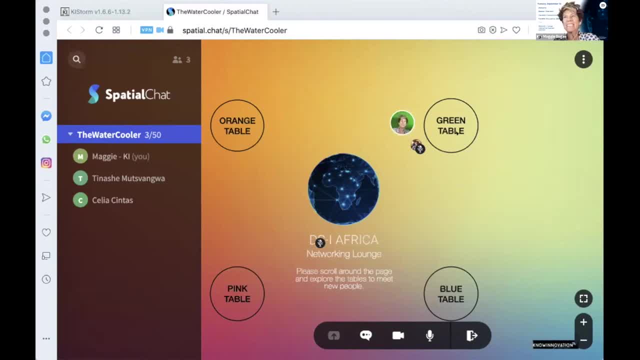 to be at the orange table, Celia will be at the green table, Dan will be at the pink table- we hope- and Michael at the blue table. We'll have some other people in there. You can see them, And what happens is, if you move your avatar close to someone else, you can see them and 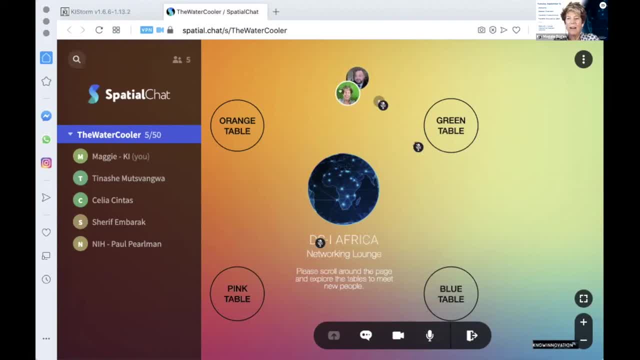 then you can hear them, And if you move away then you can't. So you can have conversations and you can go to different tables and check with different people. So that is how you will get to the network lounge. But before you go there, I just have a couple of other. 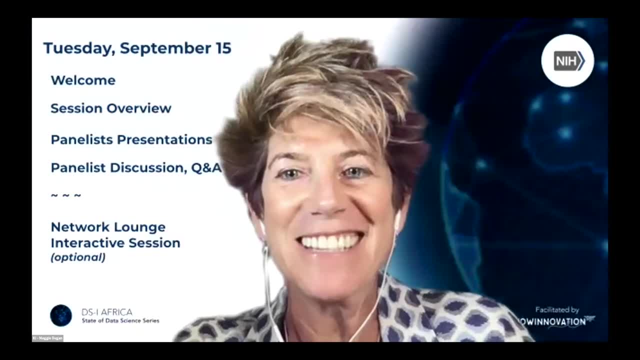 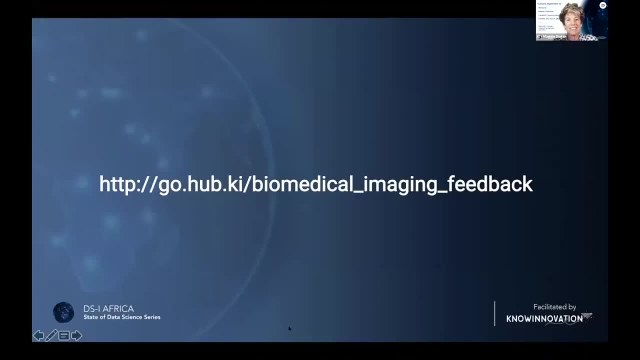 things I would like to share with you that are important information for you to know. First of all, we're really interested in your feedback on today's session, So in the chat we'll put this link as well so that you can easily click on it. But we invite 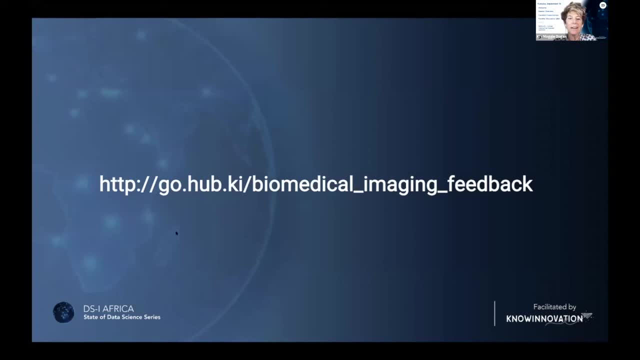 you to just do this very quick survey to let us know how today's session went for you. I want to remind you about the hashtags. If you think that there was something interesting that came out of the day that you want to talk about in social media, we encourage you. 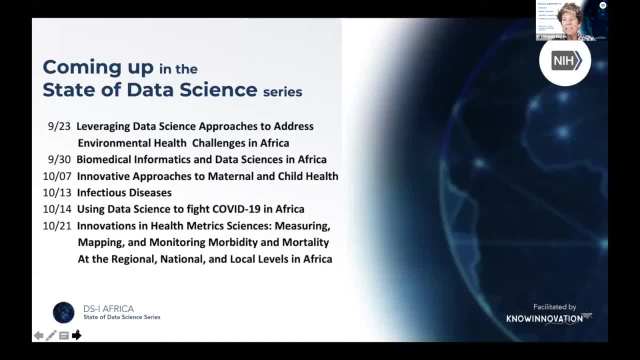 to use these hashtags. There are some more series coming up for the state of data session. Thank you, Thank you everyone. Thank you everyone, Thank you. We'll get to the next one, which is the data science series. Next week we have one on. 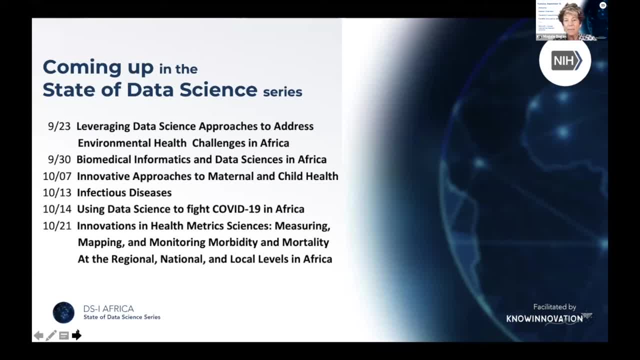 leveraging data science approaches to address environmental health challenges in Africa. Following on, we have biomedical informatics, maternal and child health care The following week. the next week we have two infectious diseases and using data science to fight COVID-19 and then later on, the 21st health metrics. So we encourage you to put those in your calendar. 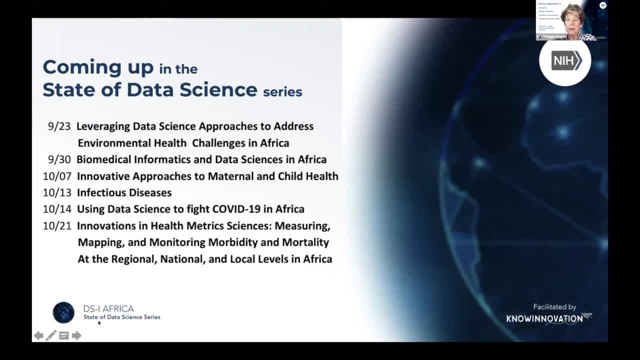 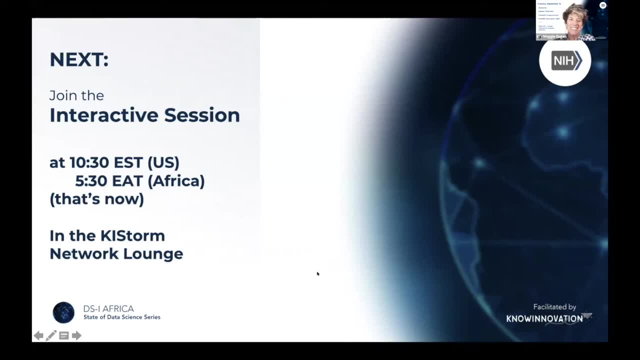 on when they are, who's going to be speaking and you can get more information and put them in your calendar. And, as we reminded you before, up next we have the interactive session. It's happening right now in the Kaistrom Network Lounge. We invite you and see you there and we